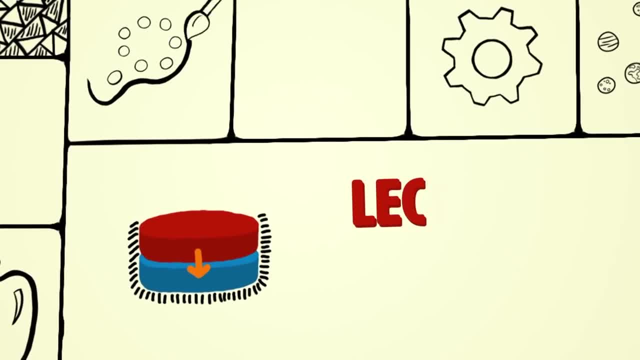 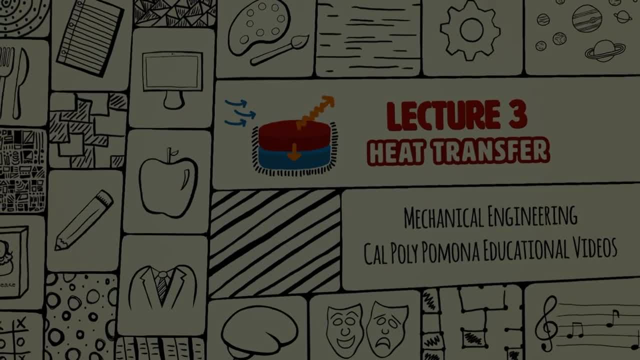 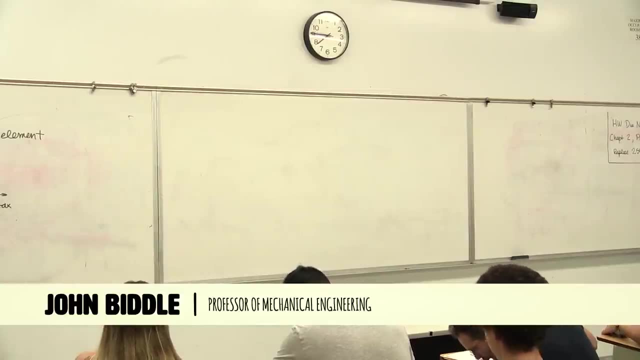 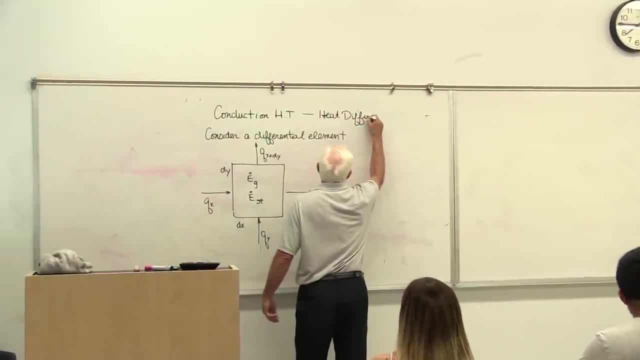 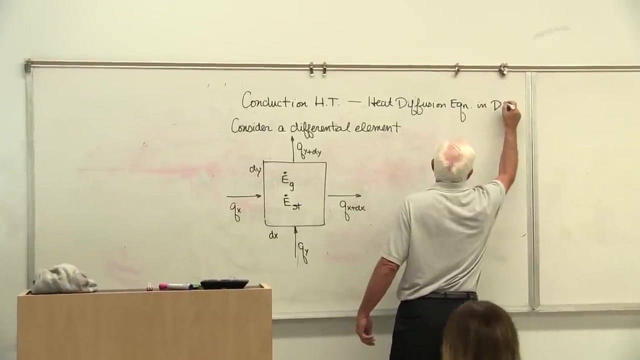 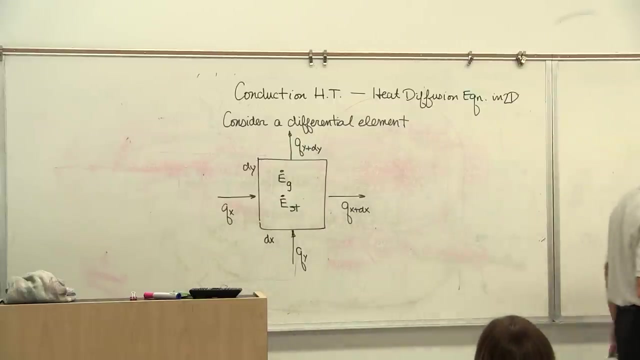 We're going to derive the governing partial differential equation, called the heat diffusion equation, In 2D. okay, we've done this little game before. in thermal and fluids We take a small element, a differential element. in this case we'll consider it to be a solid of a solid. 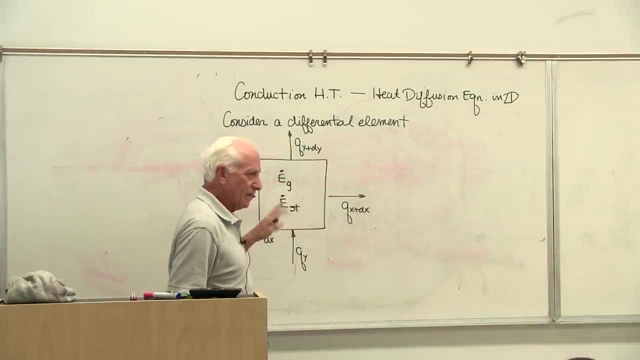 and we're going to look at all the energy terms coming in and going out of that. solid A differential element means it's dx. by dy It's going to be 2D. We're going to ignore the z right now. So here's our little control volume. 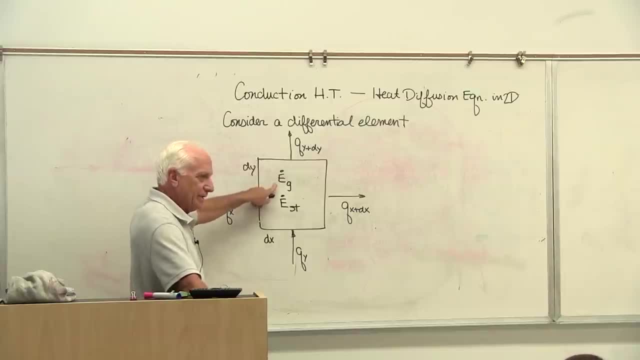 It's a differential element. E dot g is the energy generated internally. E dot storage is the change in stored energy. This is conduction. The energy coming in on the left-hand face comes in by conduction. We call it qx. We assume it varies continuously. 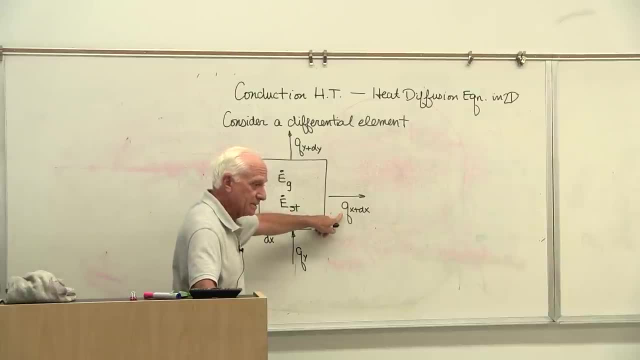 We write the energy going out as qx plus dx Energy coming in the bottom, the face down here, qy by conduction Energy going out the top by conduction: qy plus dy. Okay, so with that we can go ahead and start putting some terms in there. 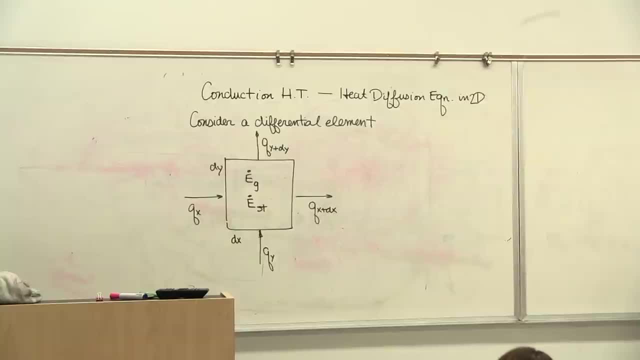 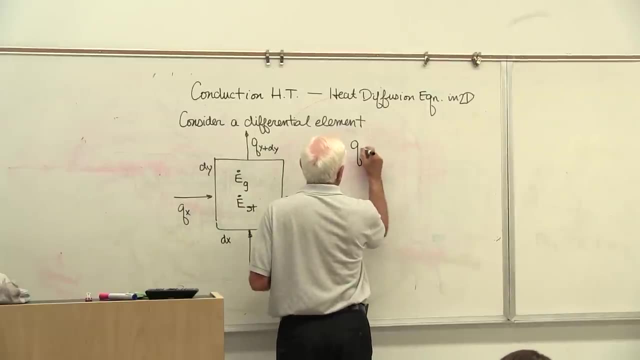 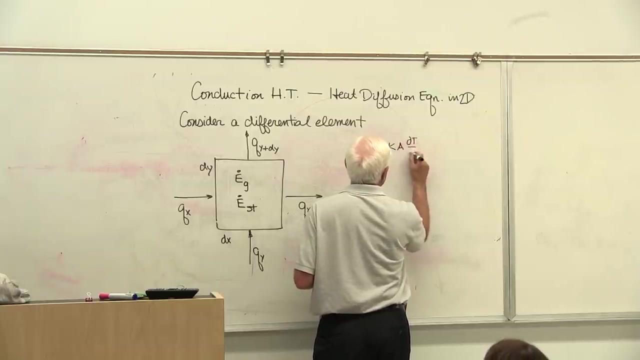 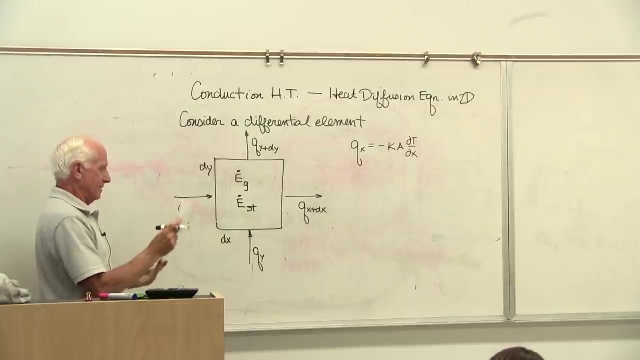 I think what I'll do. yeah, let's put in. let's put qx in here. qx is conduction, so it's minus k, a, dt, dx. The area through which the heat's conducted is this piece of paper. 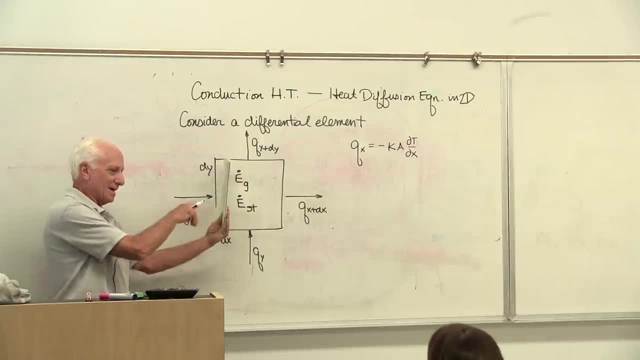 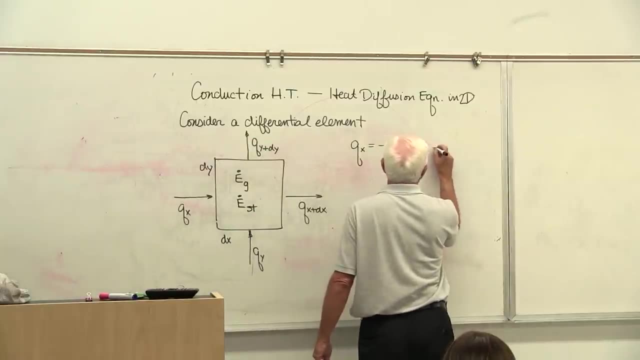 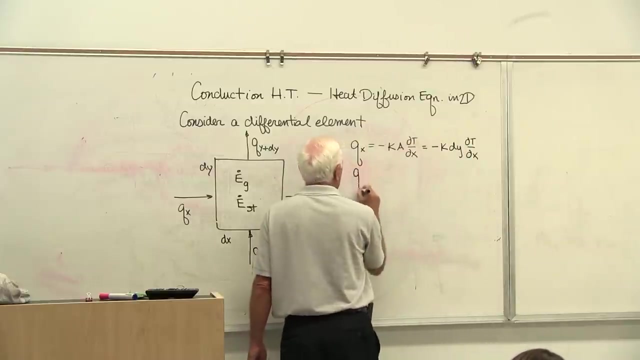 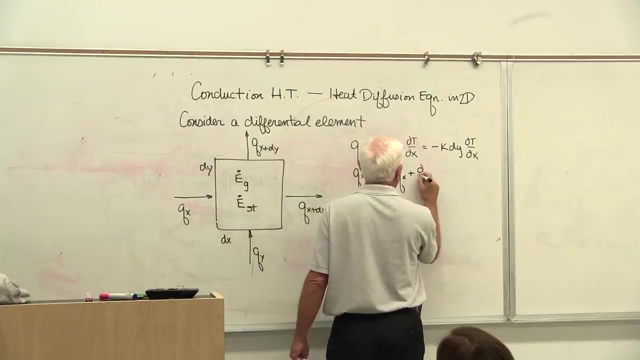 Its height is dy. Its length in the blackboard will say 1,, so dz is 1.. So it's 1 times dy. Okay, qx plus dx is equal to qx plus the partial, with respect to x, of qx times the distance you move in the x direction, which is dx. 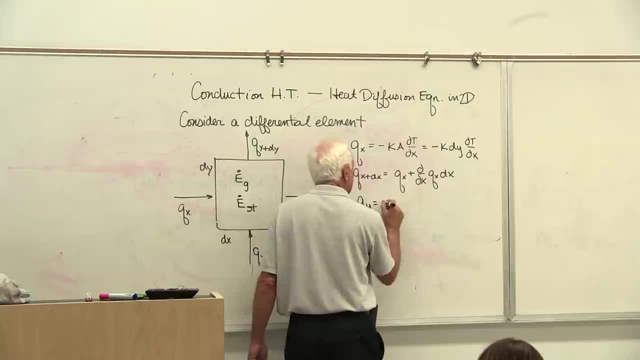 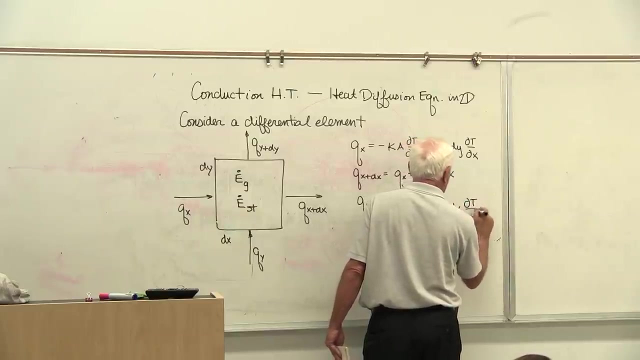 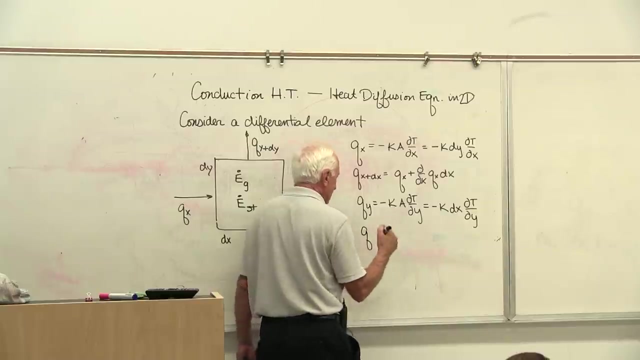 Similarly, conduction in the y direction: qy k, a, dt, dy. In this case the area is dx by 1. And expanding that in a Taylor series and neglecting higher order terms, qy plus dy is qy plus the partial with respect to y of qy times the distance you move in the y direction. 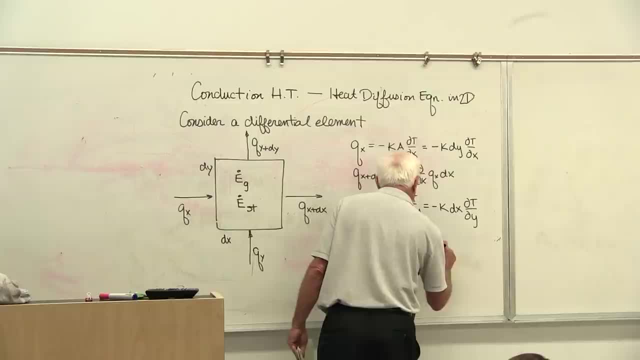 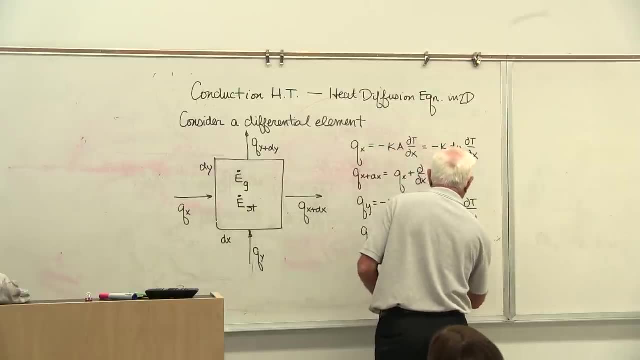 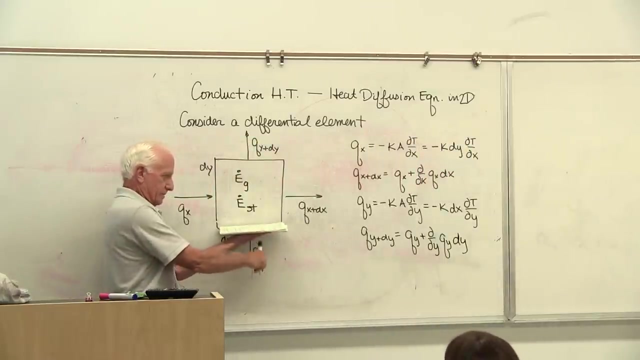 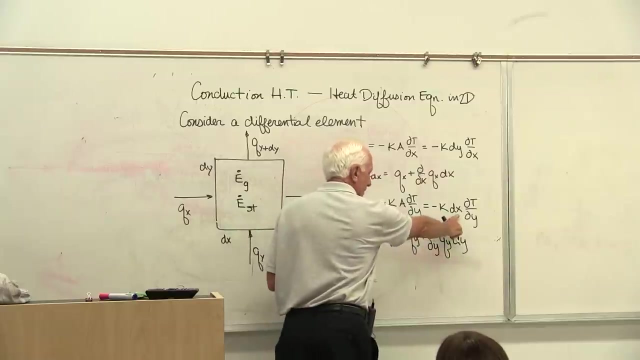 dy plus the partial with respect to y of qy times dy. Okay, The area for the bottom is the paper, So heat comes in the bottom. This length is dx, so the area is dx times 1. right there, Okay, Now let's start. 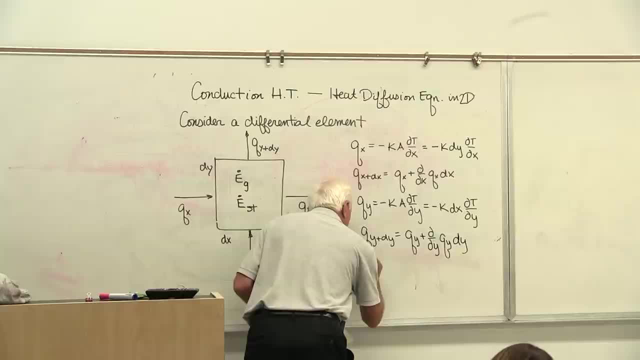 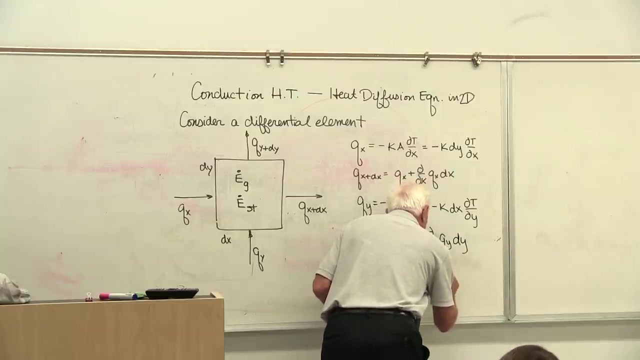 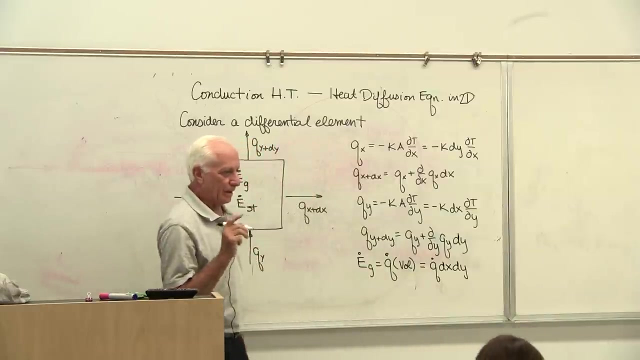 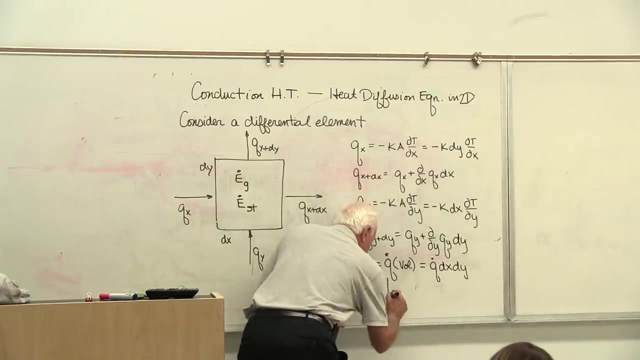 do the e dot gen. e dot gen. we bring a new term in, It's q dot times. the volume, Okay, And the volume of that little differential element is dx times, dy, times 1.. So now we have a new q term, It's q dot. That q dot is energy generation per unit volume, Per. 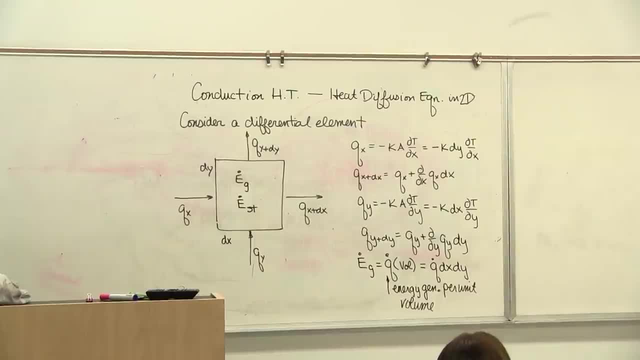 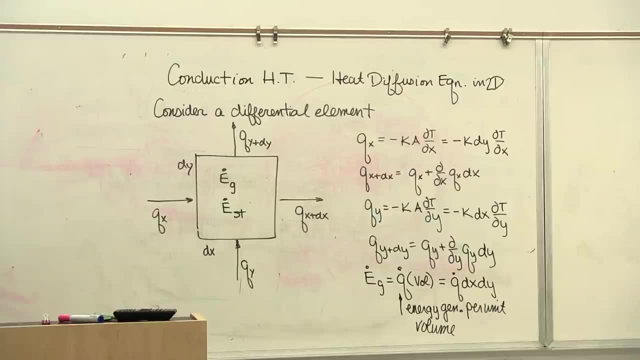 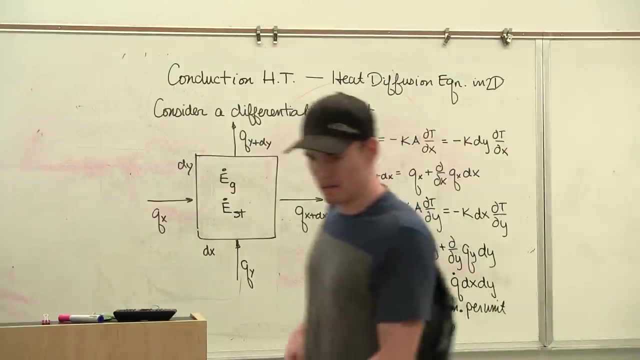 unit volume. So over here, here's our q's now: q all by q dot. q all by q dot. q all by q dot. q all by itself, q prime, q, double prime, q dot. They're all different, but they're all q's. 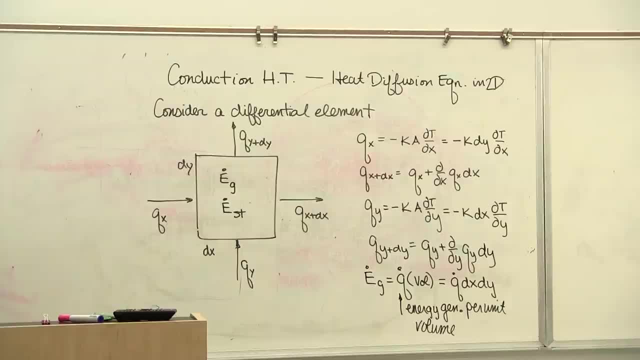 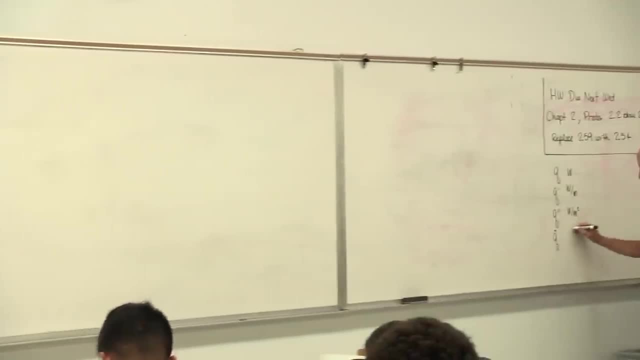 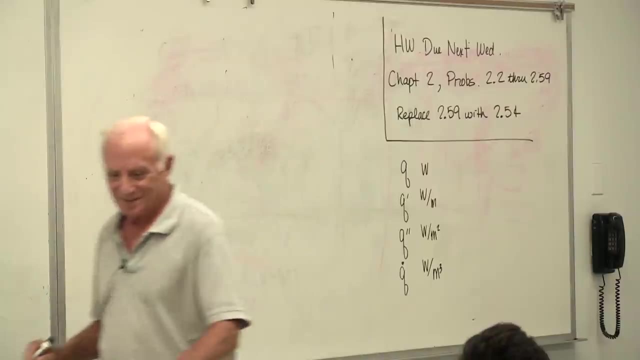 The first one watts, The second one watts per meter, The third one watts per square meter Heat flux. And now we got the fourth one, Watts per cubic meter. Okay, So four different possible q's. Know what each one means. 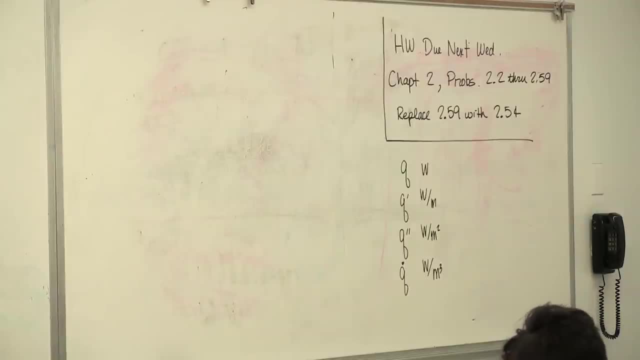 If a problem asks you on homework or exam for the heat flux, you know what they're asking for. If they ask you for the heat rate rate, you know what they're asking for. q dot: you know what they mean. Volumetric energy generation. 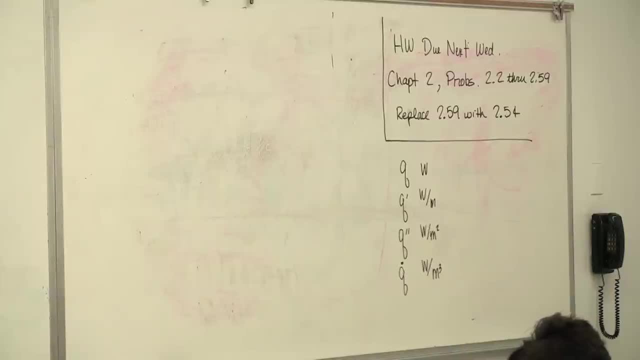 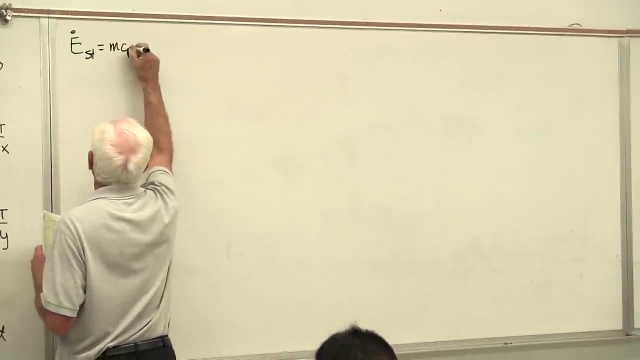 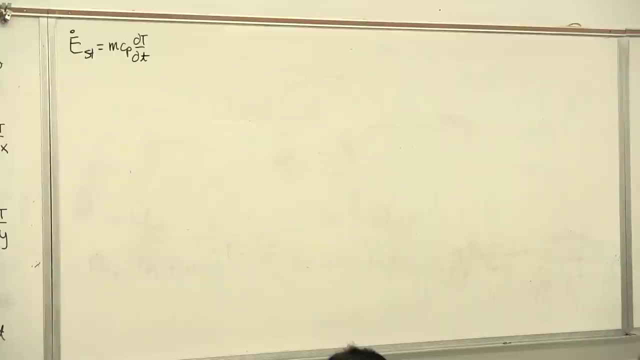 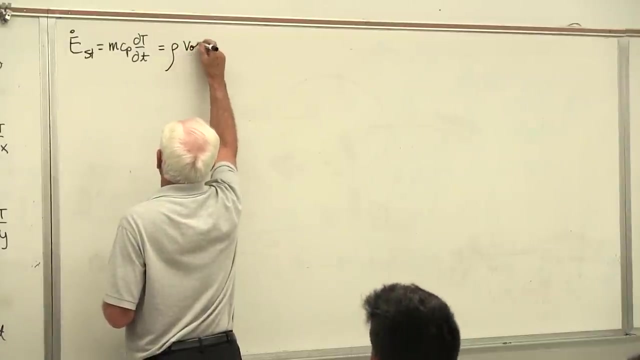 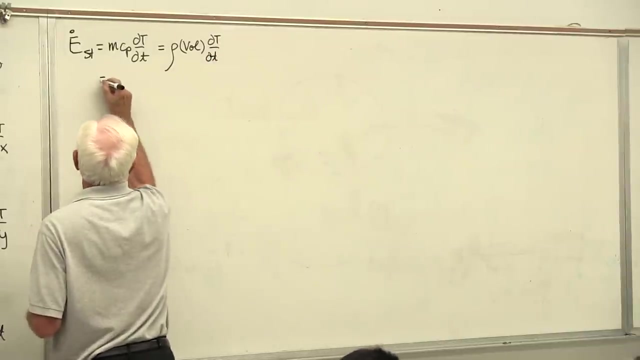 And the last one is the storage. I'll put that up here: q dot storage mass, cp, dt d time. The mass of that differential element is rho times the volume dt d time. So this is equal to the volume dx by dy times 1.. 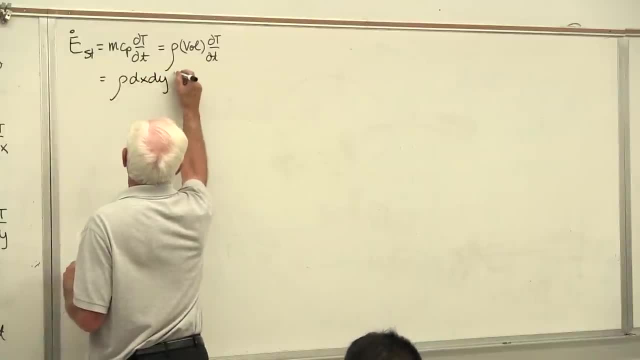 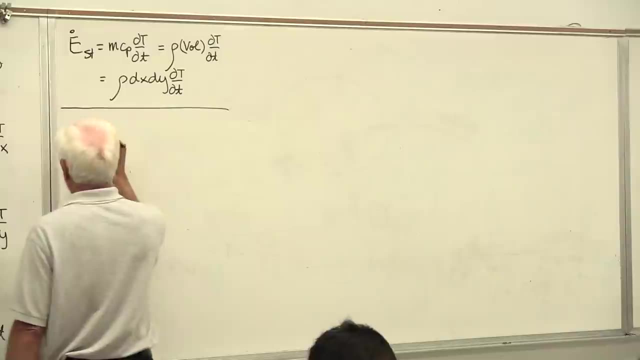 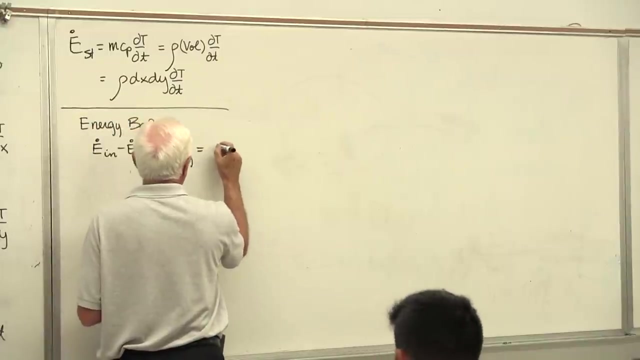 So rho dx dy partial t with respect to time. Okay, now we put those in the energy balance equation. Okay, energy balance equation: it says what comes in minus what goes out plus the generation equals the change in the stored energy. 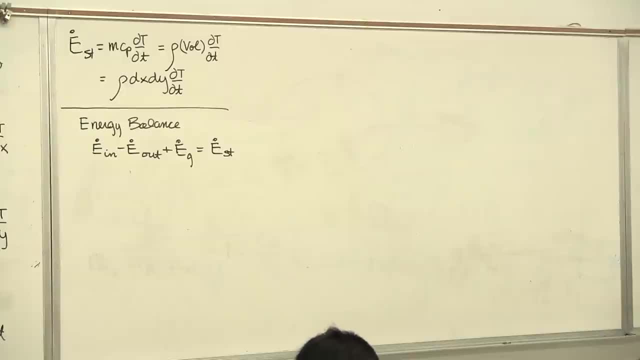 Now look at the picture. What comes in by conduction qx plus qy? What does out? Okay, look at the picture, or this equation: right here, It finally것��. Then we have QY going out, And then we have plus Egen down here. 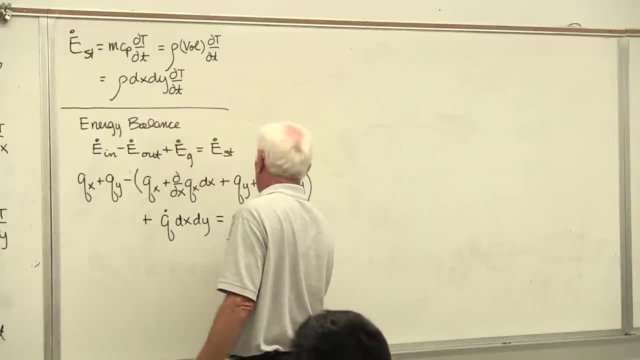 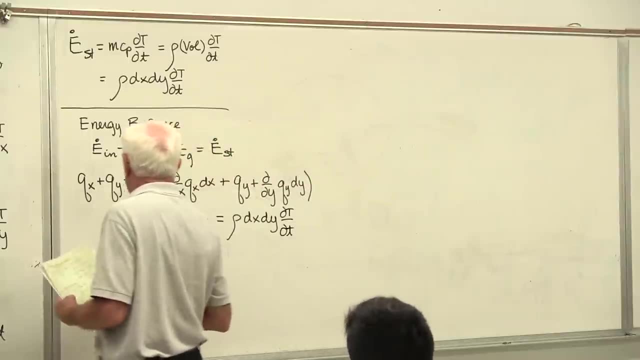 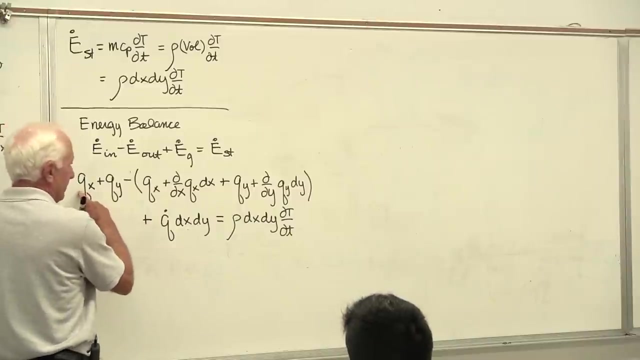 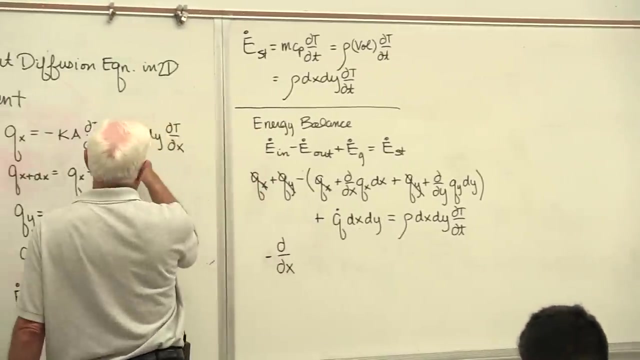 And then we have that equals Q dot storage up here. Q dot X minus Q dot X cancels out. Q dot Y minus Q dot Y cancels out. We're left with partial with respect to X. X of QX. there it is okay. there's a minus sign in front of there. 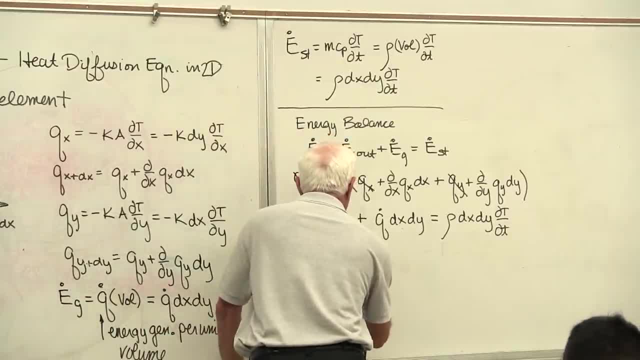 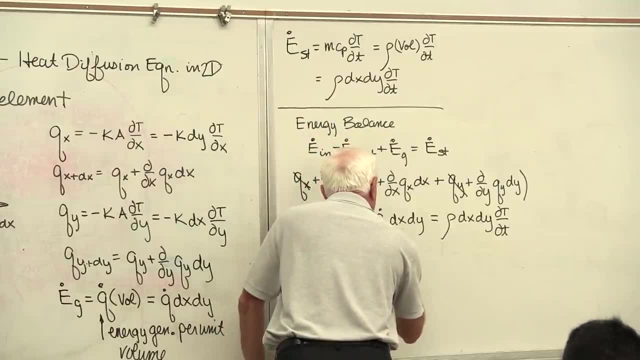 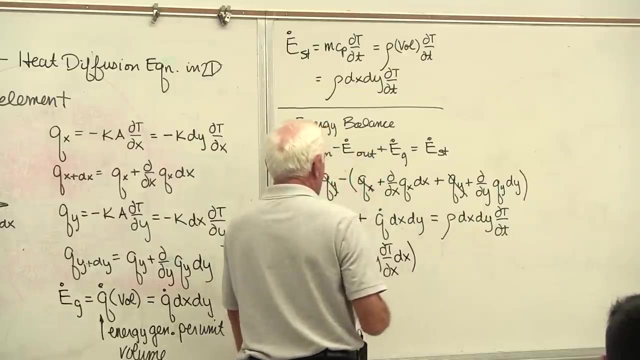 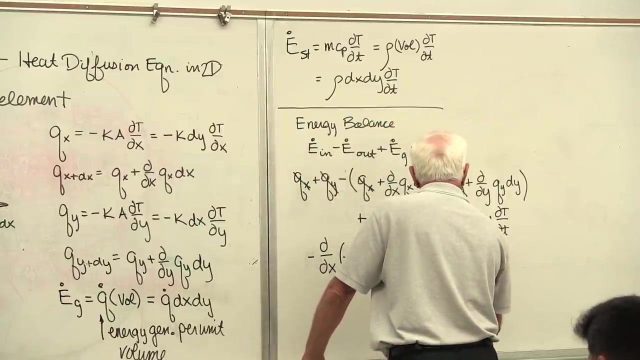 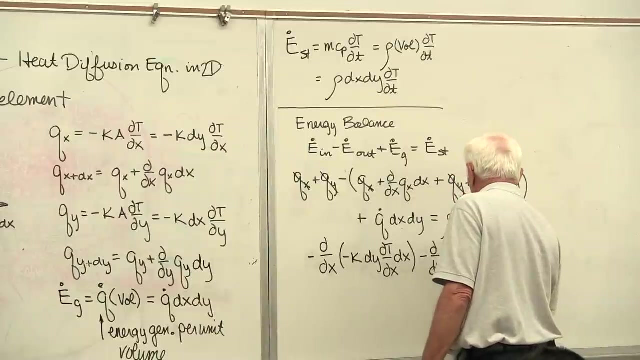 Minus K, DY And we have DY partial T with respect to X times our DX. And then for the second term, the Y term, It's minus partial with respect to Y of QY. there it is minus K, DX partial T with. 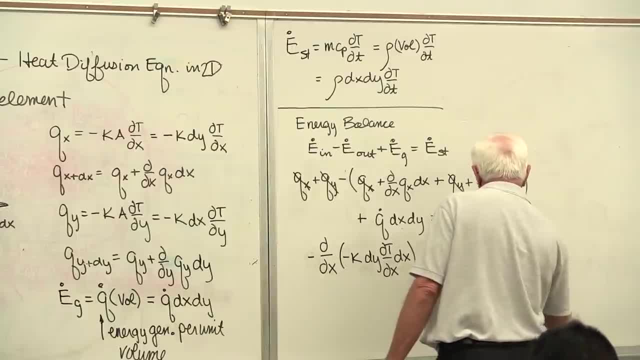 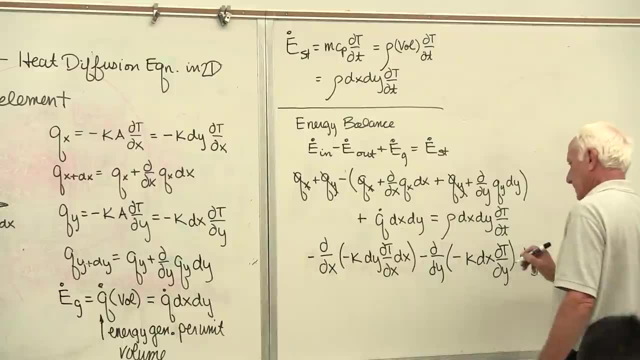 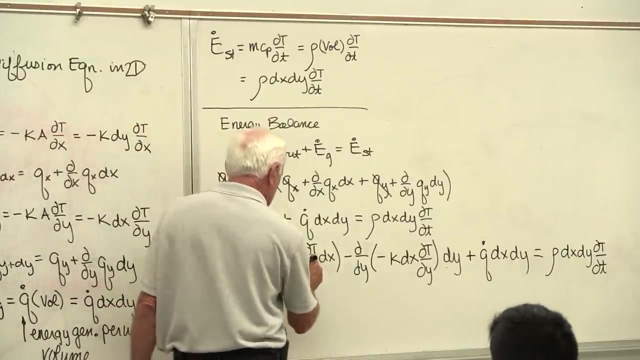 respect to Y multiplied by DY, okay, And that we have our E dot gen, which, right here, Okay, E dot gen plus Q dot DX DY, equal E dot storage. right there, And lucky for us, we see each term has a DX DY in it. 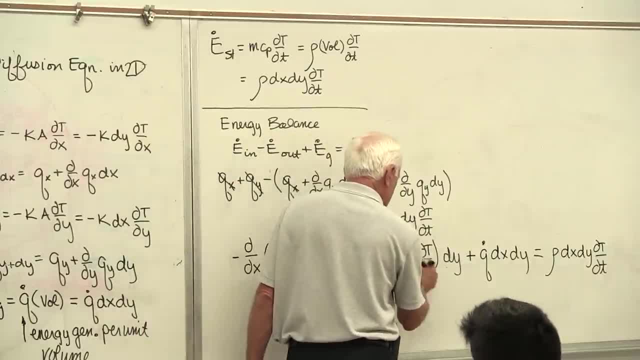 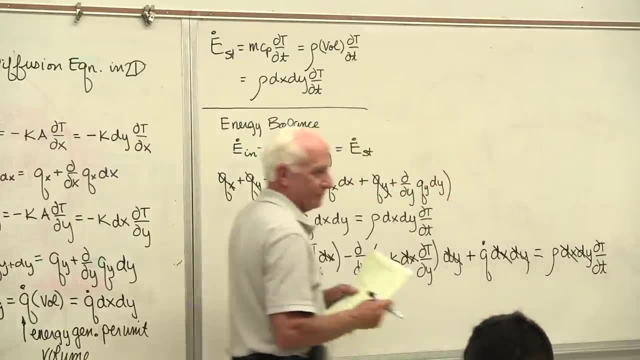 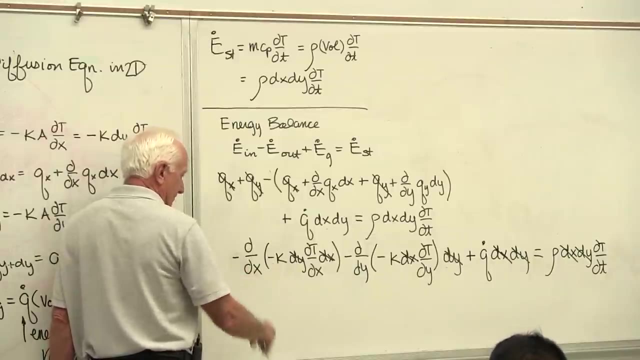 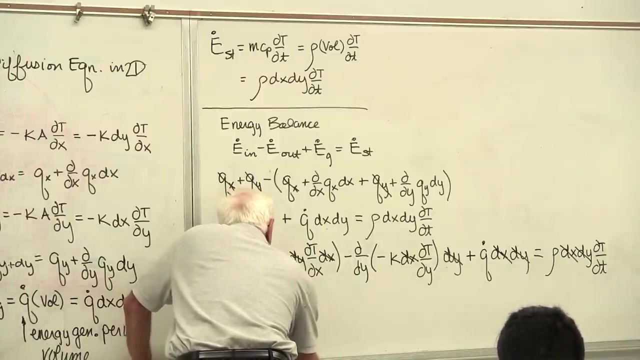 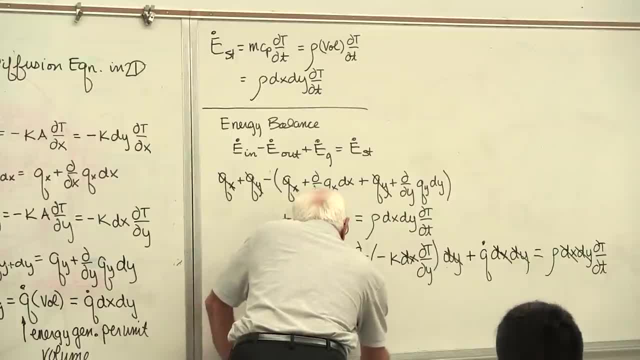 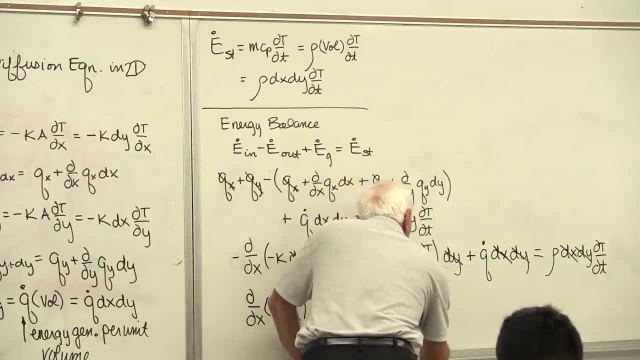 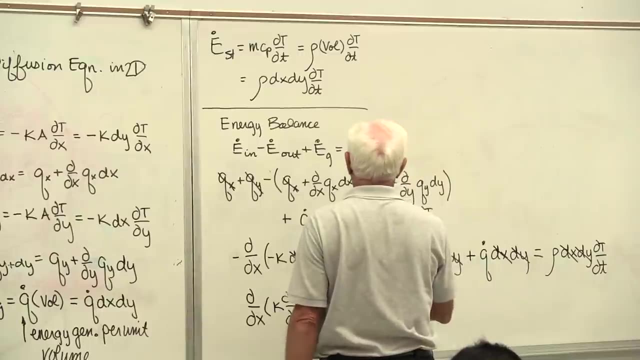 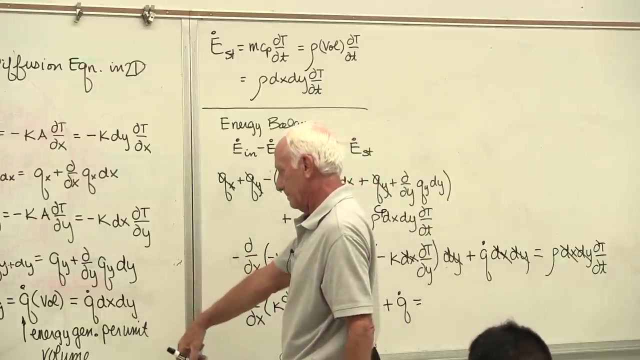 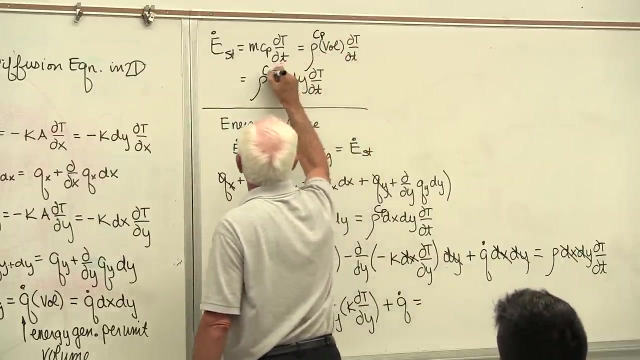 Plus partial with respect to Y, K, DT, DY, Okay, plus Q, dot is equal to: there should be a pop up up up, up up. row CP here for storage. I had it over here. oh, here, yeah, there should be a real part me row CP up here. row CP- okay, row. 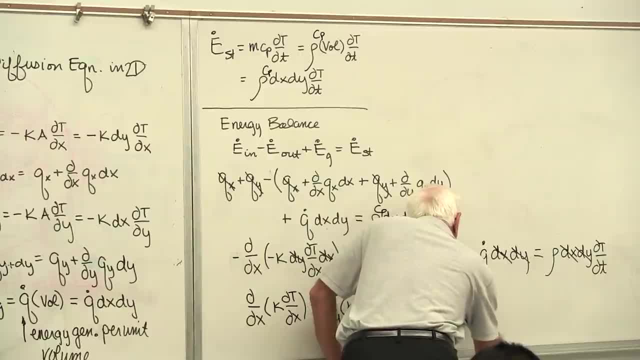 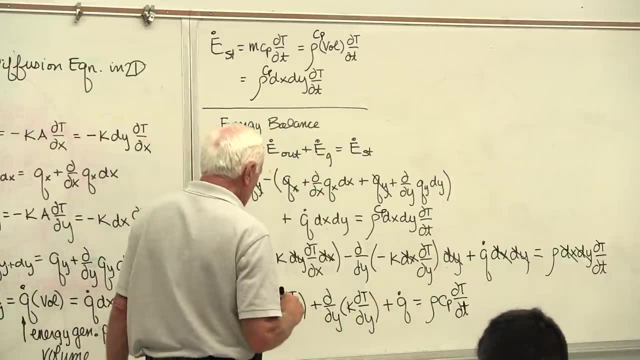 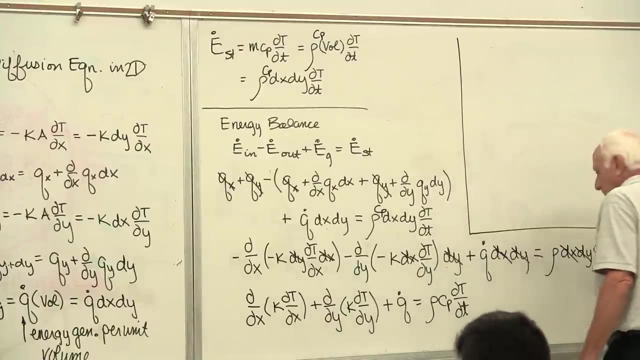 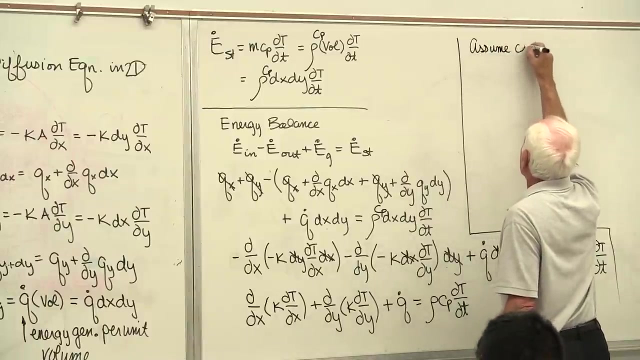 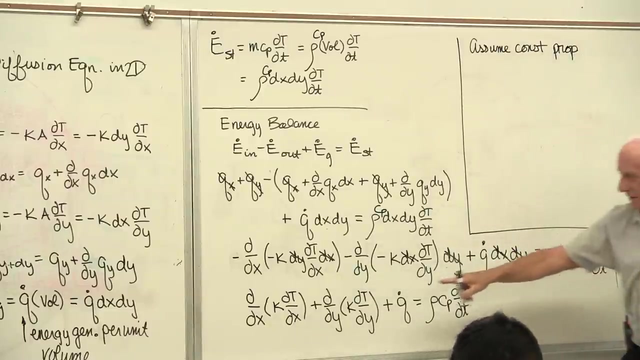 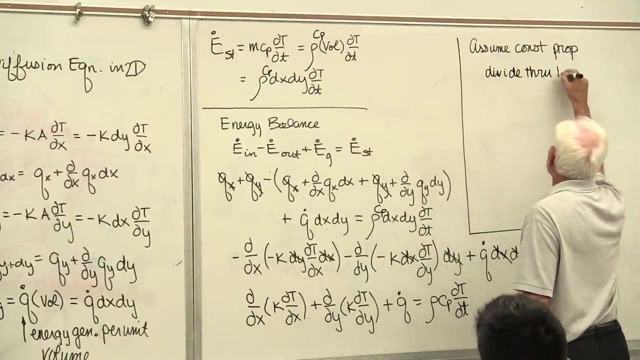 CP partial T with respect to time. we're gonna make an assumption here, make life a little easier right now. we're going to assume the properties are constant. assume constant properties. the K value then comes outside the partial sign. K comes outside the partial sign to button and divide through by K. okay, so we have second partial T with respect to X. 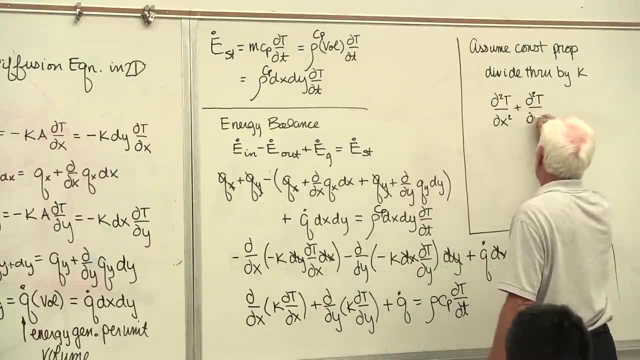 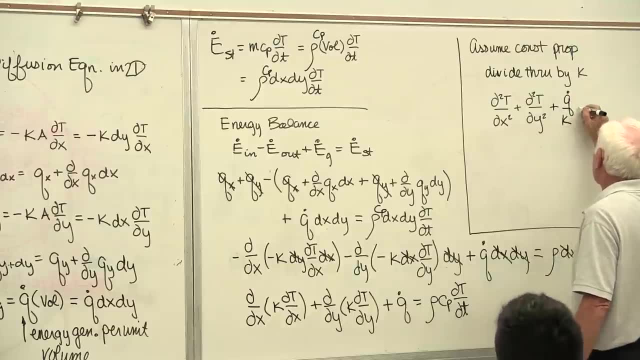 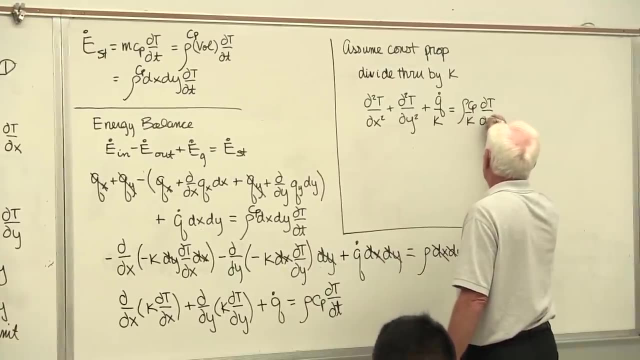 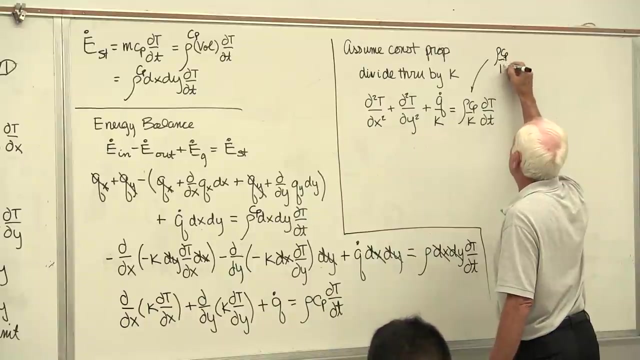 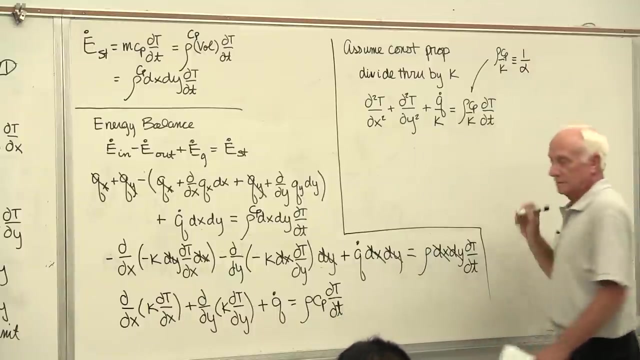 second, partial T with respect to Y plus Q dot over K is equal to row CP over K. partial T with respect to time. but row CP over K is just what we define back in early chapter two as alpha, the thermal diffusivity. so the right hand side can be written as one over alpha partial T. 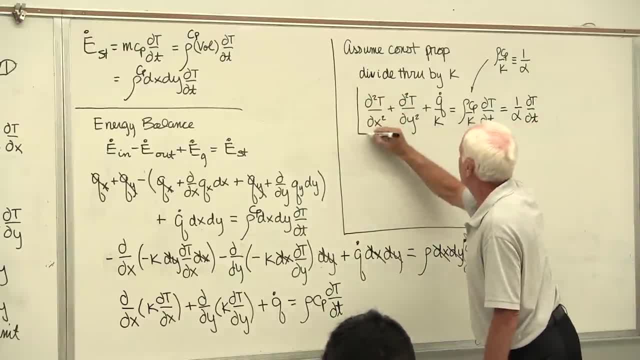 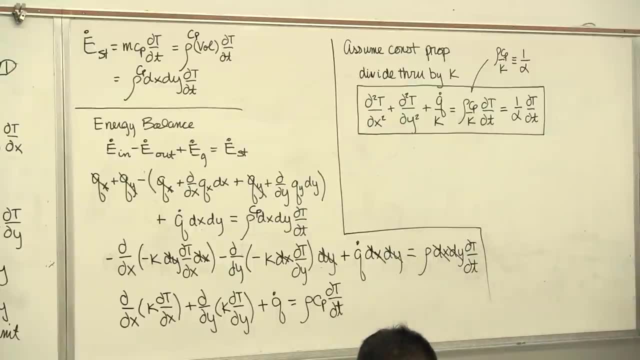 with respect to time, this boxed equation is called the heat diffusion equation in two dimensions, the heat diffusion equation in two dimensions. if it's three dimensions. all we do on the left hand side is add the second partial of T with respect to Y over K and we get the second partial of T with respect to Y over K. 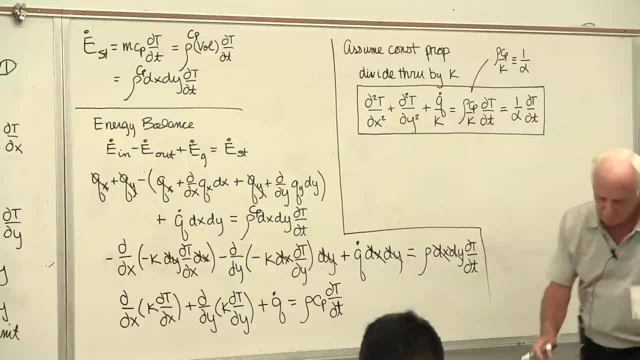 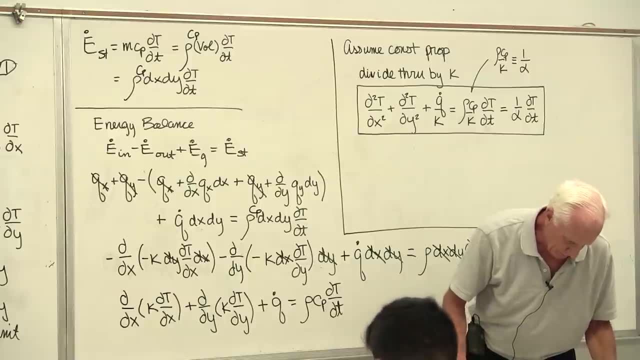 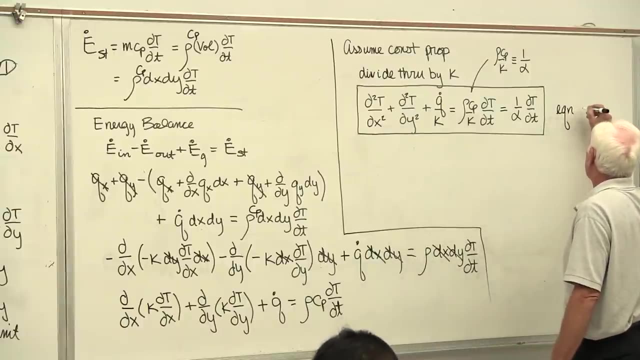 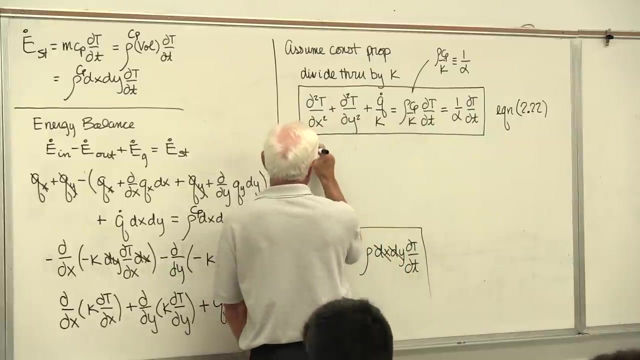 and we get the second partial of T with respect to Z and that equation is in the textbook 222. yeah, 222, equation 222. if you want it in cylindrical, correct me if I'm wrong. correct me if I'm wrong. correct me if I'm wrong. 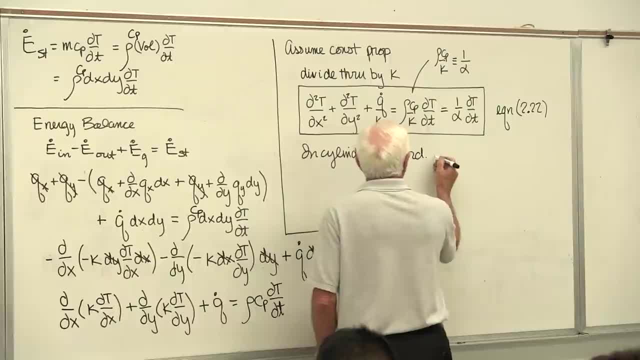 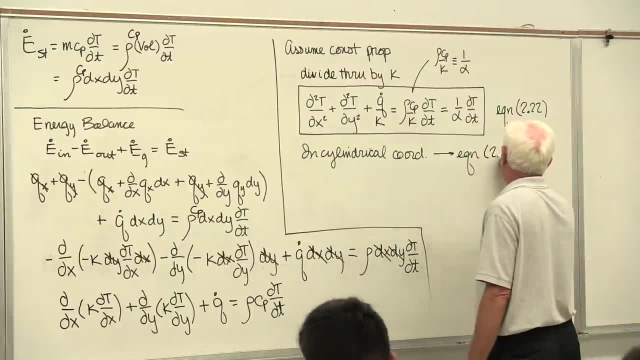 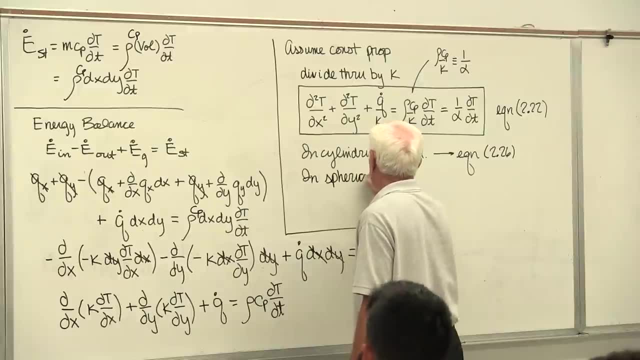 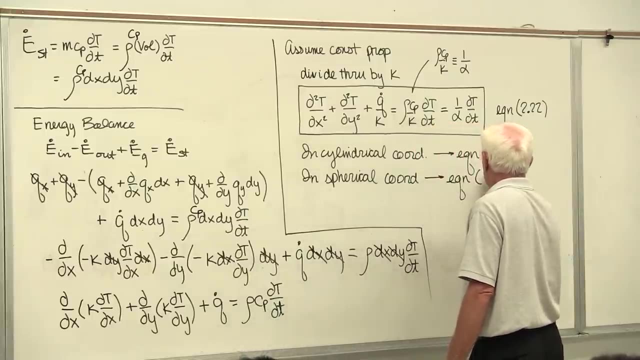 we're not going to derive it. the we're not going to derive it. the equation in the textbook is 226. if it's equation in the textbook is 226. if it's equation in the textbook is 226. if it's in spherical coordinates: equation 229. 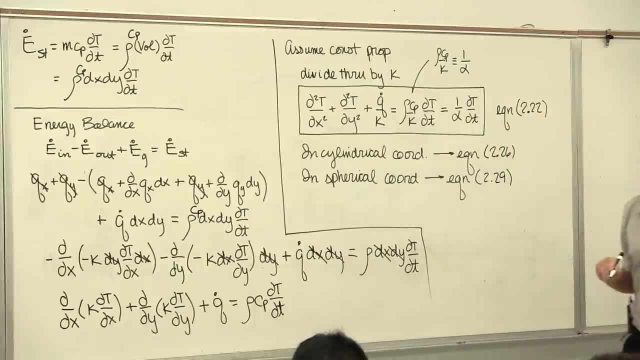 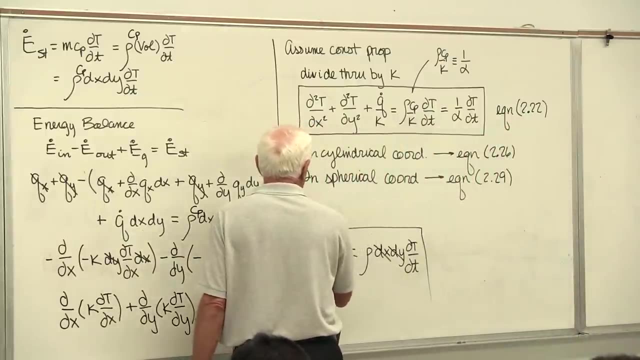 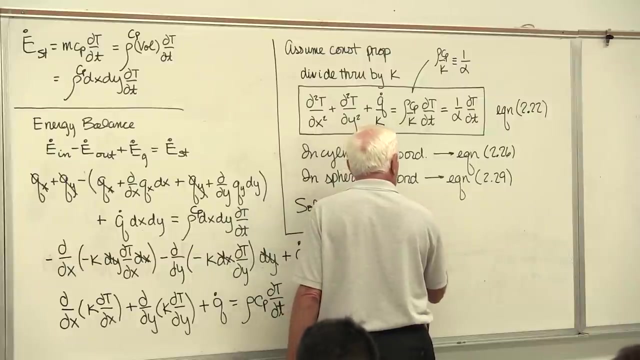 in spherical coordinates, equation 229. OK, So there's the governing partial differential equation. What's the purpose of that guy? The purpose is to solve it where you get the temperature as a function of the variables. So you solve to get temperature as a function of the variable x, the variable y and time. 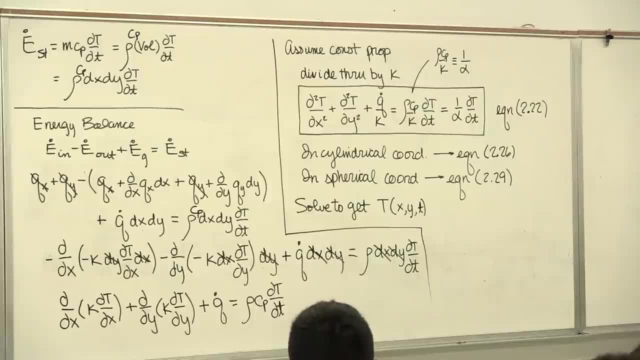 In Chapter 3, we'll solve a very, very simple version of that with a lot of assumptions, But for right now that's the general form. What are the assumptions in the boxed equation? OK, There, it is right. there, There it is. But you can't solve a PDE or any DE unless 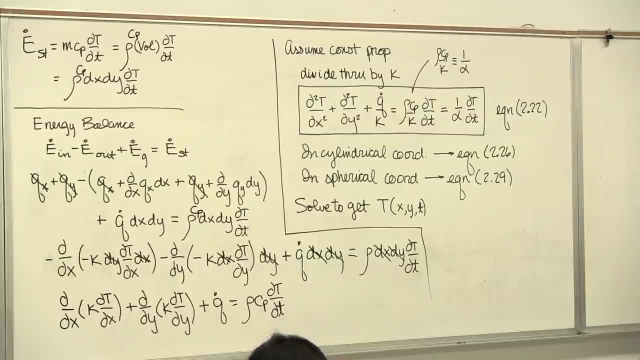 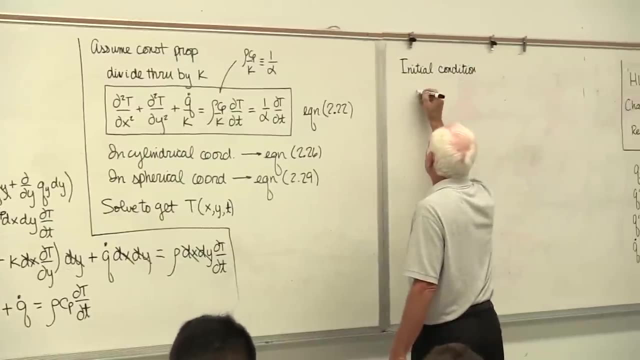 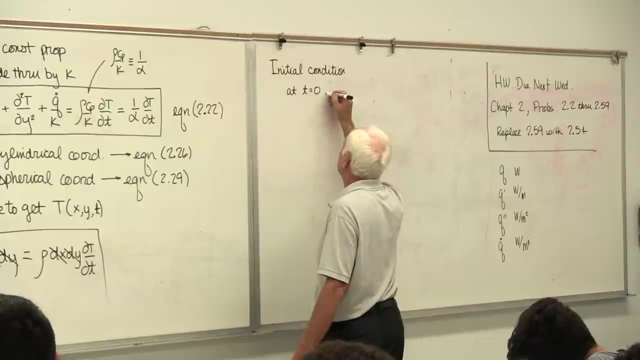 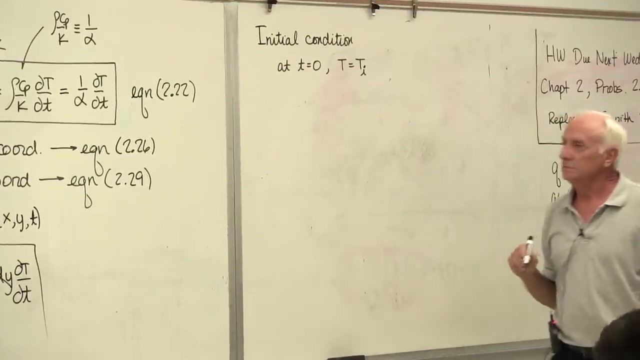 you give somebody boundary and initial conditions, So we need boundary and initial conditions to solve this. So we'll do the initial condition first. At t, the simplest one is: the initial temperature At t equals 0, the temperature equals ti, where the i of course stands for initial. For instance, if I had a 3 inch by 3 inch, 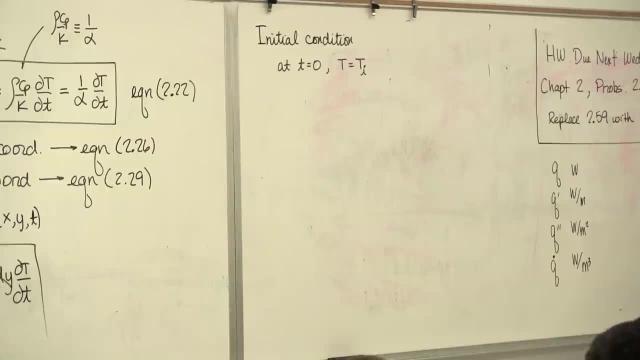 cube of copper And I heat it up to 100 degrees Fahrenheit And then I blow colder air over it at 50 degrees Fahrenheit. To solve that equation in three dimensions, then what I would need is initial conditions. So my initial condition, called ic, is when time equals 0, the temperature anywhere in 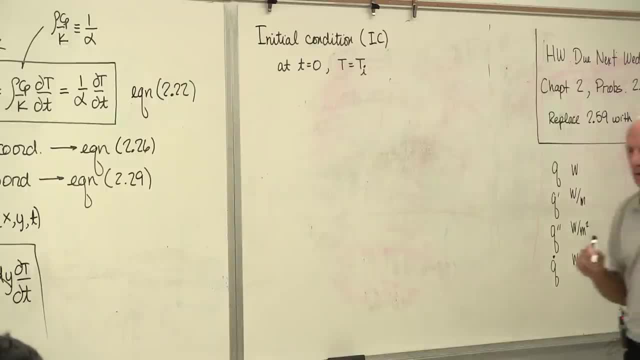 the cube is 100 degrees Fahrenheit. OK, That's it. Now I need a boundary condition. OK, We're going to make it easy for ourselves now. Let's say it's 1 dimensional. OK, 1 dimensional. So all we need is 1 condition on that. 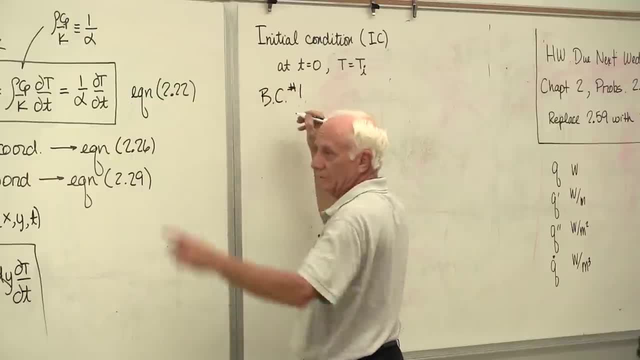 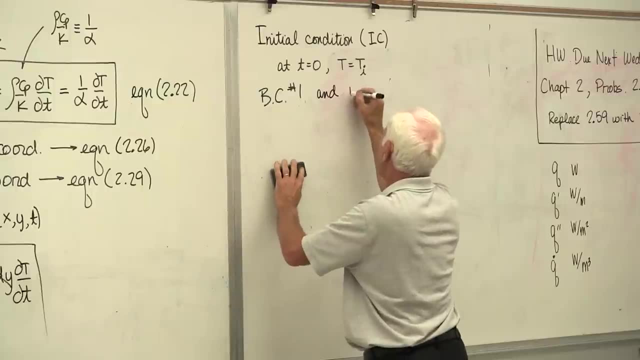 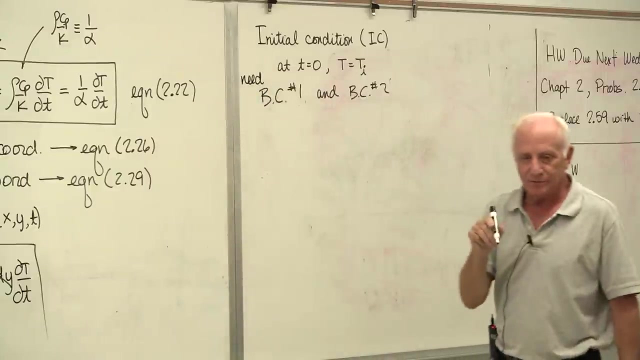 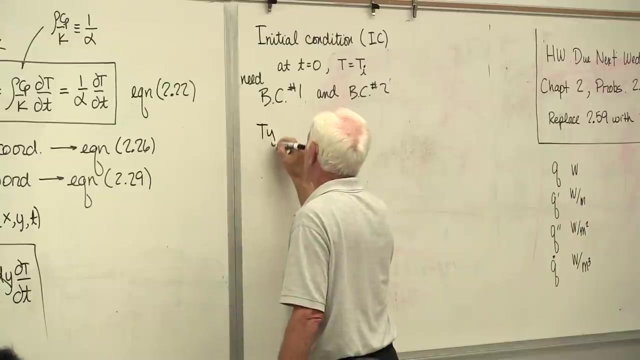 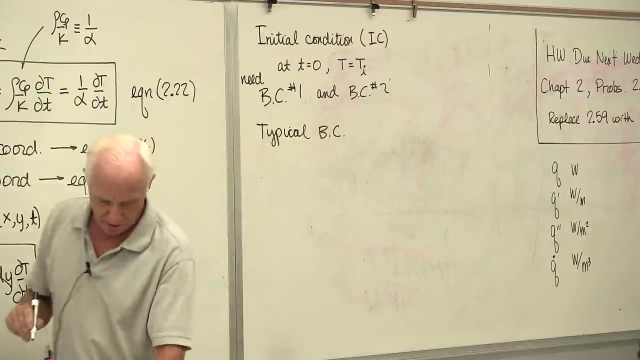 So boundary condition? there will be two of them: number 1 only with x, Boundary condition 1 and boundary condition 2.. We need these. Somebody has to tell you what are the boundary conditions. Okay, let's put some down here. Typical boundary conditions: Okay, these are on table 22.. Yeah, table 22.. 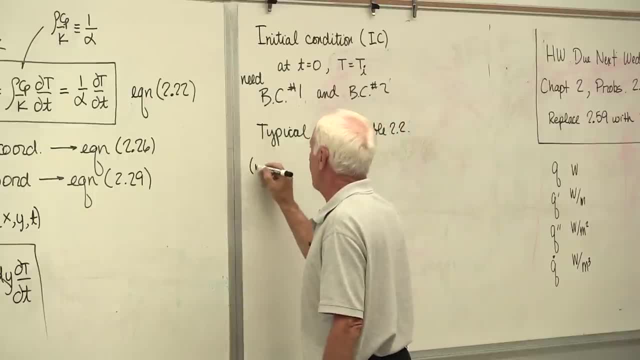 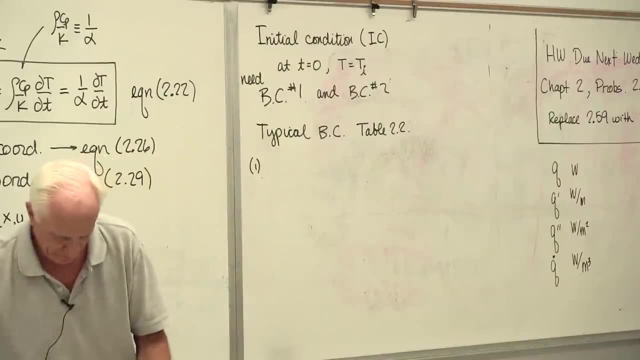 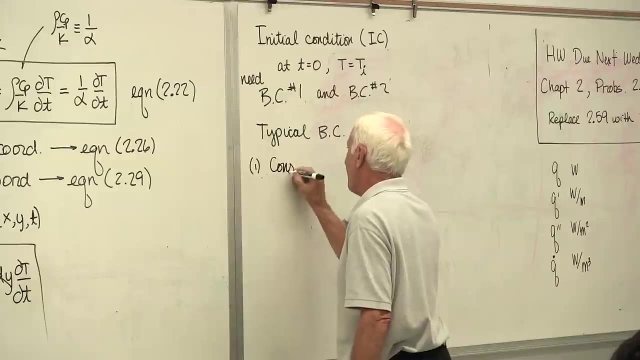 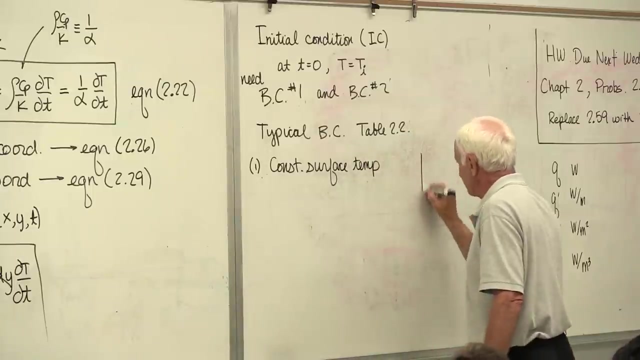 Okay, type 1.. Type 1 says constant surface temperature. These aren't all of them, These are just typical ones, the ones we use the most. Constant surface temperature. So if we have a surface- and here's the material, thermal conductivity K. 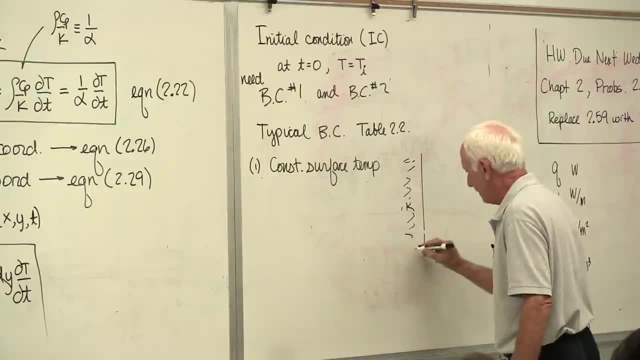 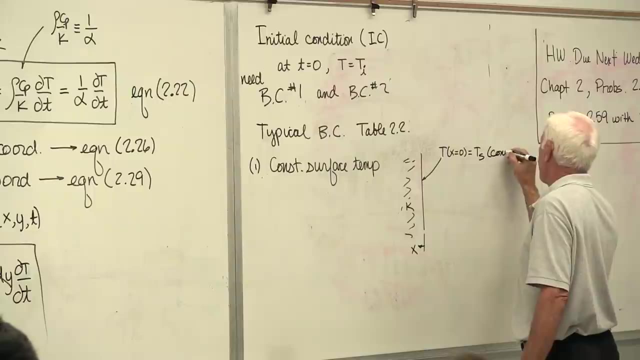 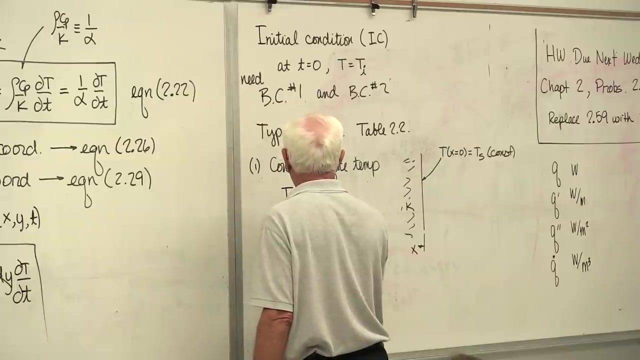 we're measuring x from the surface into the material and somebody says: oh, by the way, I'm going to keep this temperature at the surface at x equals 0, equal constant surface temperature. Then temperature at x equals 0 for any time. T for any time. 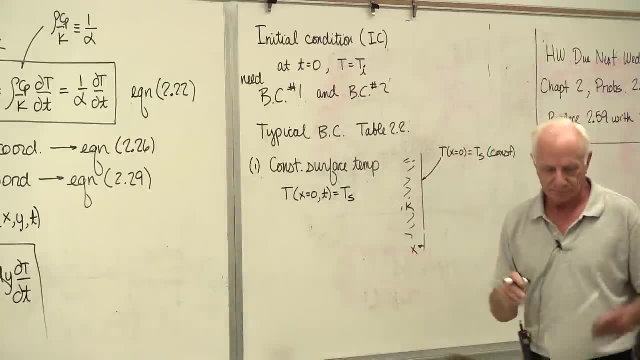 is going to be a constant value of Ts. Okay, You could probably treat that wall right here as a constant temperature wall. I guarantee you the outside wall is hotter than the inside wall right here. So if I'm going to analyze this wall by conduction here the wall outside, especially in the afternoon when the sun hits that wall, 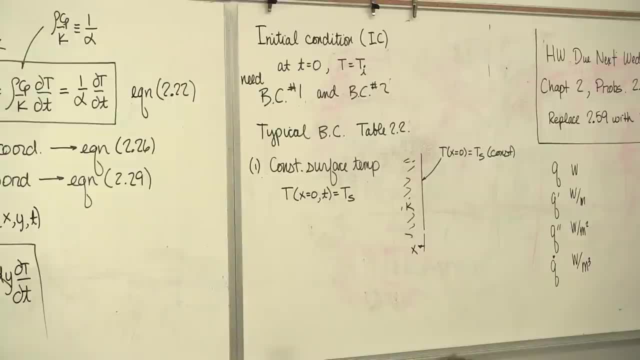 the outside temperature is warmer than the inside wall, And what's my boundary condition? Well, it could be convection, but I would probably assume- maybe to start with that- that temperature is going to be constant. I don't think it's going to vary with time for the next half hour. 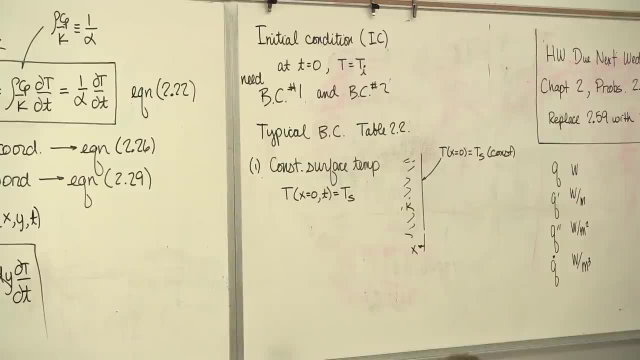 I don't think it's going to vary with x and y very much. from the middle of the wall to where my hand is, I think the temperature is pretty constant there, so I might model that as a constant temperature boundary condition. Number two: constant surface heat flux. 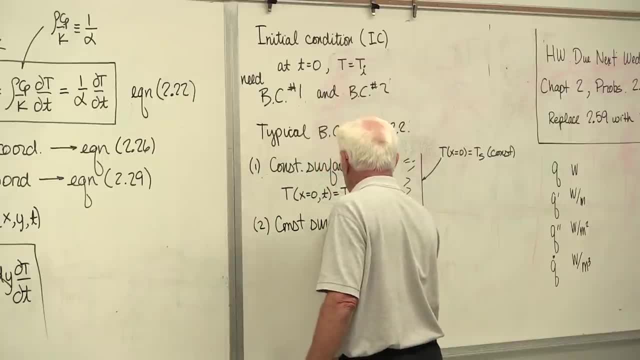 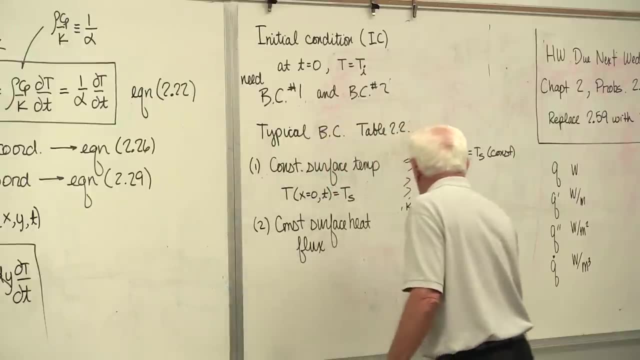 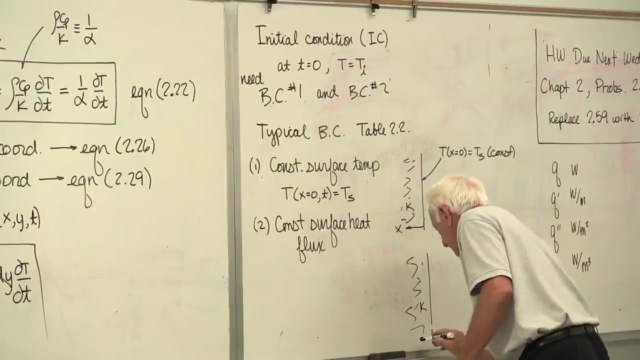 Okay, for this boundary condition, here's the wall again. thermal conductivity K. I'm going to measure x into the wall. x equals 0 is the surface, and for this one I have a constant value of T. I'm going to measure x into the wall. x equals 0 is the surface, and for this one I have a constant value of T. 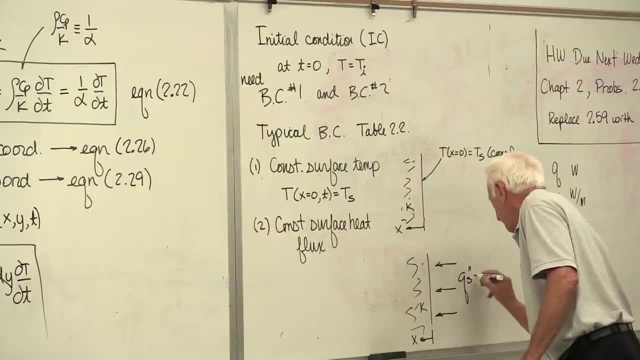 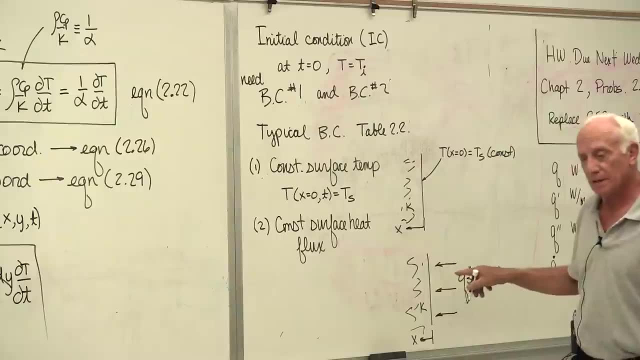 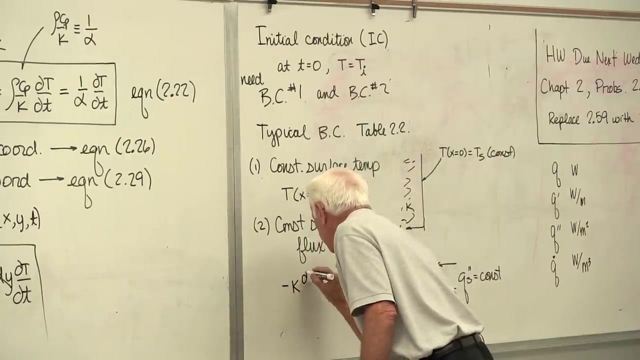 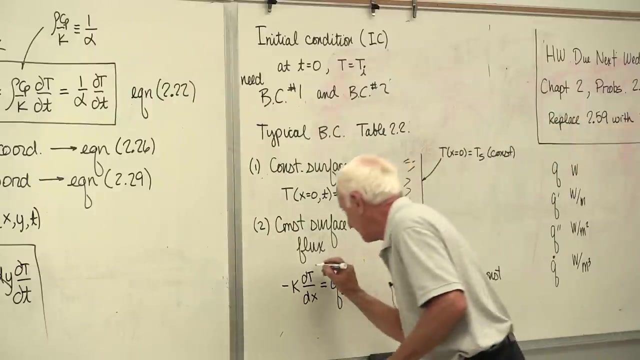 I'm going to measure x into the wall. x equals 0, is the surface, and for this one I have a constant value of T equal. that's the heat flux, QS, double prime, And this DTDX has to be at, of course, the 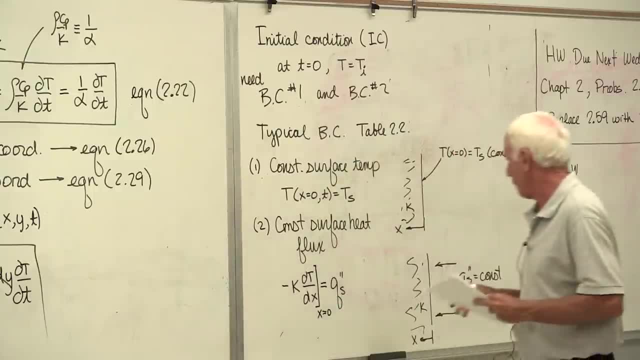 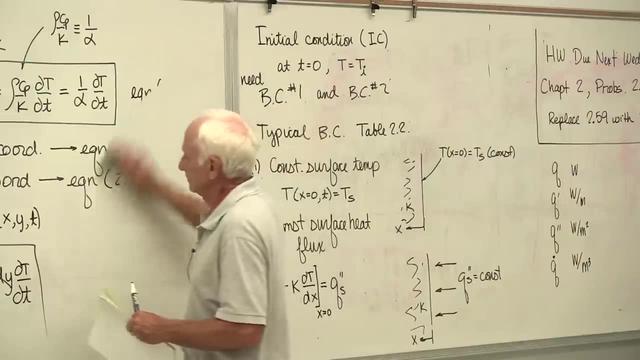 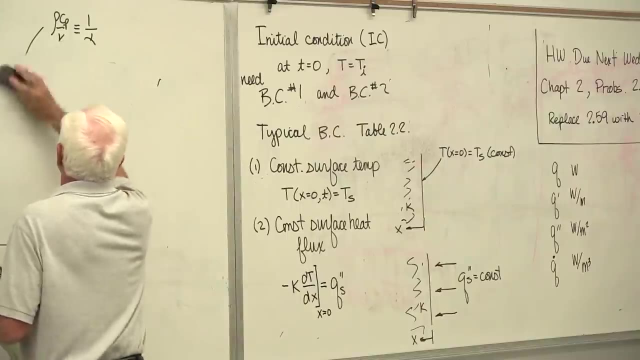 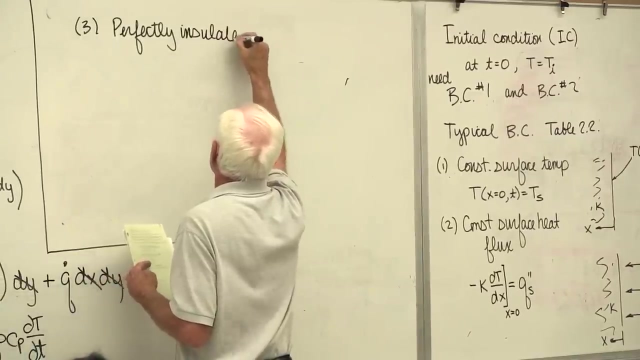 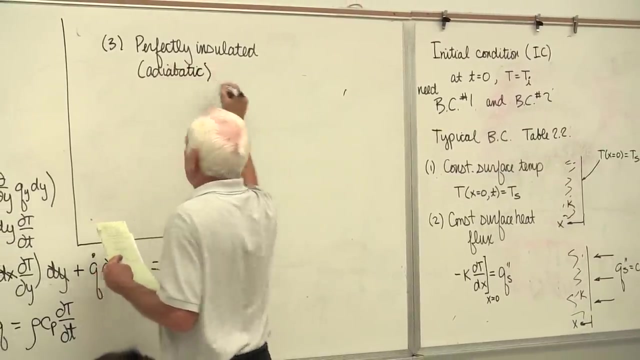 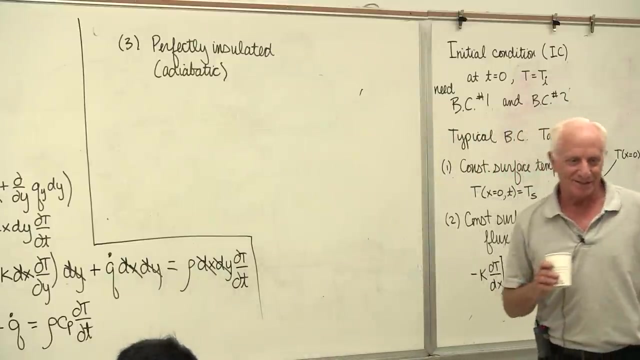 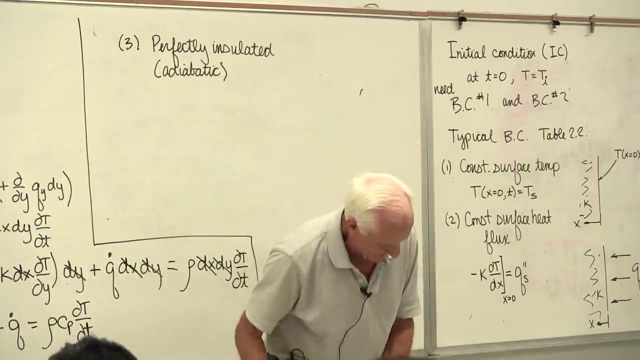 surface X equal zero Constant wall heat flux. Number three: perfectly insulated Adiabatic. The proper word is adiabatic. Adiabatic means the heat flux is zero. When someone says insulated, you always don't know if it's adiabatic or not. Okay, Homer, get over here. 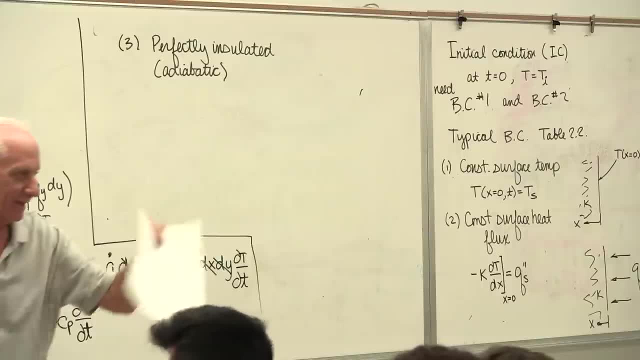 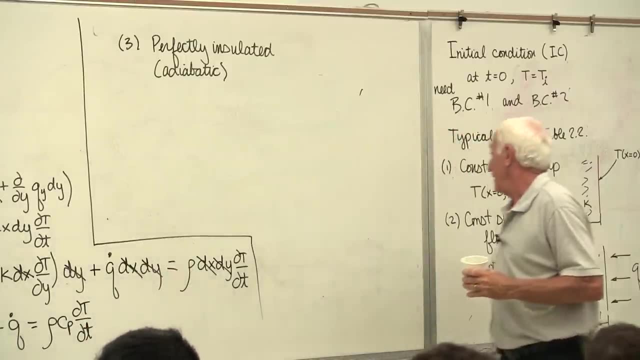 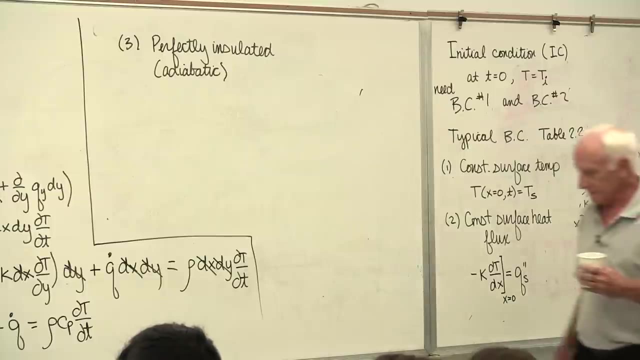 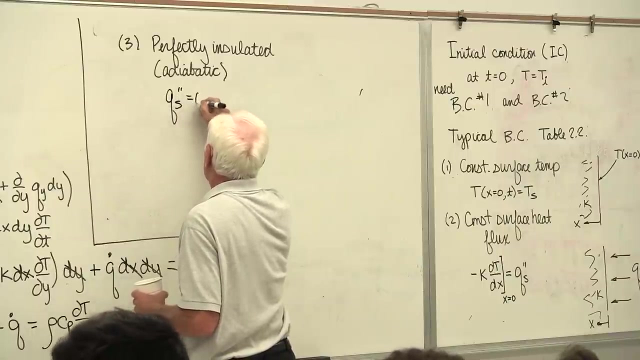 already, Homer, go to the banks. Okay, If you came in later, here's today's homework up here. Okay, Adiabatic, This guy is zero. No heat comes in or goes out. Zero. QS double prime equals zero, Which means that minus K, 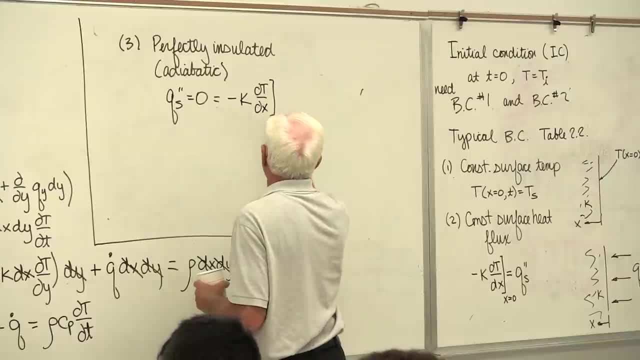 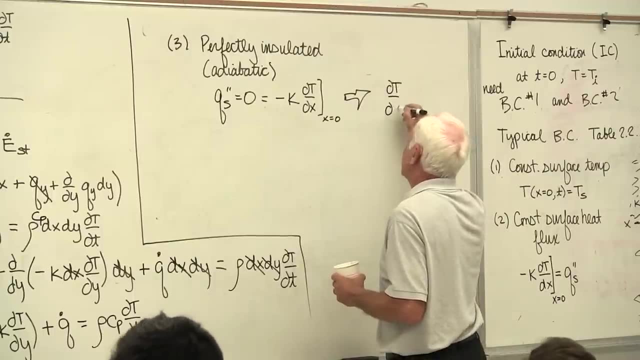 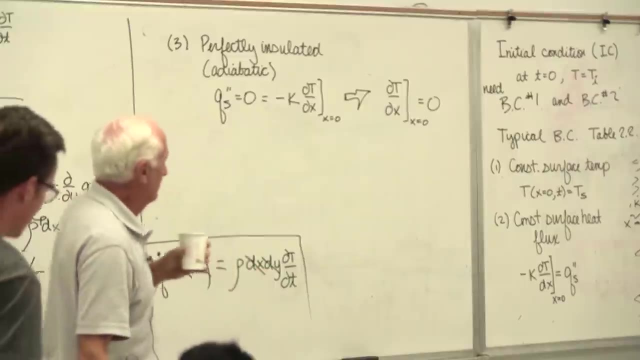 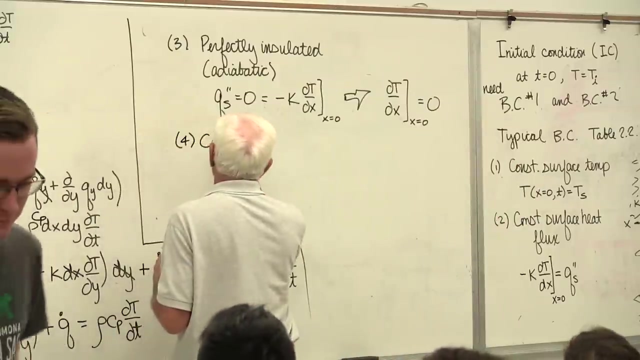 DTDX has to be zero, Okay, Which implies that partial of T with respect to X, at X equals zero, must be zero, Okay, That's the one you want. Partial T with respect to X- zero Four. Convection at the boundary. 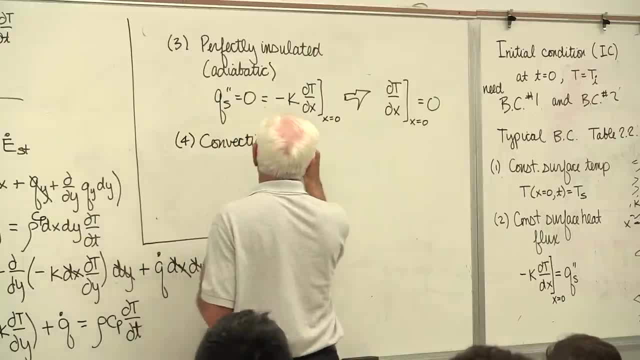 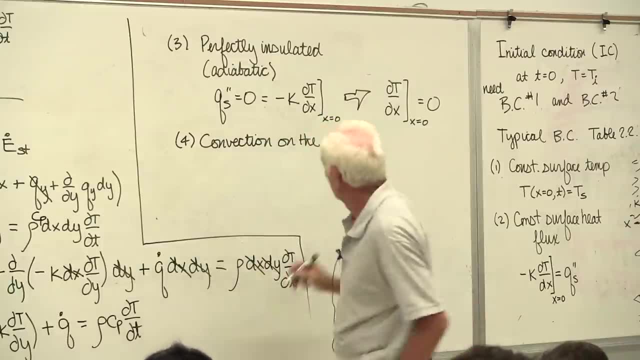 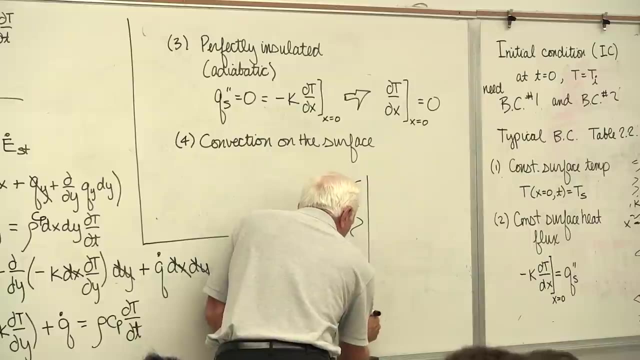 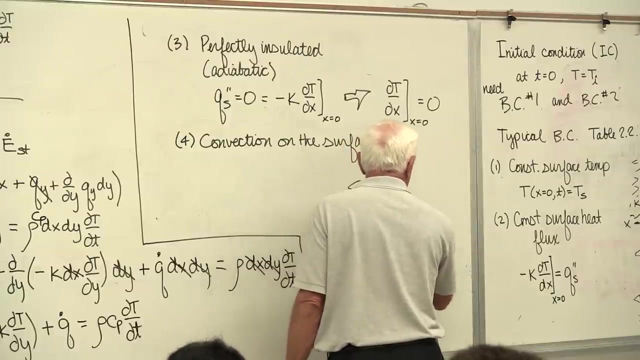 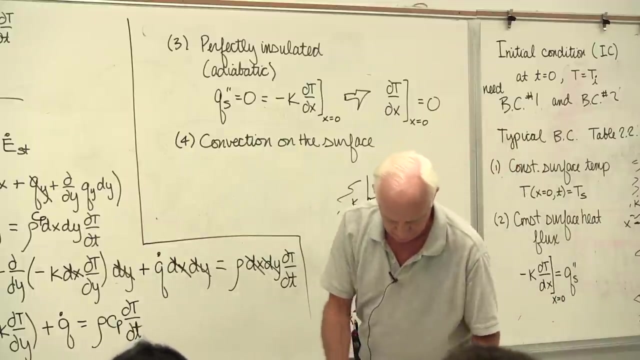 Zero, Okay. Okay, Here's a picture X. Now we have convection T, infinity H on the surface. Surface energy balance says the energy that comes in by convection must go out by conduction into the body. So here's our equation. 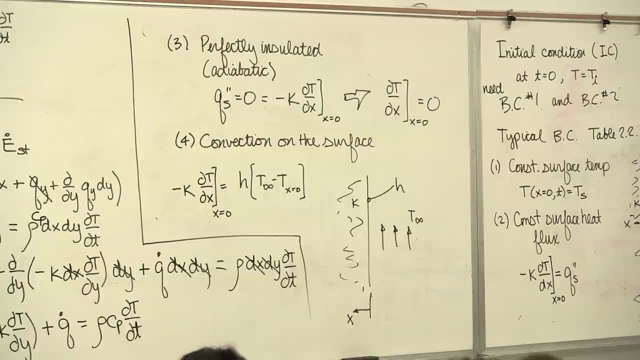 It's more complicated. It has a temperature on both sides of the equation: dT, dx at x equals zero and the temperature at x equals zero. It's a more complicated boundary condition. So you've got the governing differential equation and then you've got the correct boundary conditions. 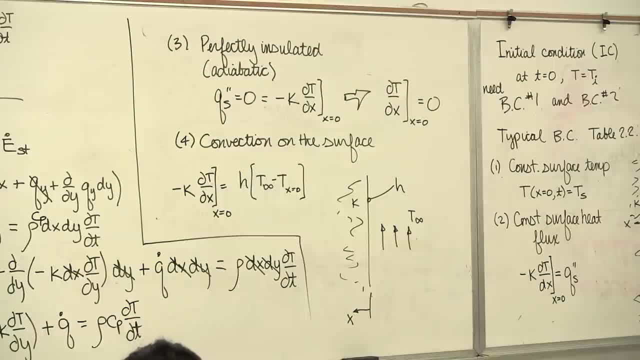 Once you apply those to the differential equation, you get a solution for temperature in the body as a function of x, y and time, if it's two-dimensional. I told you about this constant surface temperature. You know, when steam condenses in a condenser in a power plant. 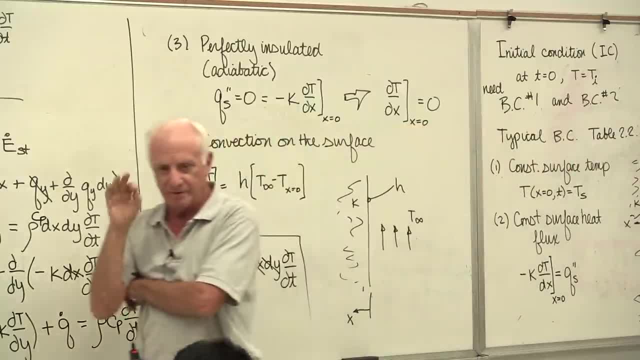 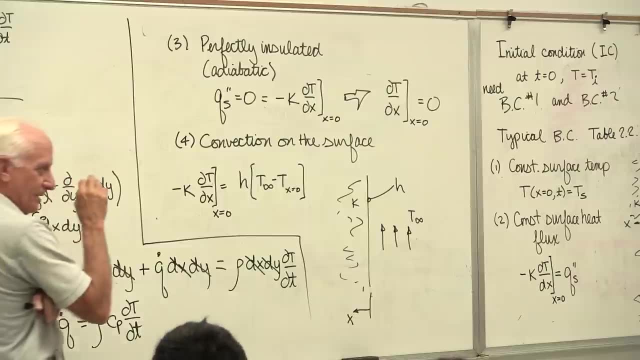 when steam condenses in a condenser at the condenser pressure- you've had thermal, you've probably noticed- it condenses at the saturation temperature of the condenser. So the tubes are like this: in the condenser They're carrying cold seawater, probably Pacific Ocean. 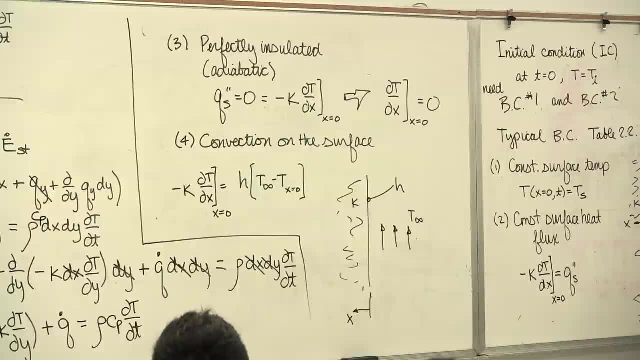 The steam comes in here, It condenses into droplets. at what temperature? The temperature, saturation temperature for the pressure in there. and then, of course, the droplets combine and they go off into the condenser- hot well, Every time they go into the condenser, hot well. 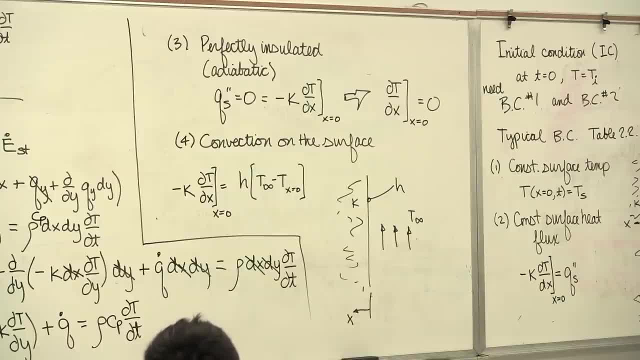 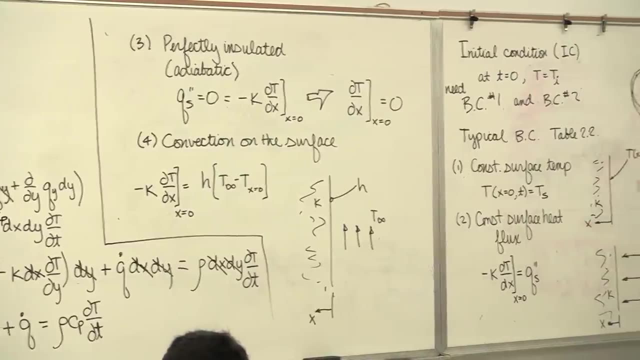 they condense. That temperature is the same, It's a saturation temperature. Yeah, okay, That's this guy. Constant surface heat flux. Oh, you could buy electric-type heating blanket, industrial-type blanket, and slap it on a wall. 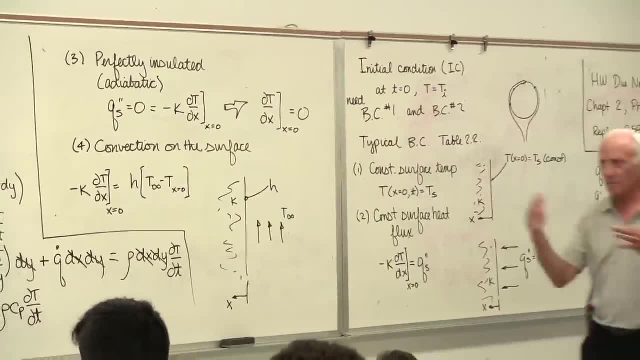 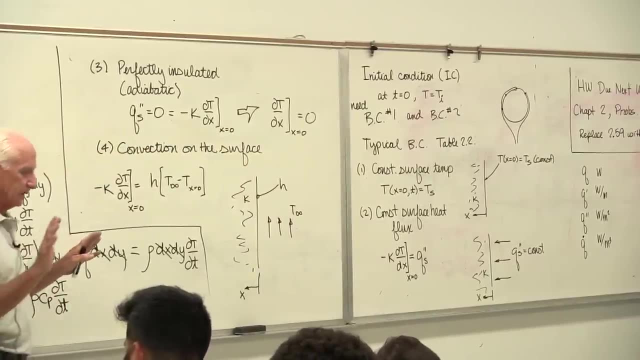 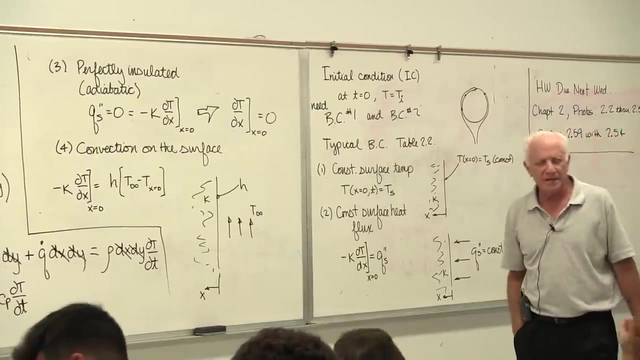 and then hook it up to a voltage supply and provide so many watts per square meter from your electrical conducting blanket on there. Sometimes these solar power plants, especially the one up at 395, and whatever Highway 58, on the way to Mammoth, for instance, 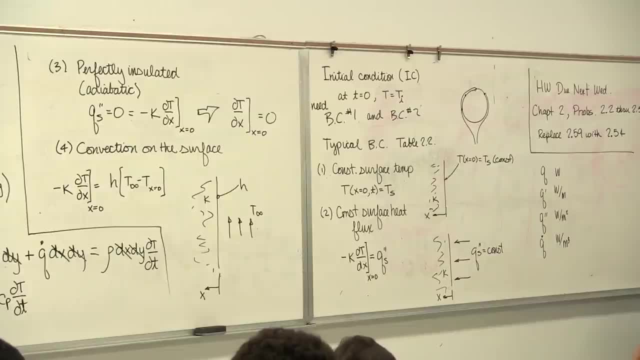 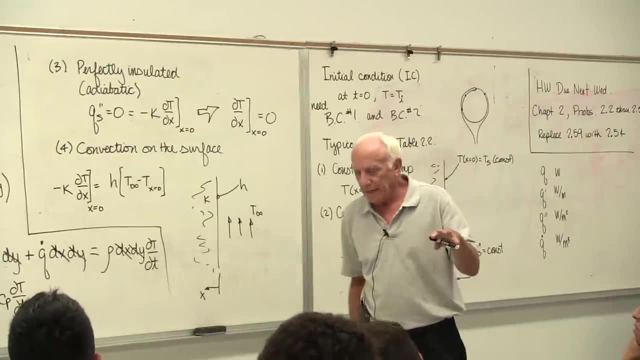 you'll see it on the west side, Big parabolic trough collectors. Some of those collectors carry heat transfer oil in the pipes that go through the focal point And at night they don't run the collectors at night. of course At night there's oil in there. Or you could put the oil back into a big storage reservoir or leave the oil in the pipes. and the pipes are wrapped with the electric heating blanket And they trickle a little bit of power through it, a little current through it, just enough to keep the oil warm. Because when you throw in the morning, when you throw that pump switch on, you don't want cold oil very viscous, Your pump might burn out. So you heat the oil up a little bit so that when you throw that pump switch. 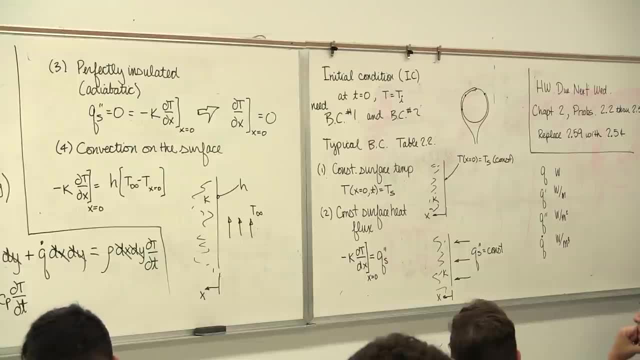 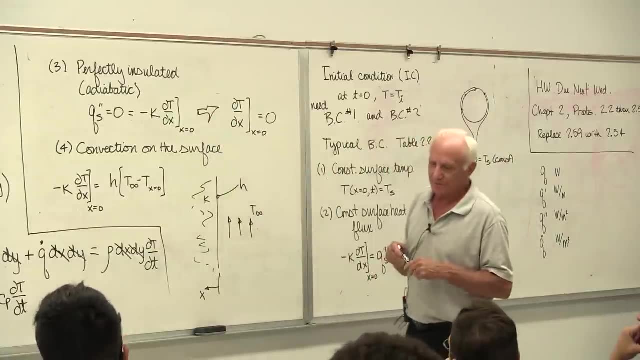 the oil is less viscous So you wrap it in a blanket like that again. Okay, We all know about adiabatic. you know You put up insulation on, it's going to be pretty much adiabatic. You've heard the term adiabatic turbine. 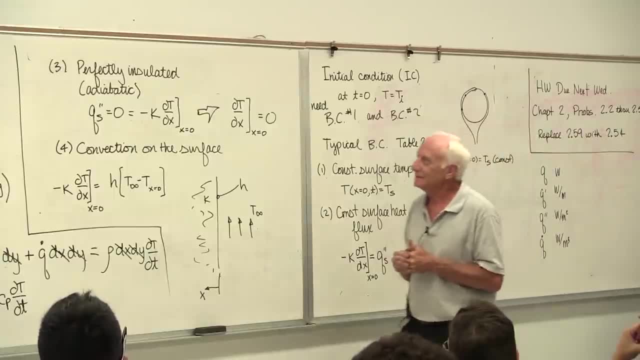 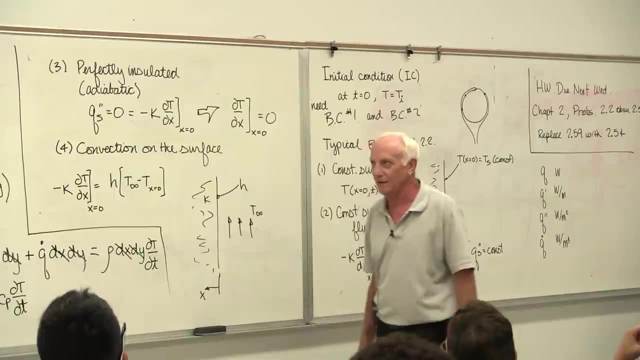 Oh, you know. guess what that means. You know what that means about the turbine. yeah, from thermal Convection on the surface. everything we do on the surface of the earth here is about convection On my body, on this front wall, on the outside wall. 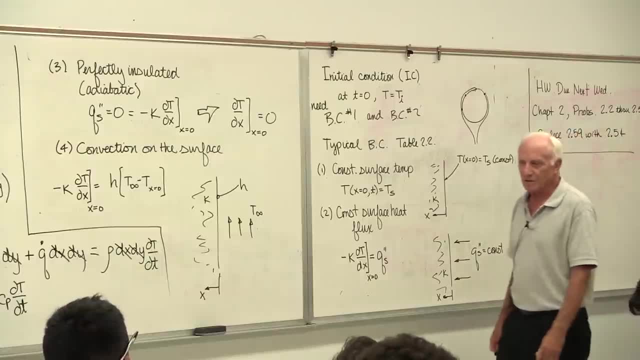 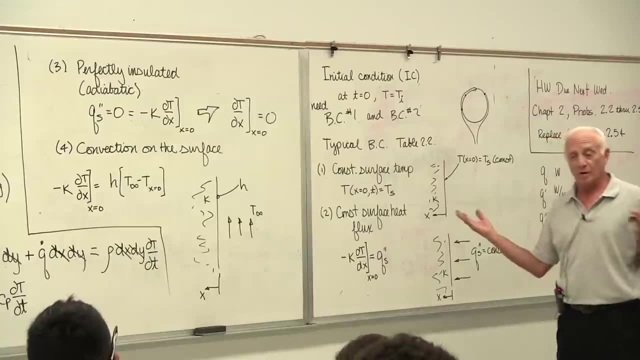 on the tree trunks, on the street, the asphalt, that's all convection. So there's a lot of convection going on, Okay. so anyway, and there's more, There's more. Obviously, we're building some kind of space vehicle. 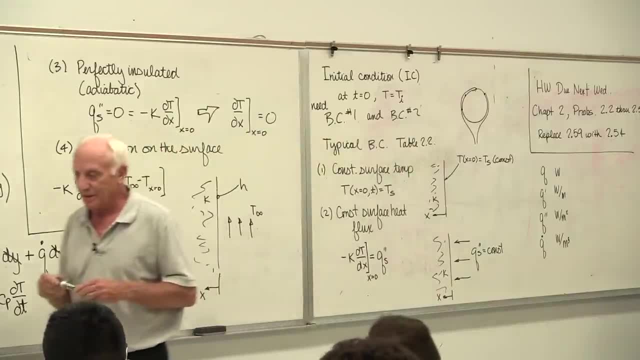 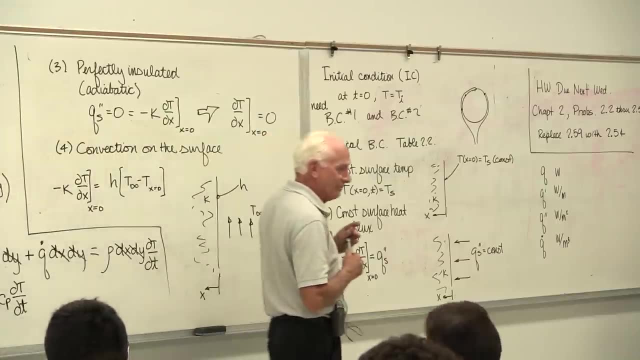 We can't. there's no conduction, There's no convection, It's all radiation. I don't have radiation up here because that's for the advanced group. okay, Radiation is a tough boundary condition. The fourth order in temperature. 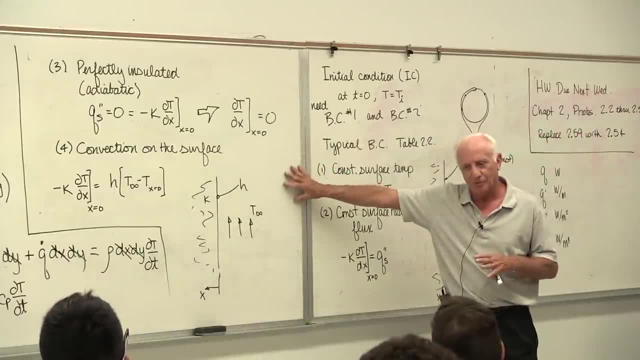 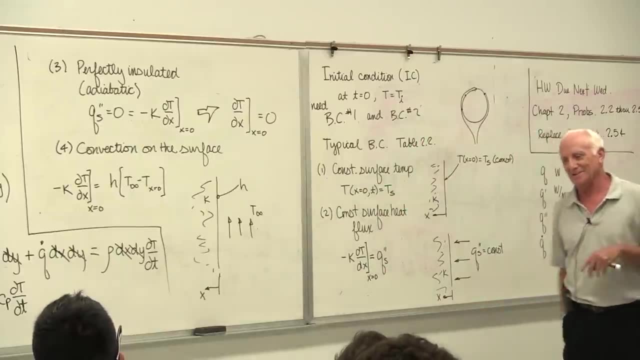 So, no, we won't be considering radiation on this list, although in the real world, yes, it does happen frequently. Okay, so these four are the only four you're going to be responsible for in our heat transfer course. Okay, so now we have that set up. 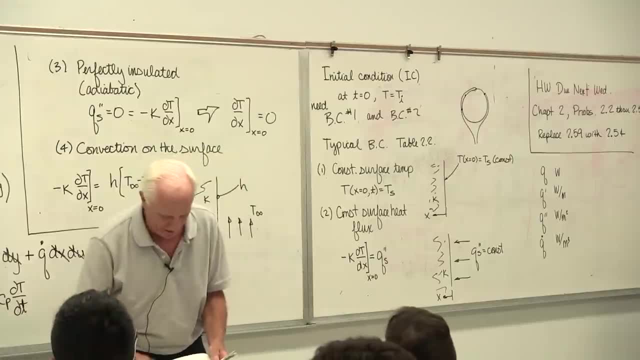 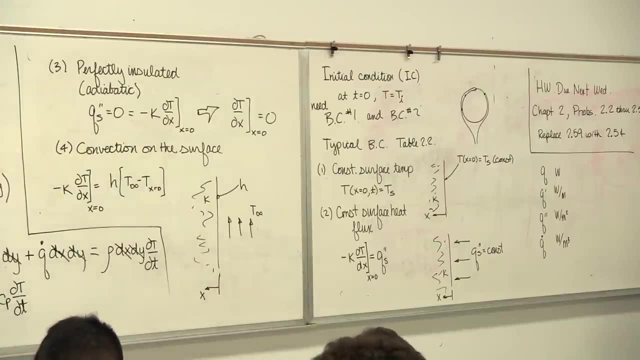 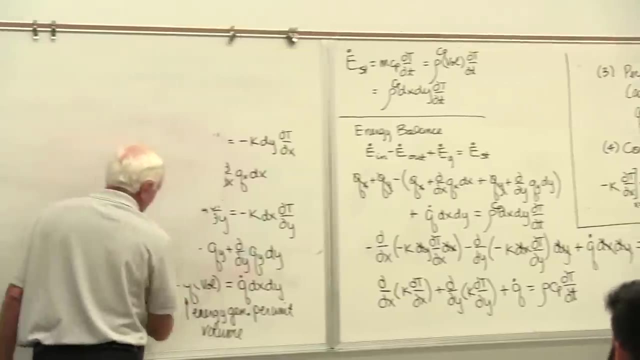 The heat diffusion equation with the correct boundary conditions. Okay, let's look at some problems to see how we use all this material in Chapter 2.. We're going to start off with a very early problem. You'd think problem 2.1 would be the easiest problem. 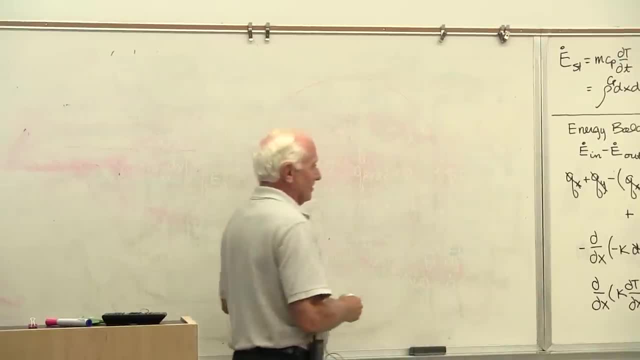 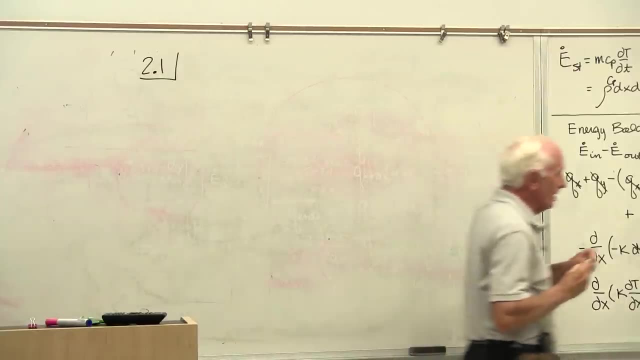 in the whole homework set at the end of the day, End of the chapter, not true, not true? So problem 2.1 is very similar to your homework, problems 2.2 and 2.3.. So I'm going to go through 2.1. 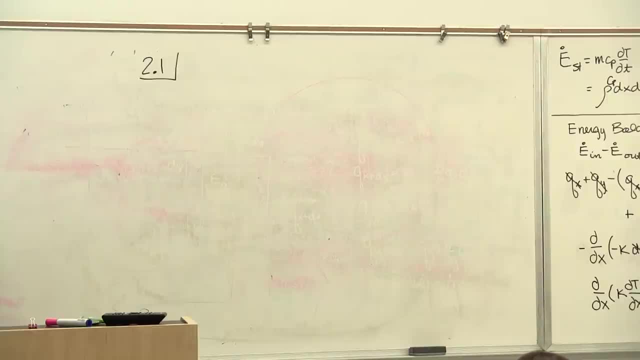 to give you some major hints how to work that, Let me read it first: 2.1.. There's a picture given in the textbook. Okay, it says we have heat conduction through an axisomal symmetric shape shown. So it looks like this: 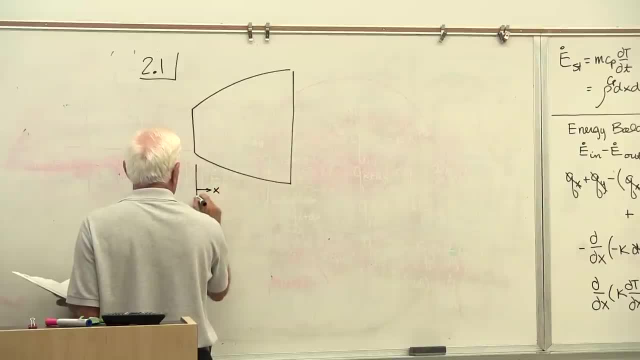 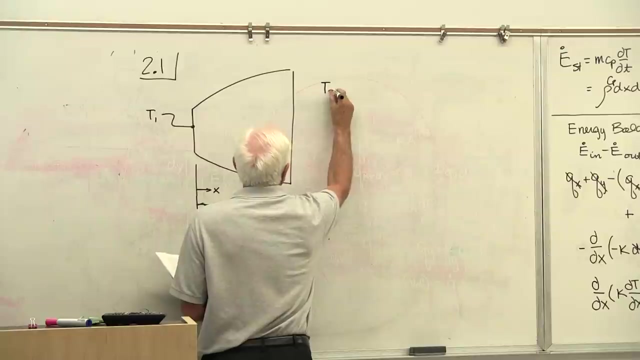 We're going to measure in x from the left-hand side. This is x equal L, He tells me the temperature on the left-hand side is a constant temperature at that surface and the temperature over here on the right-hand side is a constant temperature. 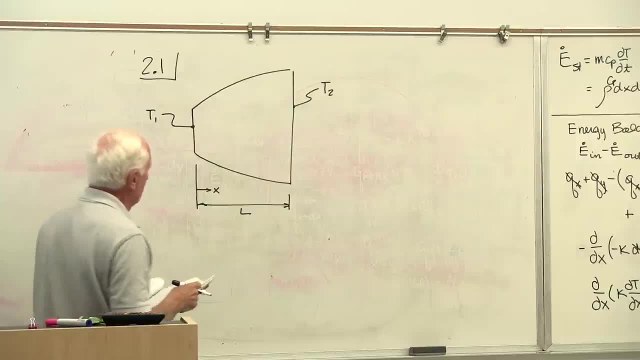 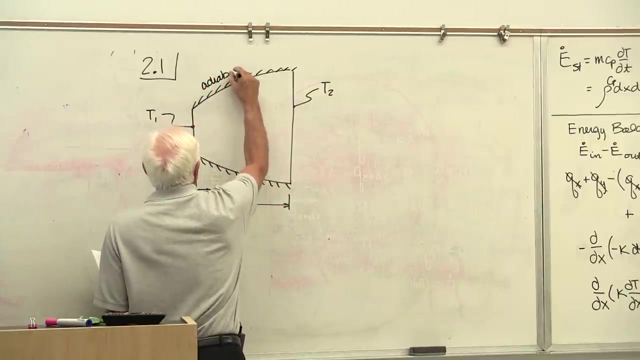 on that surface, Given constant surface temperatures. He doesn't tell me he should and I would definitely do that on a problem that the sides of this are adiabatic, perfectly insulated. Let's see what else we're given here. 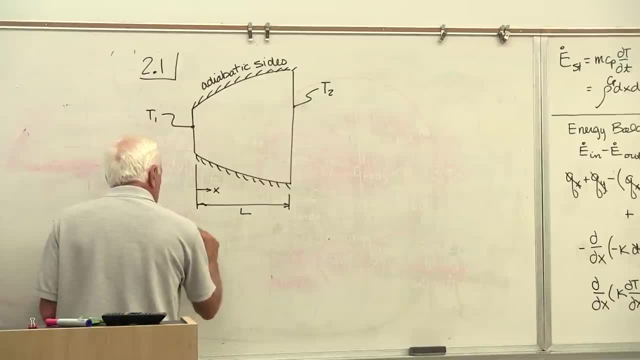 He says: assume the problem. says this, assume. assume. Assume S-S steady state, Assume one-dimensional heat's only transferred in the x direction, Assume constant properties, Assume no internal generation, Okay, Okay. And then he says: sketch the temperature distribution on Tx. 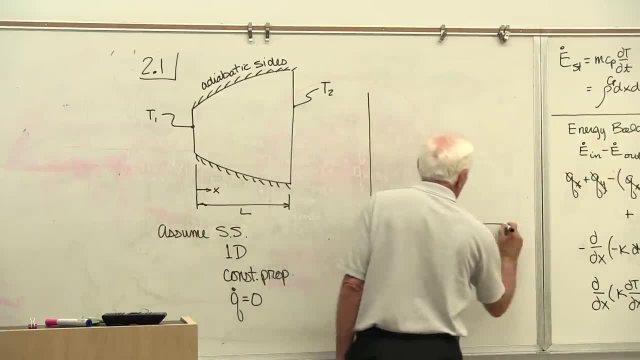 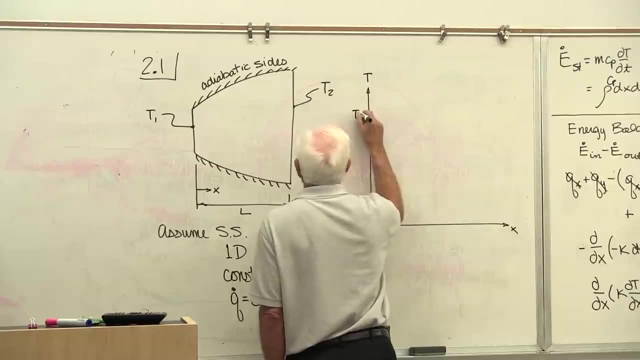 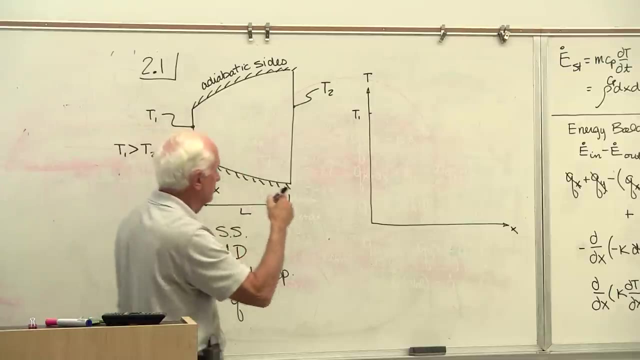 coordinates. So he wants you to T1.. He tells me, by the way, that T1 is greater than T2.. So I know T1's a hot side, T2's a cold side, T1 and then L, T2.. 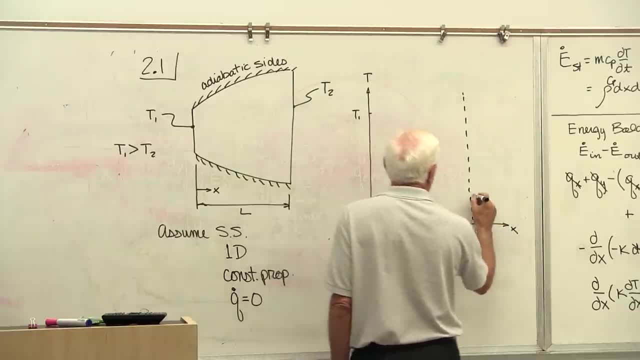 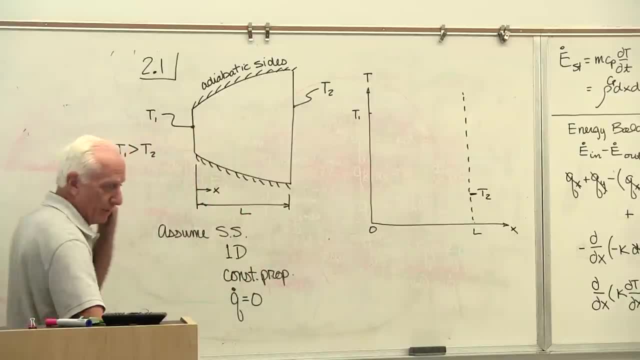 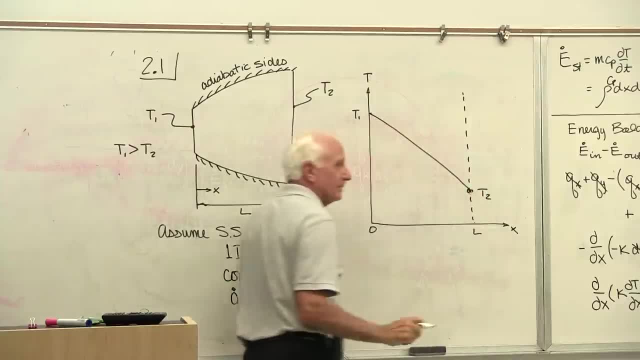 straight line. Why shouldn't it be a straight line? Okay, That's one possibility. Then you might say: well, you know, it could be a little bit of curve to it, so I don't know, Maybe it looks something like this: 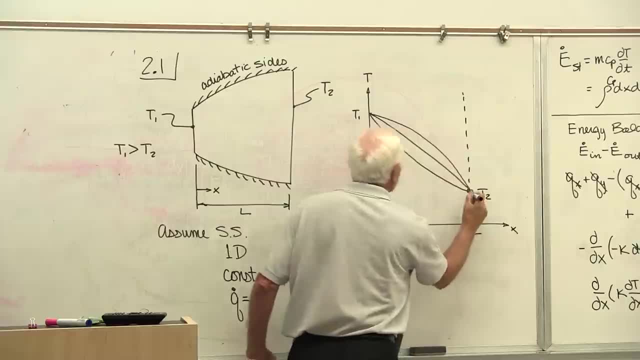 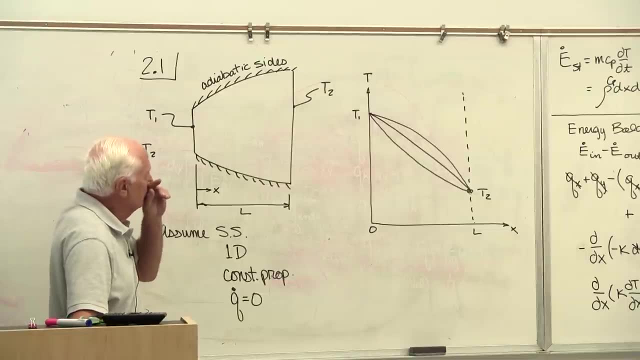 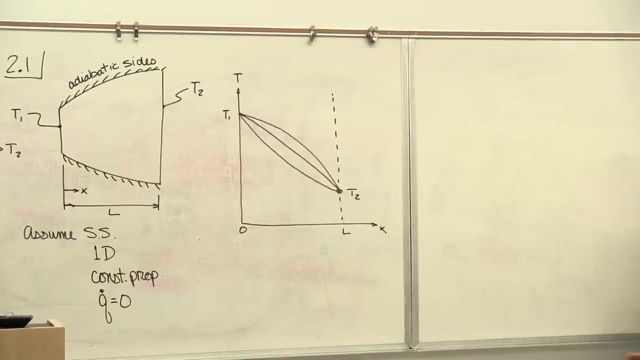 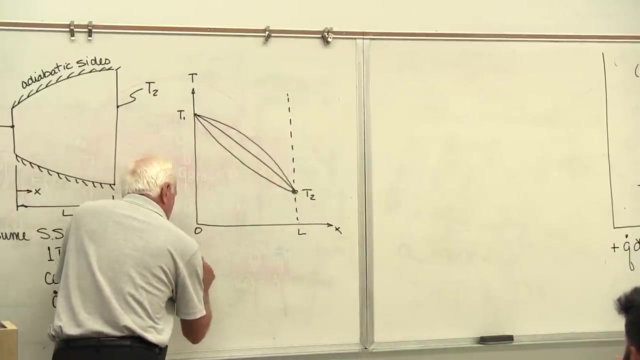 Or maybe it'll look something like that. Those are all possible shapes. Well, okay, The problem is conduction, heat transfer. So we're going to write. Let's just do something first. to make it simpler, Let's do energy balance. 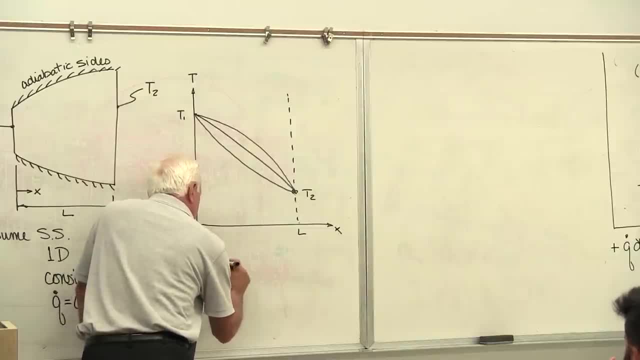 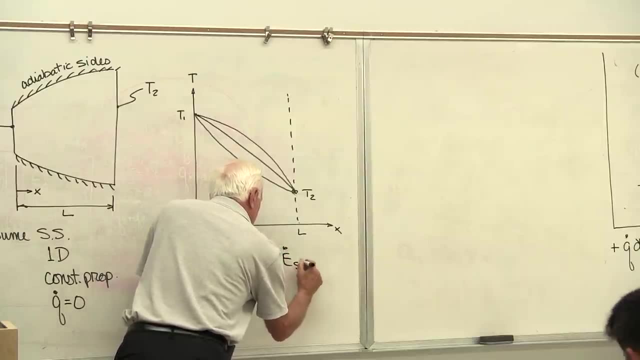 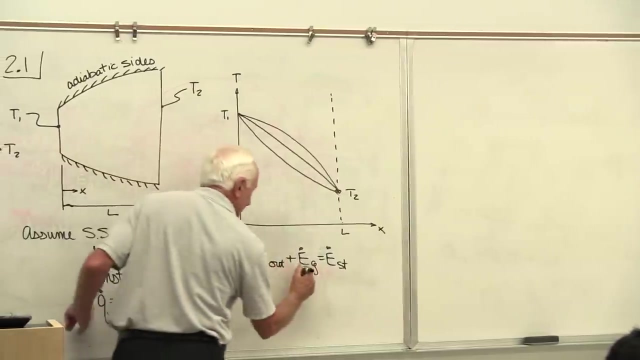 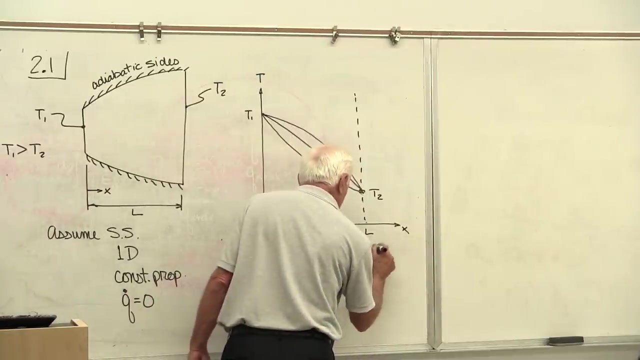 E dot in minus E dot out plus. E dot gen equal E dot storage. Now he said that Q dot zero. Okay, Goodbye. He said Steady state, Goodbye. Conclusion: E dot. that comes in the left-hand face. 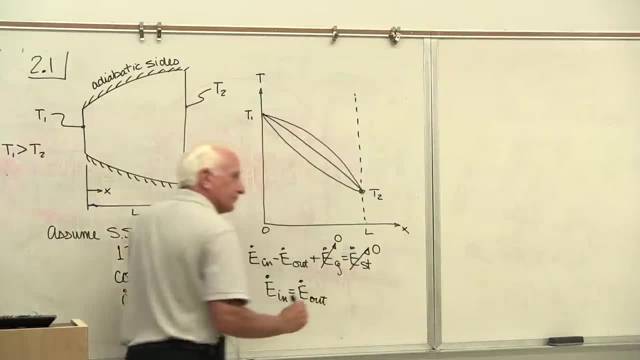 must equal E dot that goes out the right-hand face. If I have 50 watts coming in the hot side, 50 watts has to go out the cold side. Where else can it go? The side walls are adiabatic, perfectly insulated. 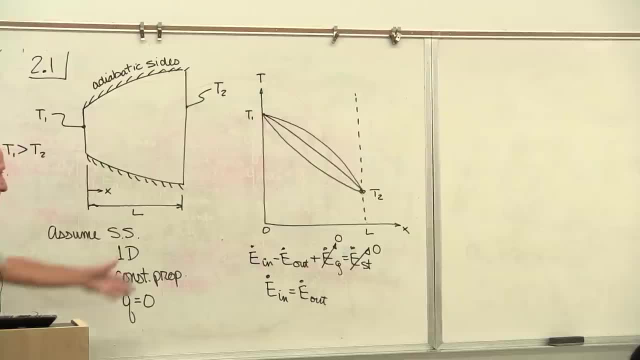 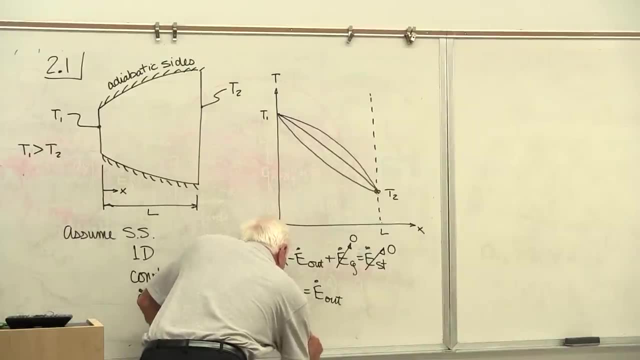 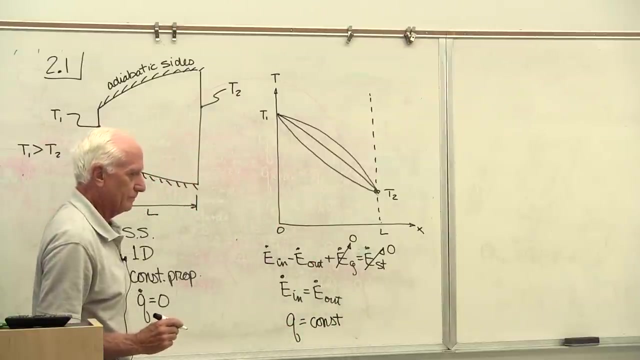 There's no generation, It's steady state. That's what the energy balance tells me. So right away, now I know what that means. That means that Q in watts equal a constant Constant. Okay, Let's then write down conduction. 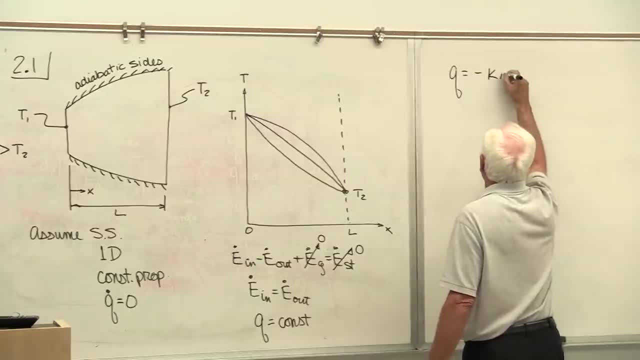 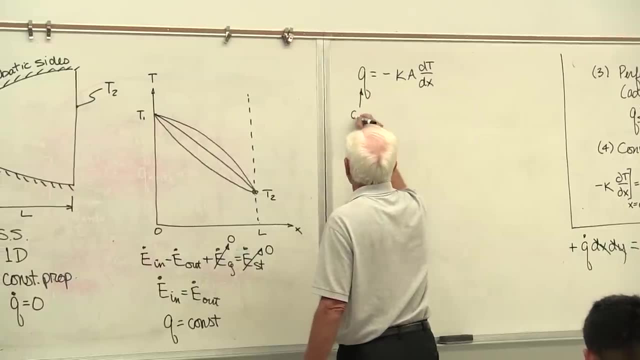 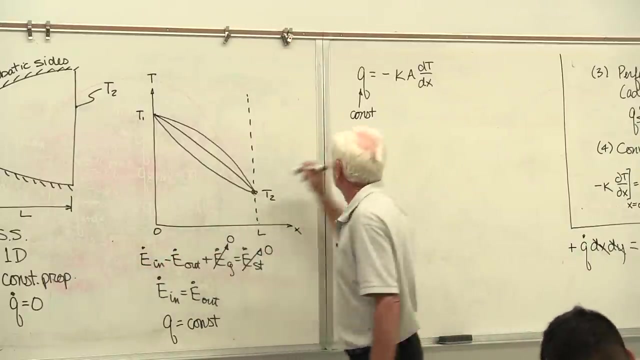 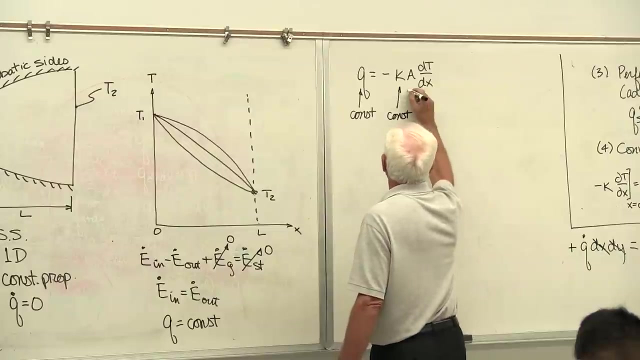 Fourier's law Minus K, A, DT, DX. Okay, Let's write that down. Q is, I just showed you, Constant. Problem said: Assume constant properties Constant. It says then conclusion that this thing right here must then be a constant. 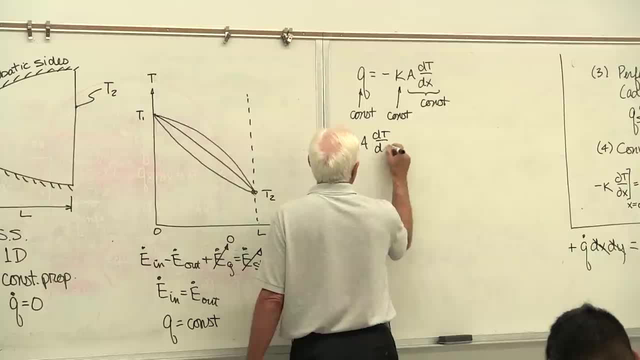 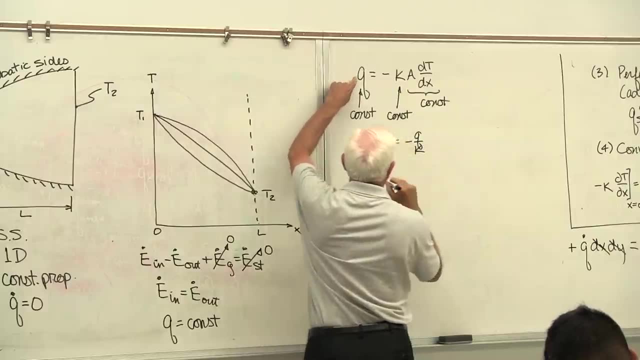 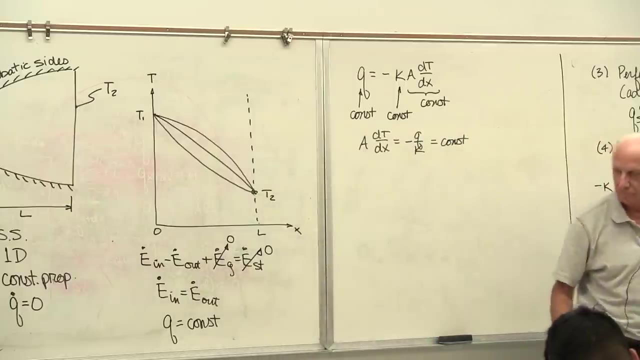 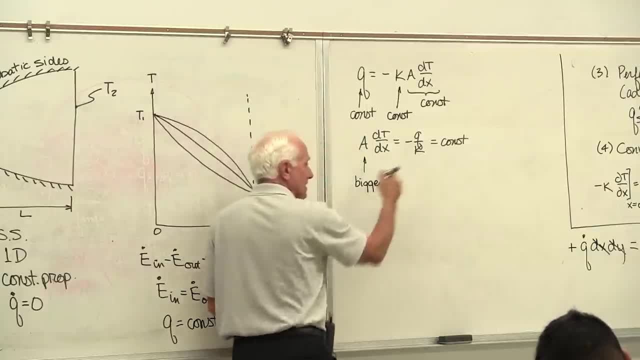 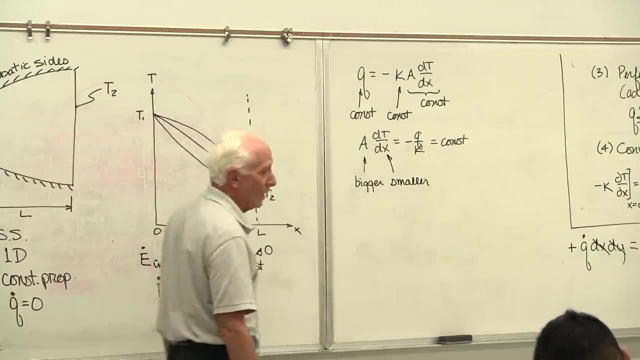 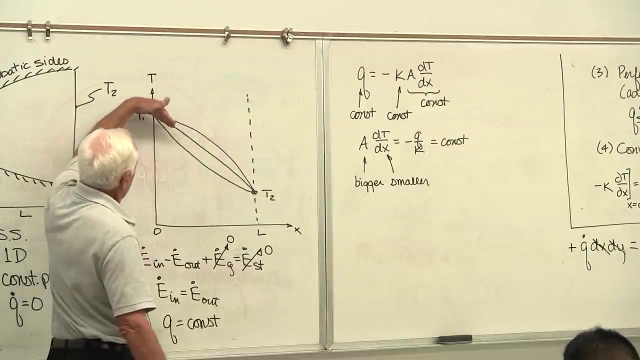 If you multiply this bigger number by another number to get a constant, this guy better be getting smaller, Otherwise it wouldn't stay constant. What does that mean? That means as x increases, the slope dt dx must be getting smaller Slope dt dx. 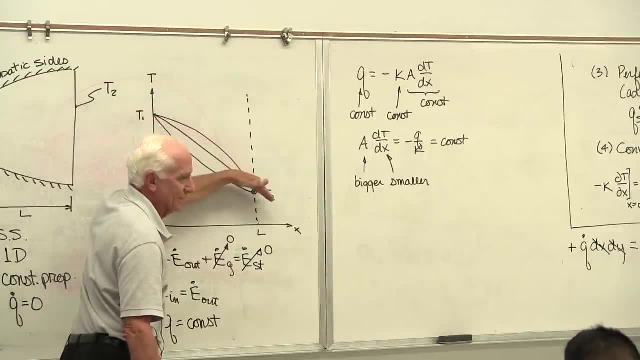 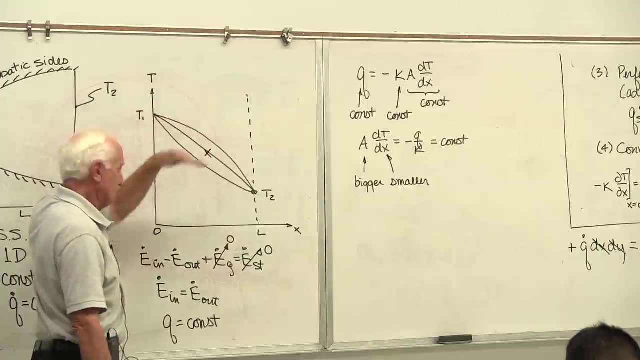 Slope. dt dx Slope is here at this location, Same slope. That's not working. It's not that one Uh-uh Slope didn't change at all. Don't forget a steep slope, Steep slope, shallow slope. 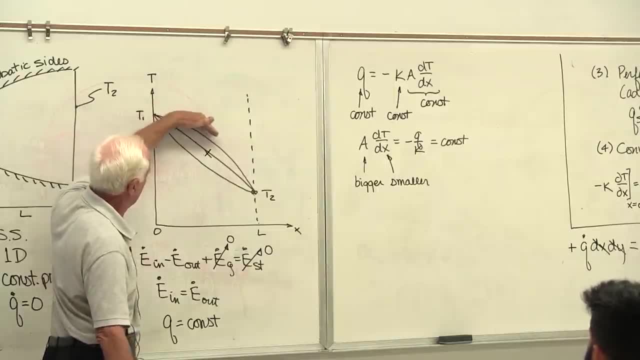 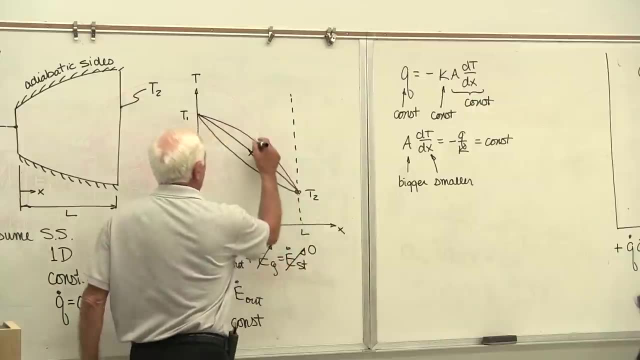 Okay, Here's a slope here. Okay, Go down here. Ooh, big big, big, big, big, Small slope, Big slope. No, uh-uh, you've got it, that one Big slope, Small slope. 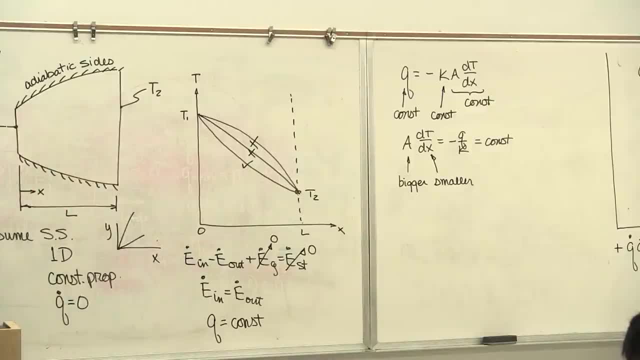 Yep, that's it, That's it. No numbers. Sometimes these problems drive people crazy. They say: please give me numbers on an exam, Don't give me symbols. I hate symbols on exams. I want numbers. I know. But sometimes you know, sometimes this helps you develop engineering intuition. 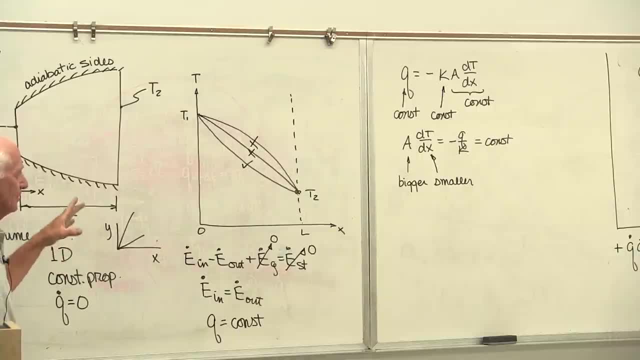 That's the important point. It helps you to draw something without ever having to solve the governing partial difference. Okay, So it's a differential equation. Okay, That's the key. All right, so that's how we prove that guy. 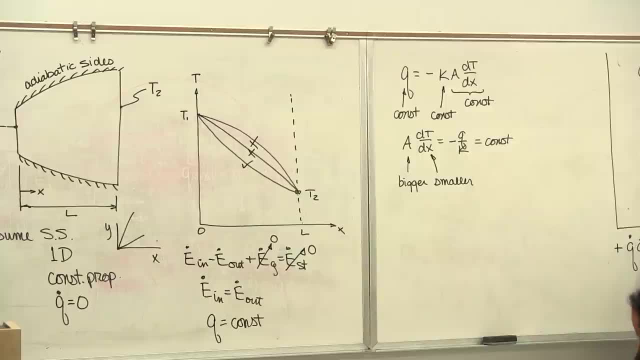 It's that one right there. Okay, If you want to look at Q double prime, Q over A- what happens here? This guy numerator is constant Denominator. as X gets bigger, becomes bigger, Okay, the area gets bigger. Conclusion: Q double prime gets smaller. That's kind of intuitive. 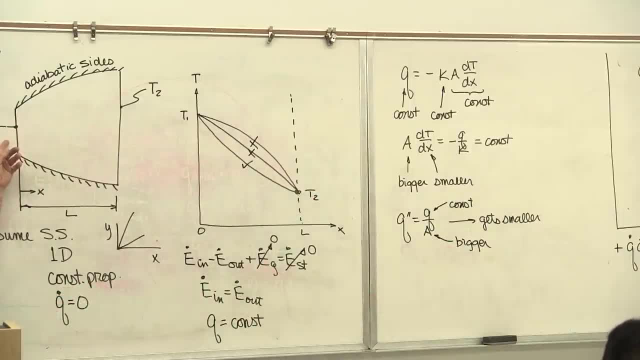 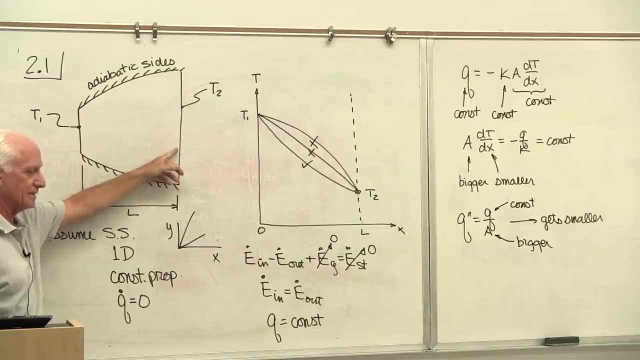 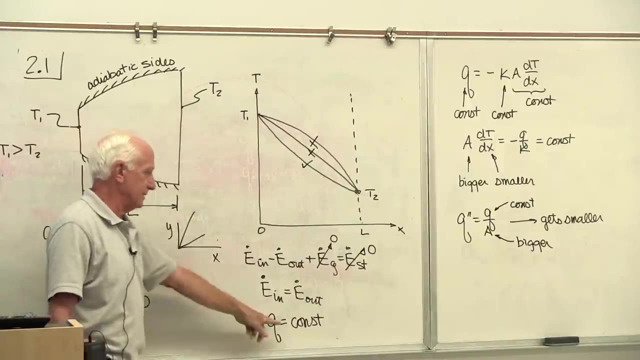 If I've got 50 watts here divided by a small area and 50 watts here divided by a big area, yeah, Q double prime gets smaller. as X increases Q, though 50 watts in here, 50 watts crosses here, 50 watts crosses here, it stays constant, Q stays constant, Q double prime gets smaller. 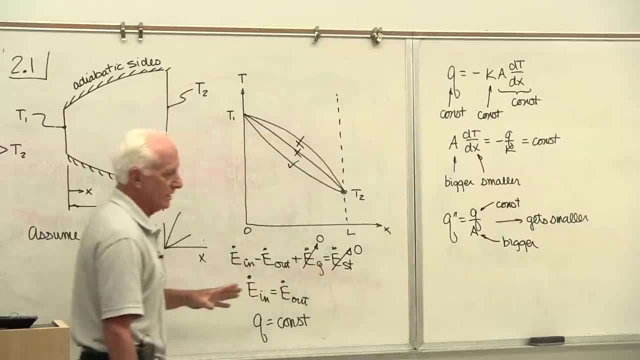 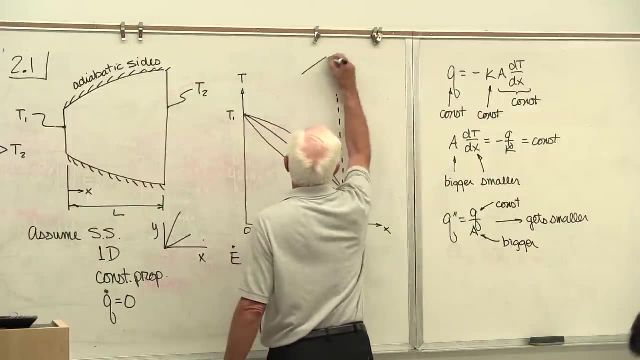 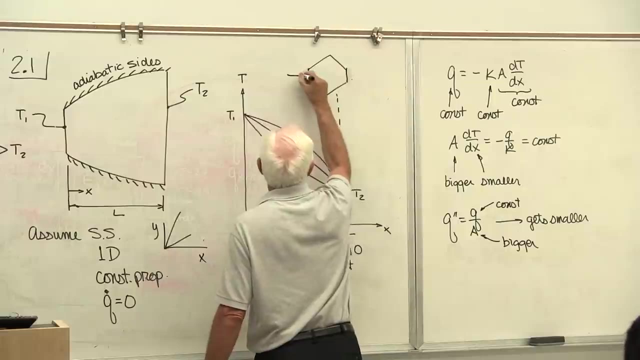 and the slope DTDX gets smaller. A lot of stories in there. So your two problems are very similar. The problem 2, 2, 2 looks something like this: I think it looks. yeah, it looks like this compared to that guy. Okay, so 2, 2 and 2, 3 are very similar. 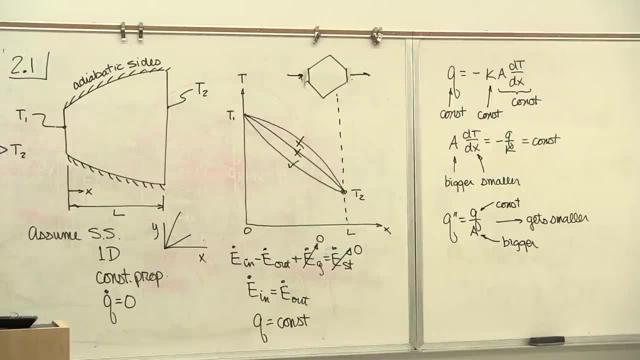 Use my solution as a guide for you All. right now, let's talk about the homework that I passed back. so you know what's going on with the homework. All right, let's see. This is what was passed back. This is what's due today. That's what's due next Wednesday. Okay, 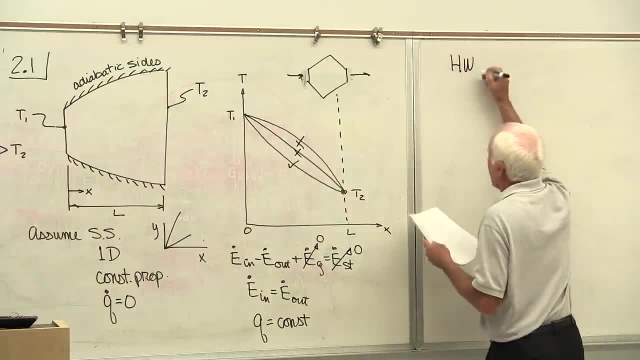 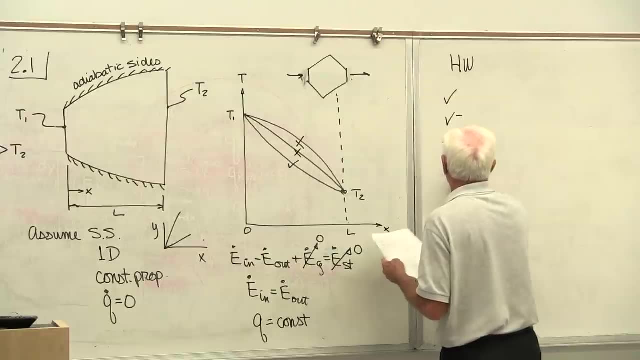 So, on the homework, you can either get a check, a check minus zero or an asterisk. And if you had me for fluids 311, you know how I do this. so it's not any news to you, but we'll go over it. I'm going to pick up 12 homework sets. I'm going to have 12 grades. 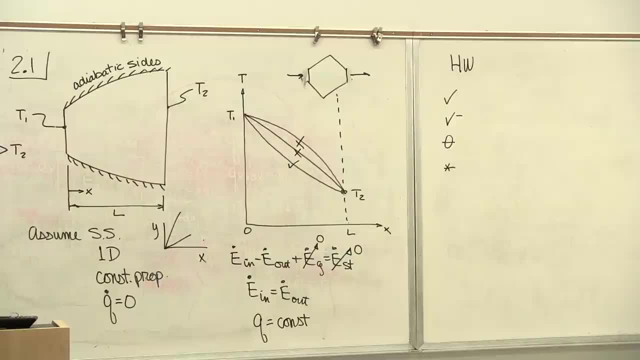 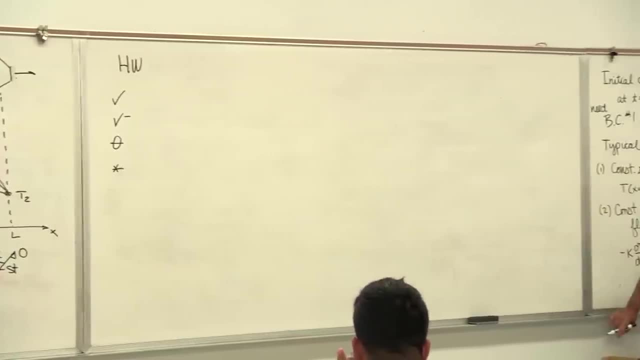 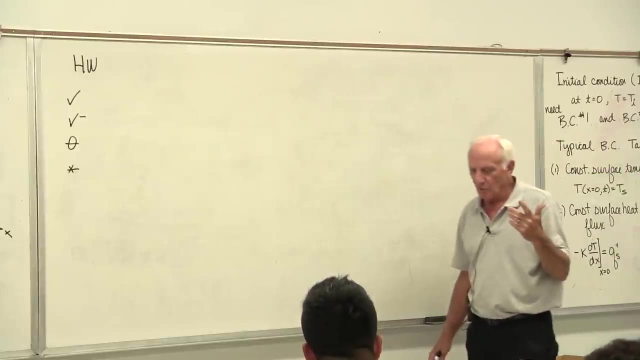 in my grade book. I'm going to knock out the two lowest grades and keep the top 10 homework scores Each homework set. you can get one of those four scores in the upper right-hand corner by your name. typically You'll see the symbol If I assign eight problems and I grade one. 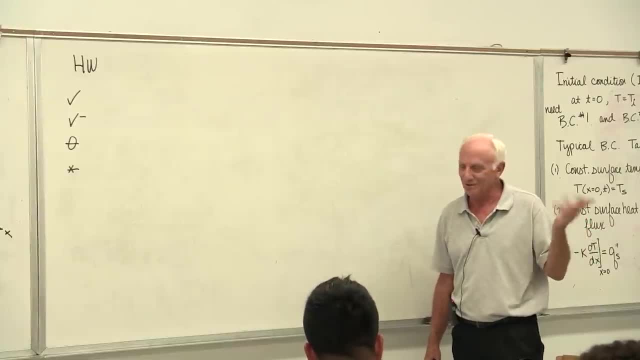 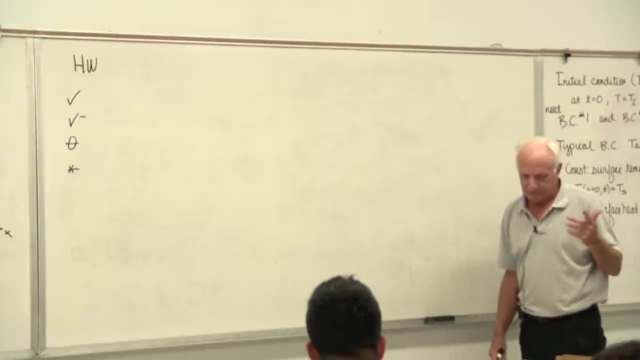 or two. let's say I grade one. I graded one this time, The first problem. just look at it, You get a check. Okay, If I pick up a homework set with 10 problems and I grade two of them and you got them both, pretty much all right, you get a check. 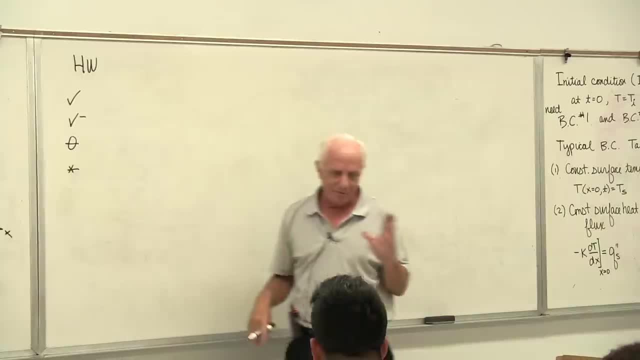 If you worked one and got it all right and worked one and didn't get it right, something was wrong or the wrong equation or the dimensions were messed up, then it'd be a check minus. If I pick up 10 homework problems and I grade two and guess what The problems I grade, 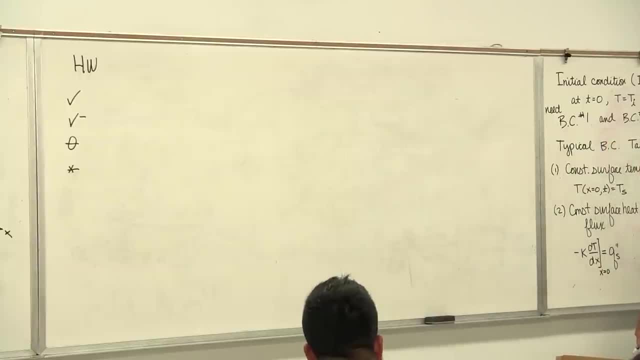 are the problems you didn't work out of the whole set. You worked eight problems out of 10, and guess what I do? I grade the two problems you didn't work. You know Murphy's Law, Oh my gosh. The zero means you didn't work the problems I graded, but you worked a lot. 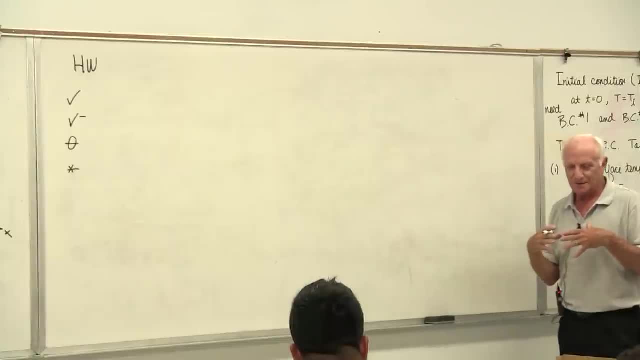 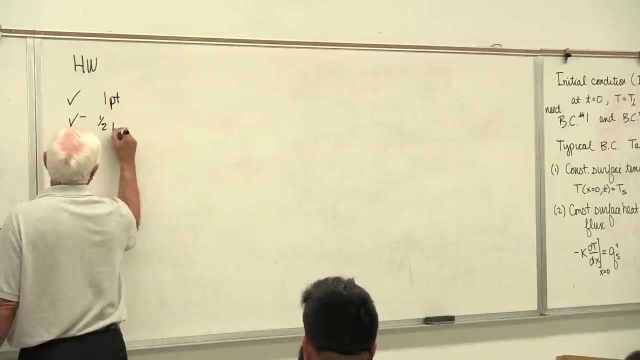 of the rest of the problems. okay, I kind of look and see if you've done the rest of the problems. So that's what the zero means. Okay, This guy counts one point. This guy counts a half a point. This guy counts zero points. The asterisk means nothing was turned in. 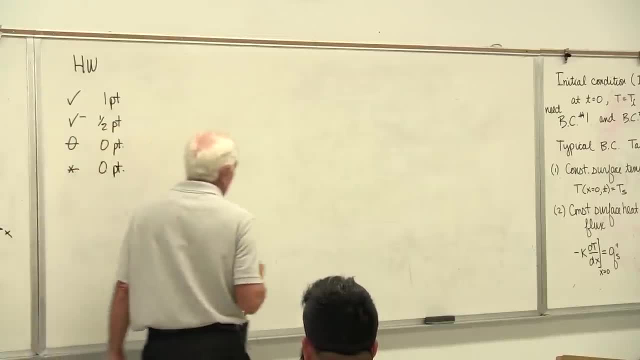 Okay, This is zero points. Avoid the asterisks. Okay, That tells me that you didn't think my homework was worth working. Okay, And my ego gets crushed- Okay, So I'm going to do this. My ego gets crushed, So it really makes me a bad day, you know. So avoid those. 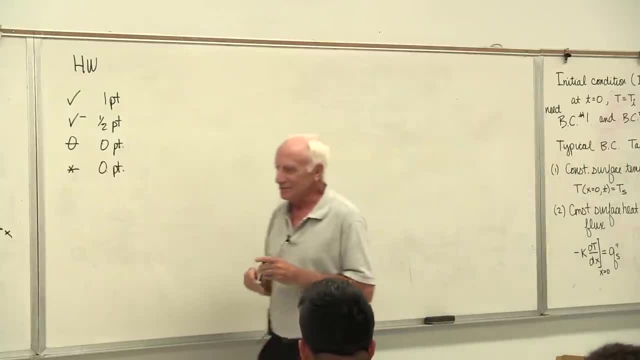 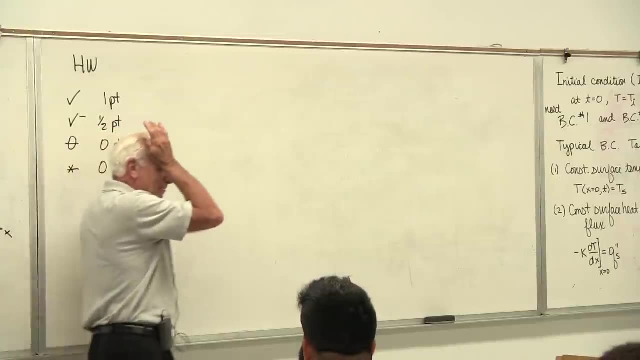 little asterisks because they can come back to haunt you. If you're sitting there, I'll be real generous and say you're at 89.4.. 89.4.. Gosh By the book, if I round off as an 89,. 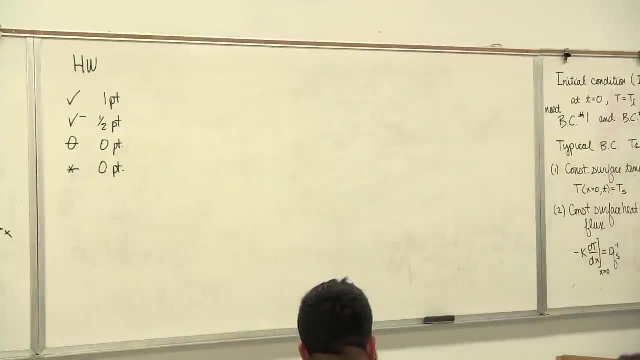 and by the book that's a B plus. Could it be an A minus? Gosh, within six-tenths of a point. One thing I'll do is I'll check the exams and say, well, the first exam, not too. 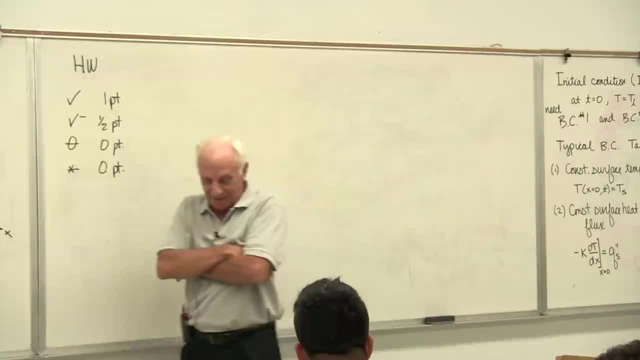 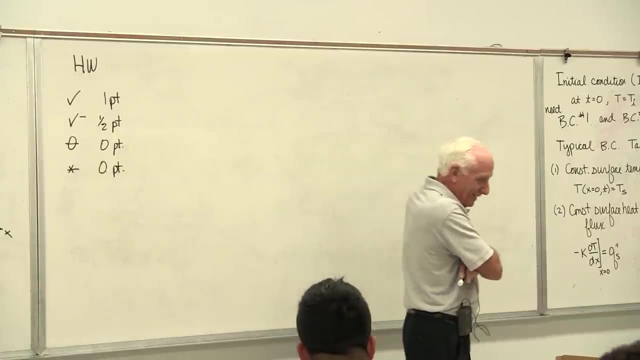 good, I don't think you knew how I gave exams yet, But the second exam was better and the final was even better, So it's some improvement. So I'll take that into account. And then I'll say: let me check the computer problems. I assigned two of them. Okay, Out of a total. 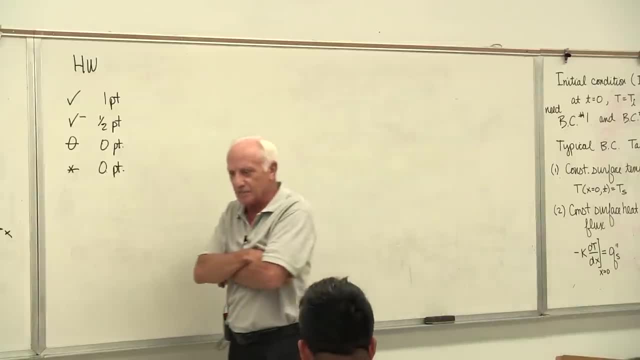 of five points. this person got four. Okay, Decent, Try each one And then I'll check the homework. And you know, I see ten homeworks. I'll check the homework. I'll check the homework, That's. I'll see six asterisks. It must have been a busy person, Must have been carrying. 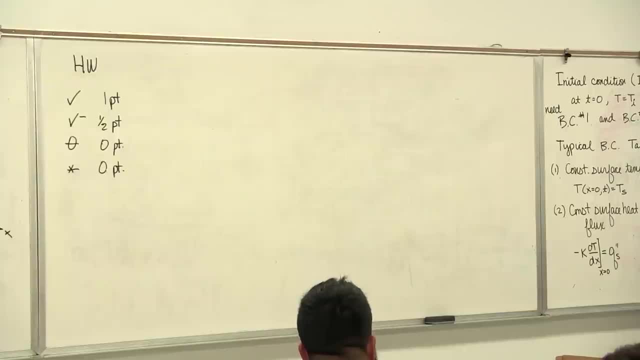 22 units because he had no time for my homework. I don't know Should I go up with the B, Should I keep it there or should I reduce it down. I don't know. Homework's important So I don't like to see too many asterisks. It's okay, I'll tell you. you know it helps you. 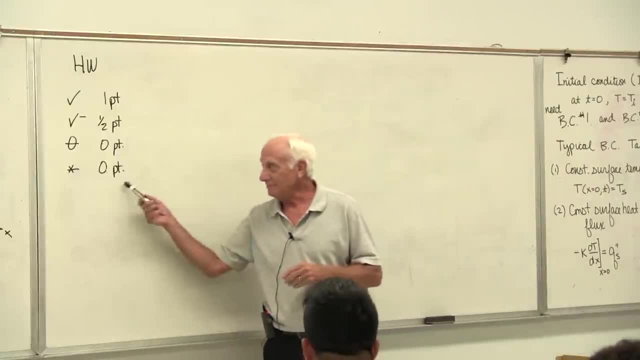 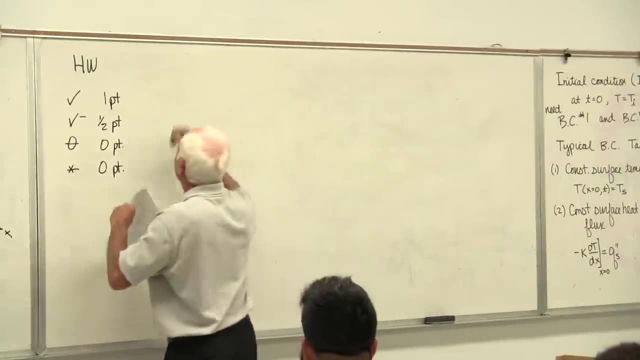 to do the homework. as you know, when you're studying for the final, All right On the homework At the top of the page, yeah, your name, of course. So you've got your name, Then you've got M-E-415-O-2.. Then you've got homework set number one. Okay. 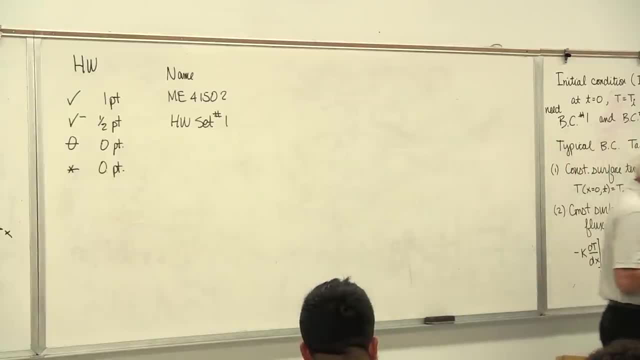 The reason why I like to see that O-2 there is because I'm grading section one and section two And I've got 34 and 34.. And I'm grading to homework sets. I've got 130-something problems to grade Anything. 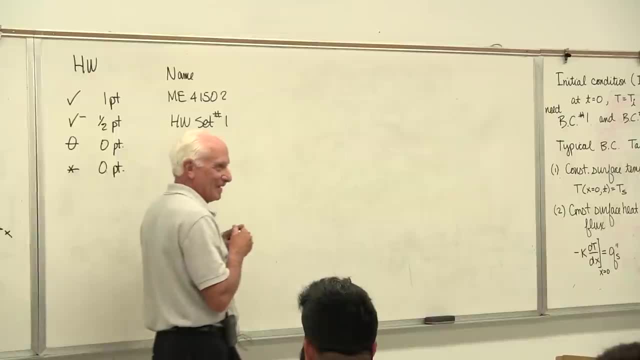 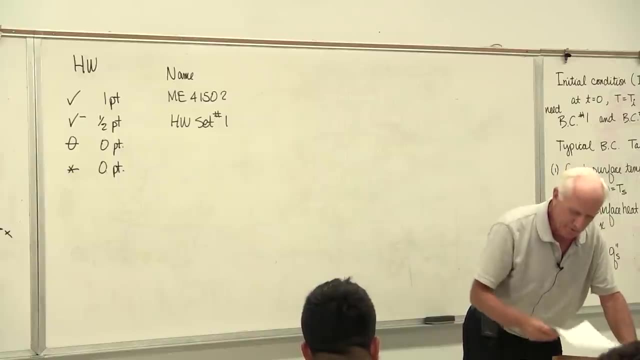 you do to make my life easier while I'm grading will help you. I guarantee you It'll make me happier, Okay? So if I happen to mess up these problems somehow, I think: oh no, Where is Gina? Is she in section one or two? Where does this go? Well, you know, I check. 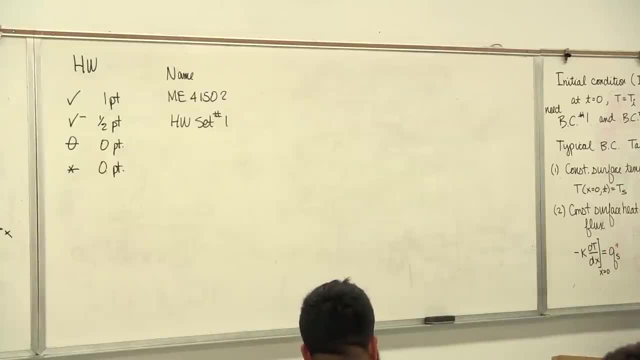 my grade book, of course, But it's easier if you do that for me, Okay, So that helps me. Number two: this helps both you and me. Near the end of the quarter, the ninth week, you say: gosh, I'm kind of worried about my grade in this class. You come and see me and say: 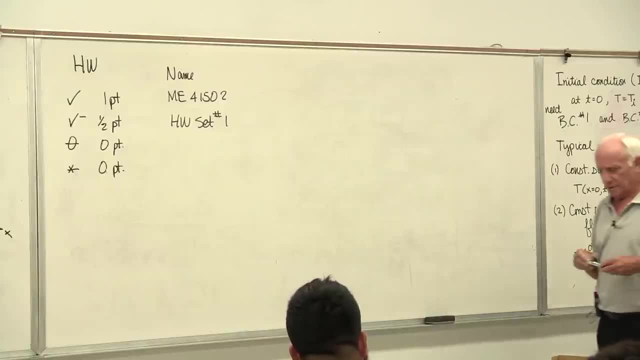 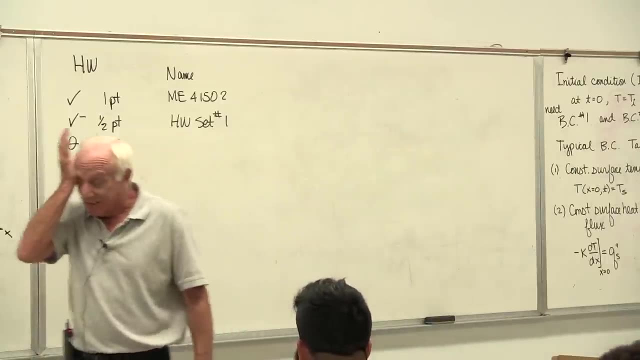 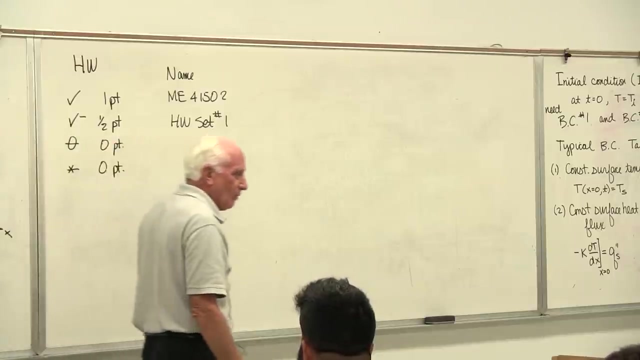 Professor Biddle, what do you have down for my homework score? And I say, well, I've got down six out of ten. And then you say, well, you know what, I've got seven out of ten. I say, oh really. I say, well, I've got a zero on homework set number three. Well, if 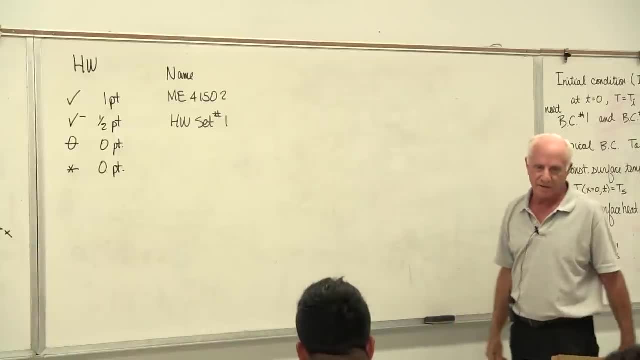 you mark these things like one, two, three, four, five, six, seven, eight, nine, ten, ten, fifteen, twenty, twenty-five. six, six, seven, twenty, twenty-five. it's easy to find three. 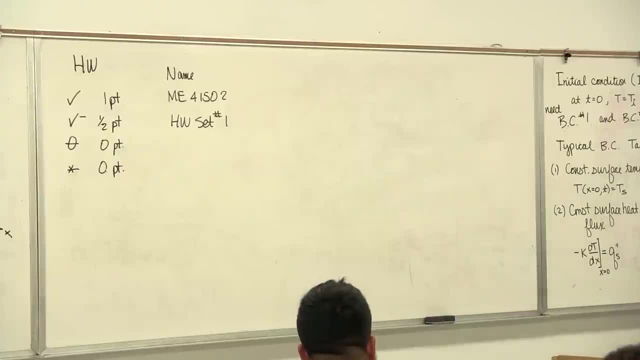 If you say nothing or maybe problem so and so and so and so I'll say: I don't know were those problems in set three or four or five? So it's easy for me and you when we talk about your homework grade if something is wrong, you know you don't agree with my. 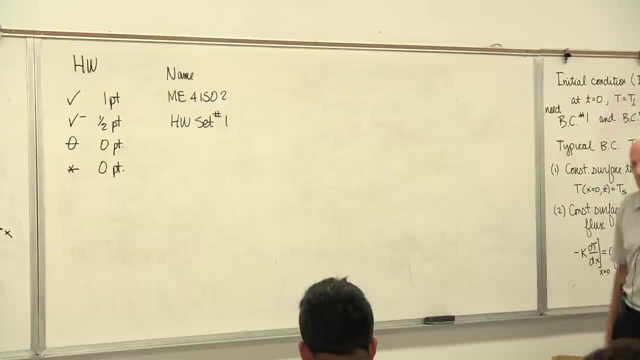 homework grade. we'll check every set and see which one is missing and why it's missing. So that helps both of us. So now, if you do a problem, let's take a problem easy: one. Two equal two minus three. Two equals two. Let's take this. one. Two equals three, Let's. 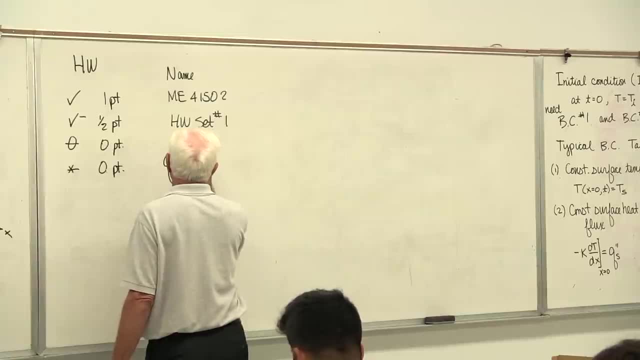 look at these problems: Two equals three, Two equals three. Let's take this one: Two equal zero, Two equals zero, Two equals zero, Three equals zero, Two equals three, Three equals three. let's just do K. let's do Q, double prime K, delta T over L. 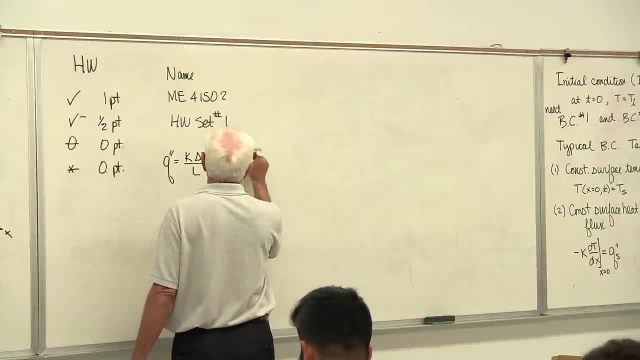 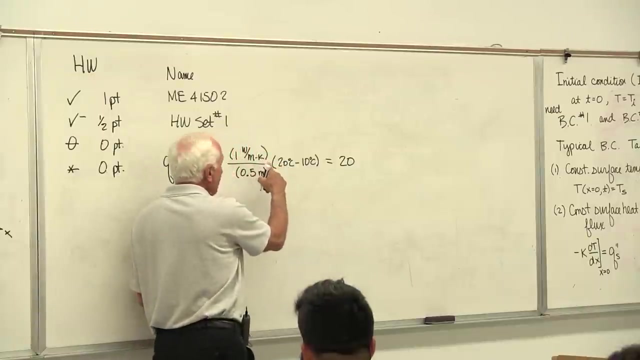 So K is 1 watt per square watt meter, K L is a half of a meter And delta T is 20 degrees C minus 10 degrees C, Equal 2 times 10, 20.. If you don't like degree K, if you don't like degree K, take your eraser. 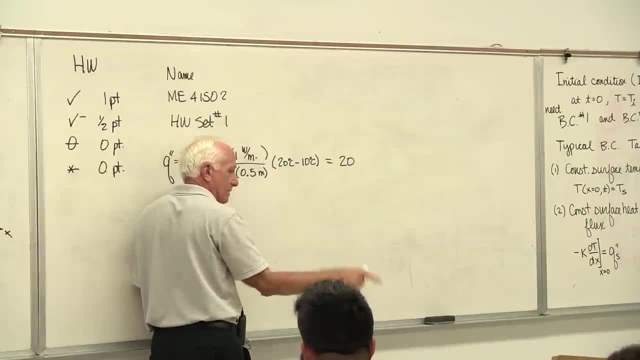 That's from the back of the book. 1 watt per meter, degree K in the appendix. Take your eraser and make that a degree C. We said before that's legal Cancel, cancel Watts per square meter. So when I look at the problem, 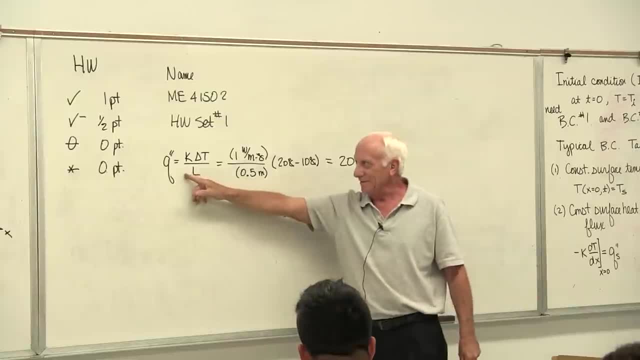 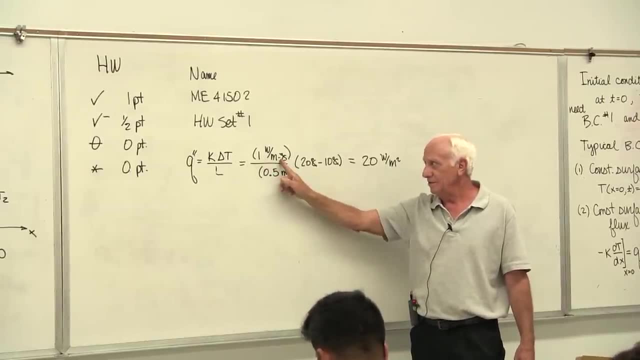 I'll see. did you put down the version with just symbols, the symbolic version? Did you put the numerical values in? Did you put the units in And did you get the right units when you were done? Okay, those three things. 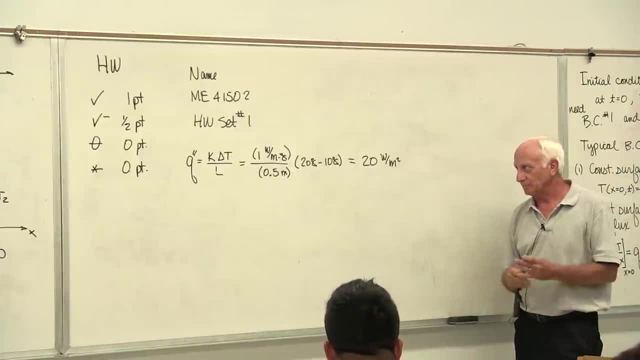 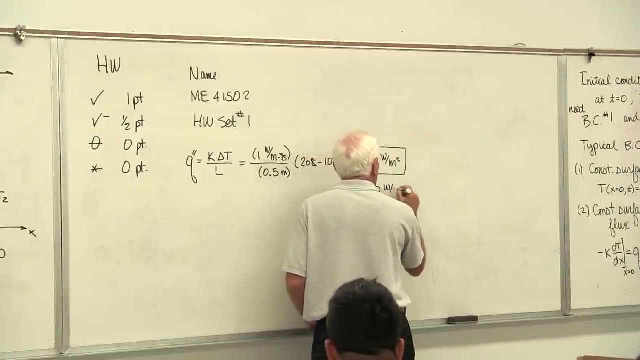 Symbolic equation, the numbers, the units and the answer. On the answer, you know a lot, of, most people will do that: box it in. Some people will do this double underline. Some people have all different ways of doing it and I don't care. 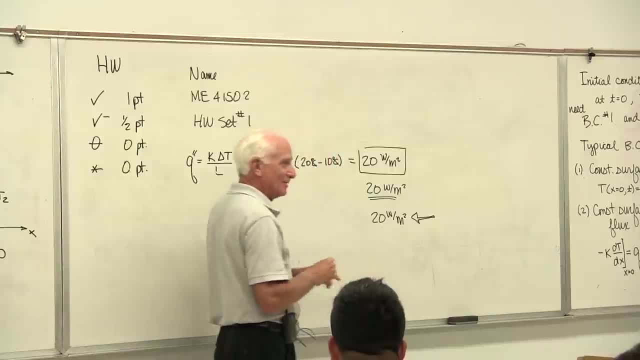 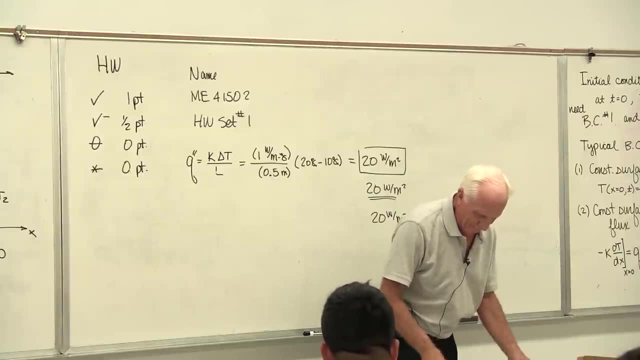 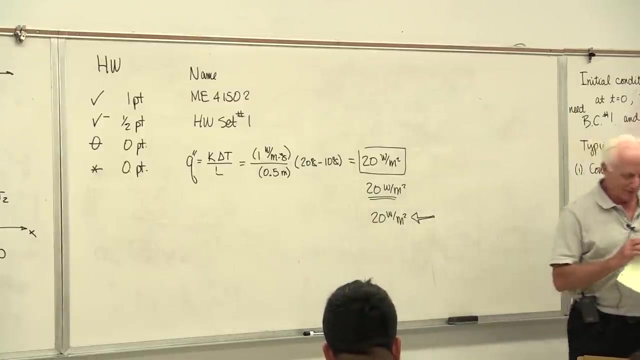 They'll put a big red arrow or something by it. I don't care, But just somehow make the final answer stand out and that helps. And the last thing I think I comment on your papers- was it really? but by the way, engineering degree is fine. 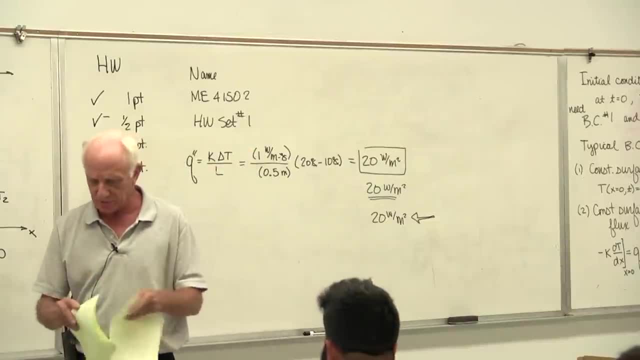 Do it one side only. It's easy when I'm gray not to worry about what's on the side Two makes my life easier. one side only White line paper is fine. I'm not going to tear this up, I'll just show them. 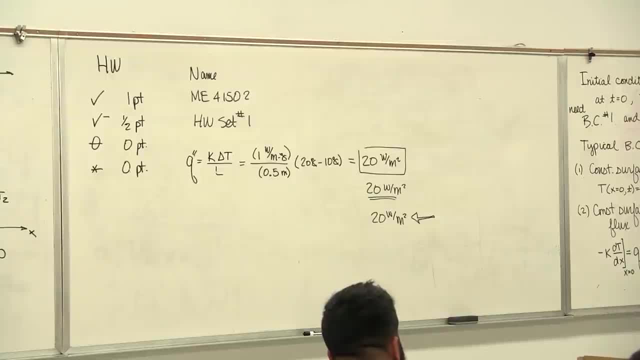 What you don't want to do is tear out spiral bound paper and it looks like Velcro, you know, sticking together. So don't do that. But paper like there white line is fine Staple, of course. of course you know we're engineers. 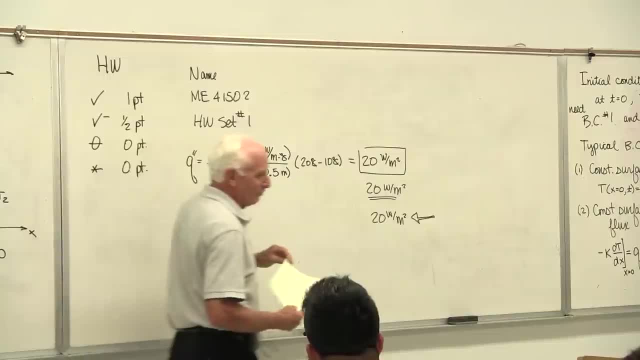 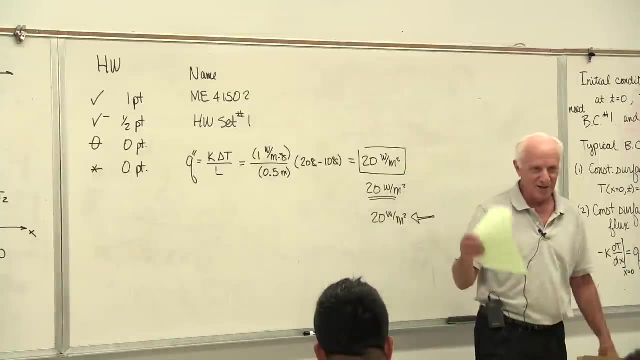 We're not art majors staple. yeah, We tell our freshman. I've told my freshman class: listen, you guys, engineers, 90% of our engineering seniors use engineering green. Okay, I tell these freshmen this story And I said now, when you do your homework, this is what you don't want to do. 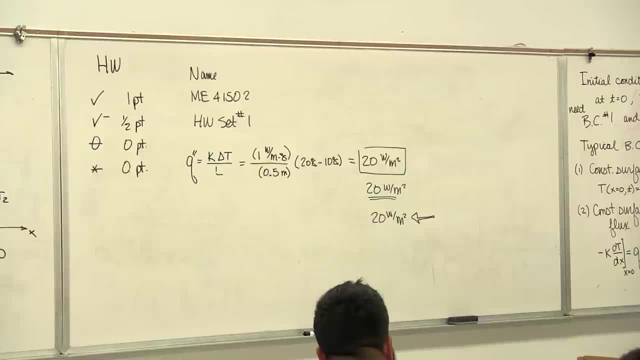 You might have been taught in high school, but change it. You take your, I'm going to turn my homework, and so I'll fold it. I'll fold it, I'll fold it, and then I'm going to tear it here, and I'm going to tear it here. 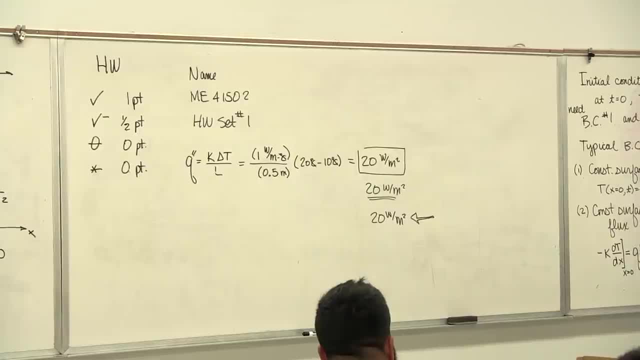 and I'm going to fold this little tab down. Am I creative? Fold the little tab down and I don't have to buy a stapler. Oh, I know, stapler might cost $2.95 for a little cub stapler that big. 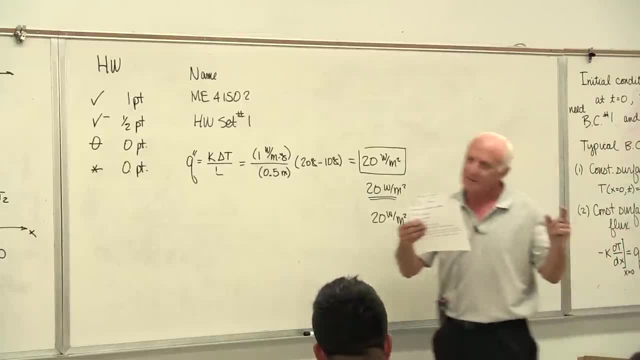 but I'm going to save $2.95.. I'm going to save $2.95.. No, no, don't do it. It's not worth it for four or five, six years of your education here. Don't do it. 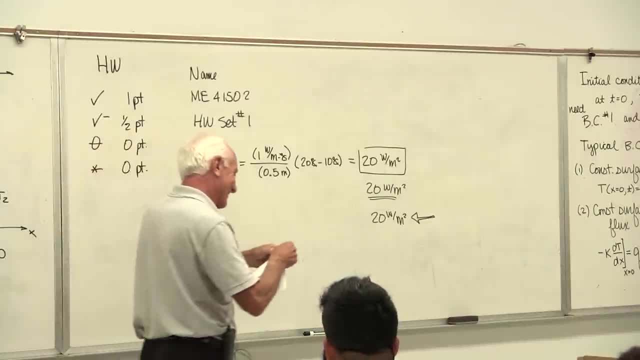 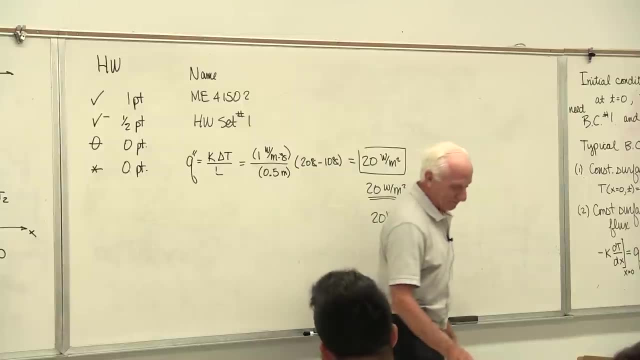 Buy a stapler. So that's what I mean by that. okay, I know you guys don't do that, but freshmen really do, honest to goodness. Okay, the last thing is between if there's multiple problems on one page. 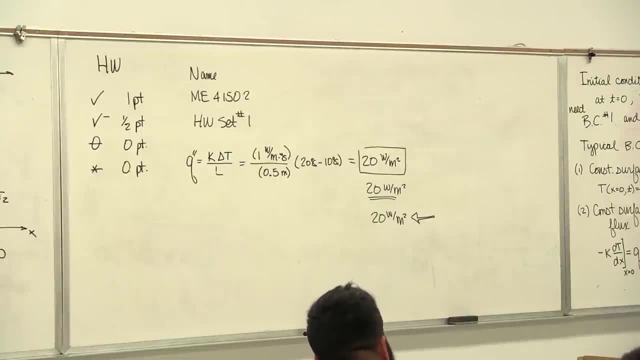 it really helps if you put lines between the problems. okay, It helps me locate the right problem to grade quickly and the reason you know when I'm grading 150 problems, I've got to move fast. I can't dwell too long. 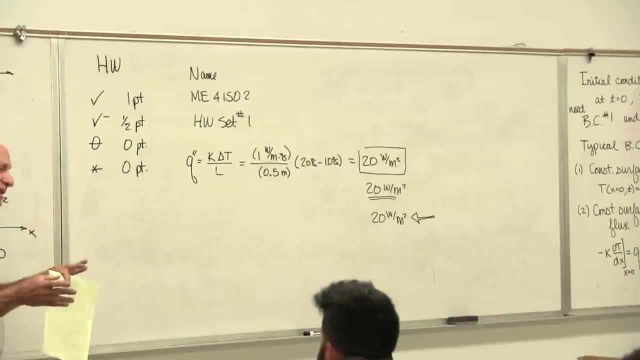 This helps me grade your homework. So, and when you're studying for the final exam, boy, is there big-time payback because you've got everything organized ready to go the week before finals, the 10th week, to look at your homework. 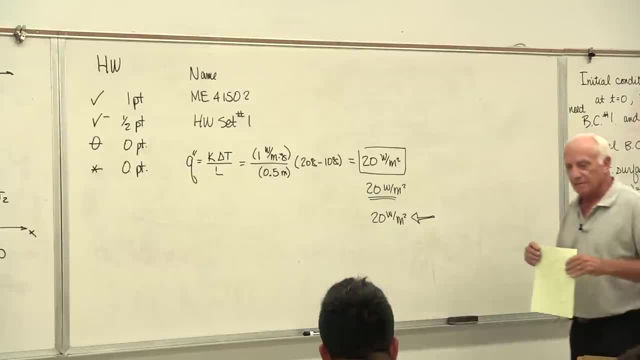 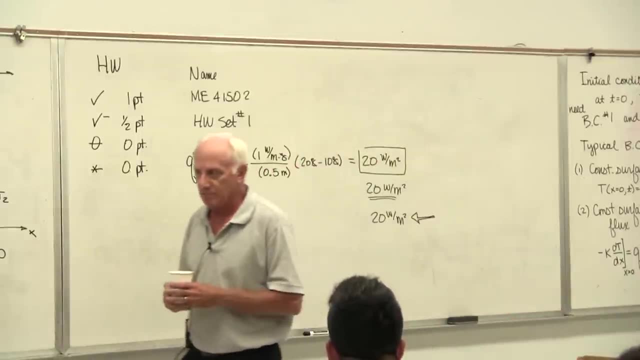 Plus, of course, you know the story: Keep your homework for every class, because when you graduate, you might need it for your job, especially for some companies who require you to be professionally registered: Aerospace companies, any company that builds bridges, or anything that. 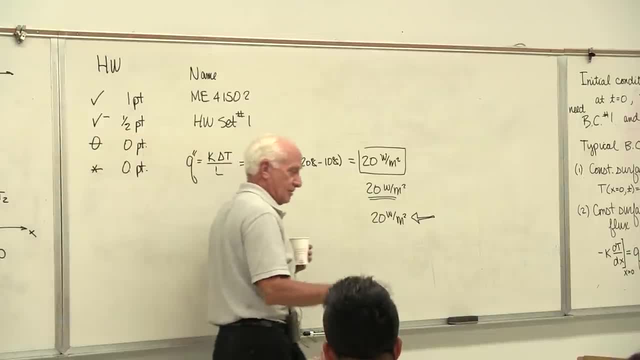 where the public is at risk. oh yeah, they want a registered engineer to sign those documents off, And so if you're going to try and pass the FE exam or the PE exam for mechanical engineering, it's great to have your homework in a little folder to review it. 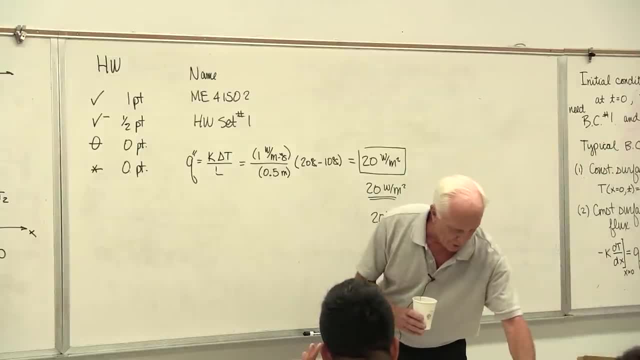 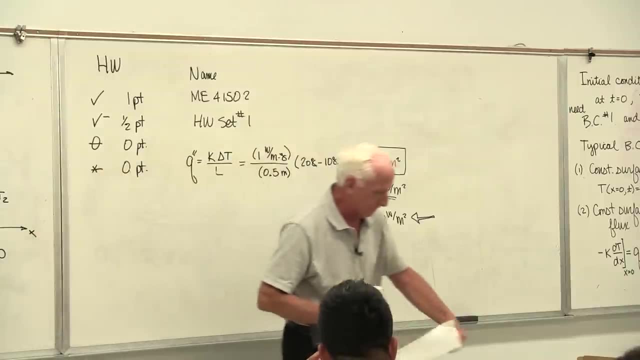 Oh yeah, sure beats going out and trying to buy a textbook that has work problems. So keep all that stuff and it'll really give you some payback if you do have to get registered professionally. Okay, now let's go back to homework and look at one more. 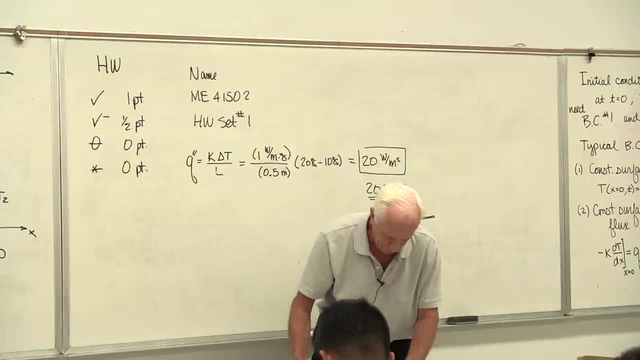 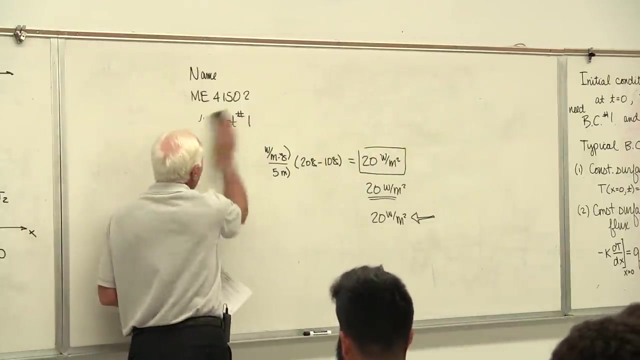 Let's take problem 31.. You have problem 30 for homework, so I'm going to do 31.. I think I'll start in the middle. I think will be okay. Was there any question on the homework format and the grading? 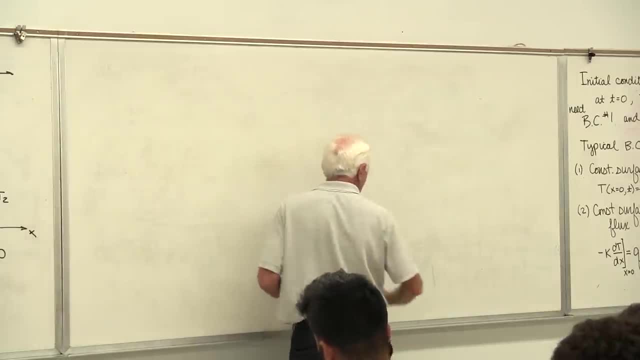 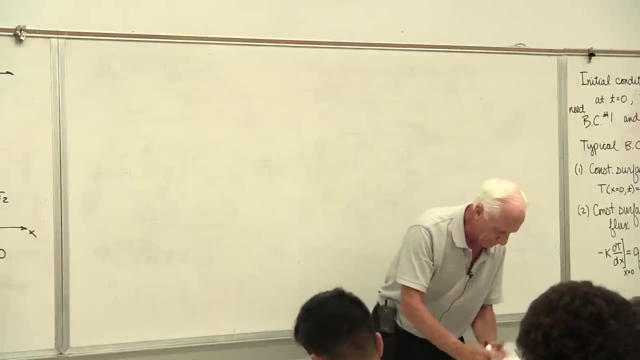 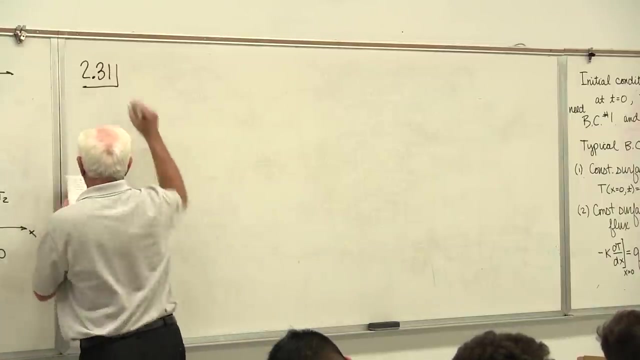 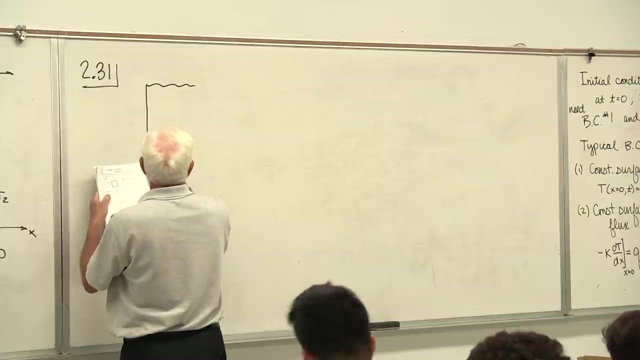 No, So on and so forth. Okay, All right, now let's see here. There's no picture in the book, so it's just words, and I'll read it. Okay, so this is 231.. We have a wall, and the wall is three-tenths meters in thickness. 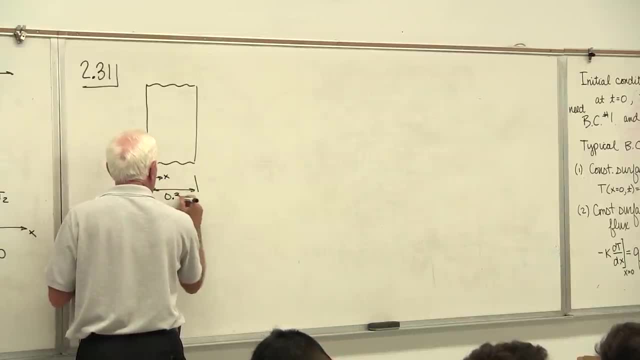 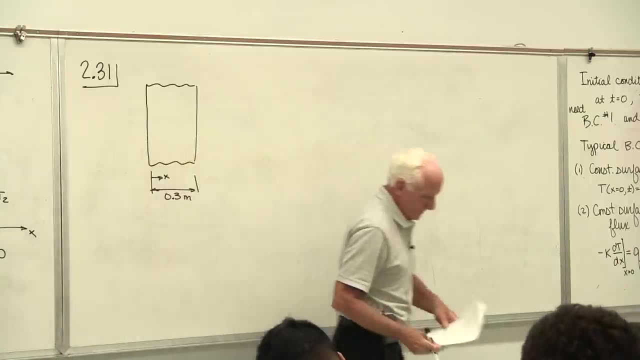 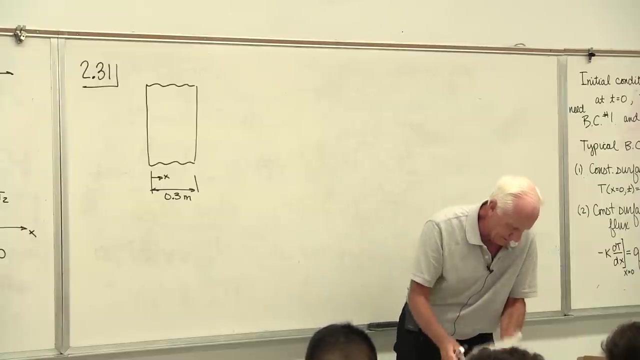 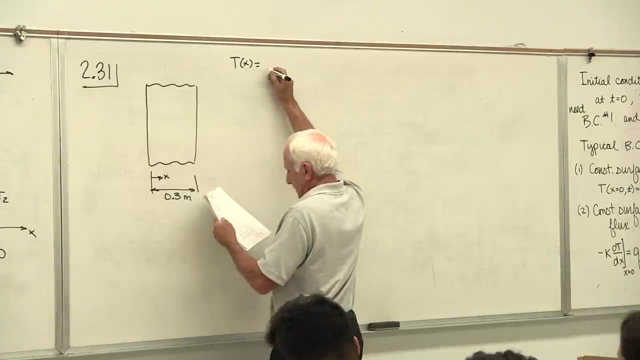 Now that's L. Let me read it so I can: The temperature distribution across a wall at a certain instant of time. he tells us this. He tells us the temperature across the wall as a function of x is 200 minus 200x. 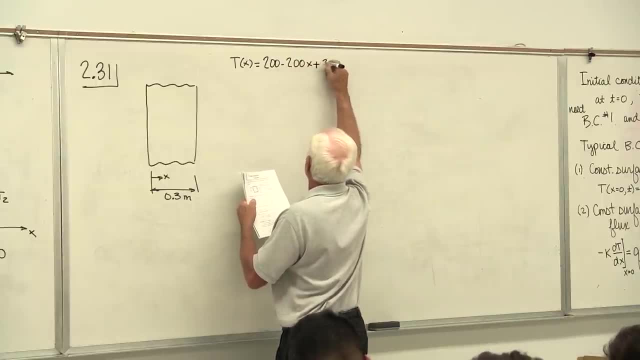 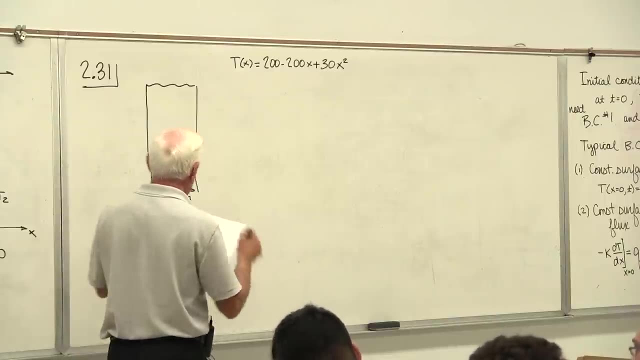 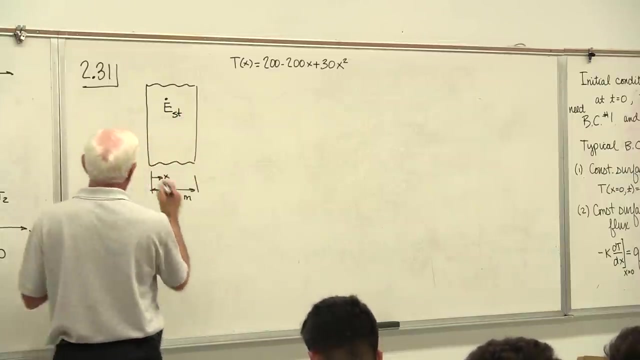 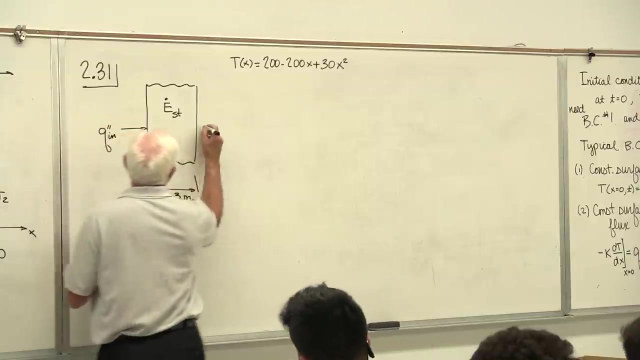 Let's see Plus 30x squared. Okay Okay, we've got storage in there, so this is a time-varying problem. We've got conduction coming in. Okay, Okay, Okay, Okay, Okay Okay. 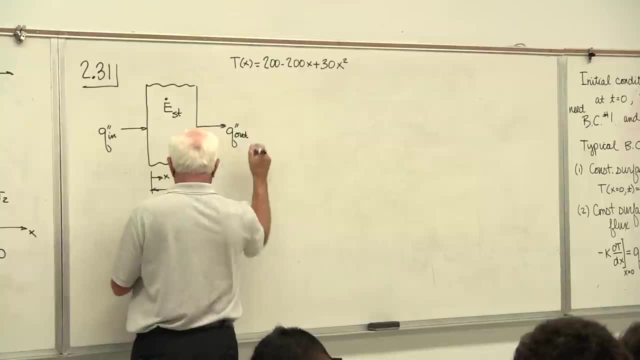 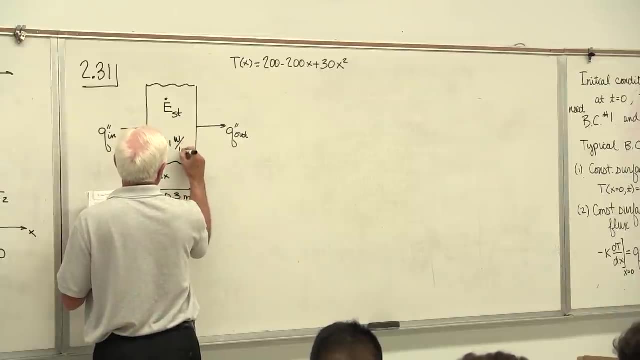 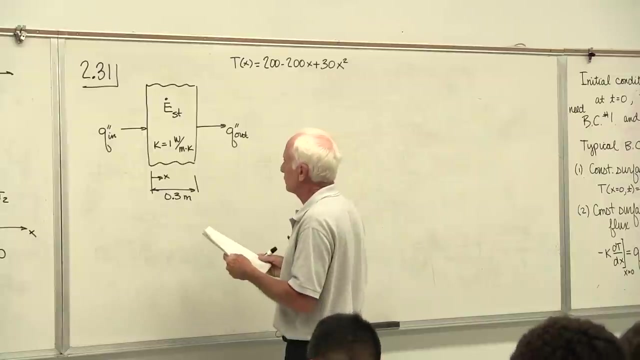 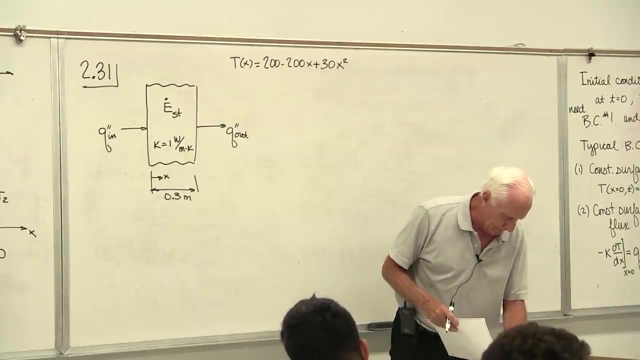 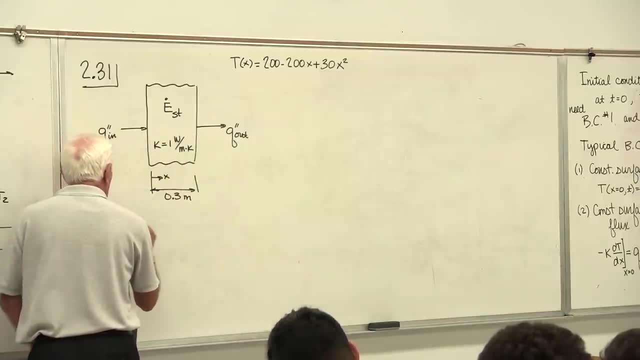 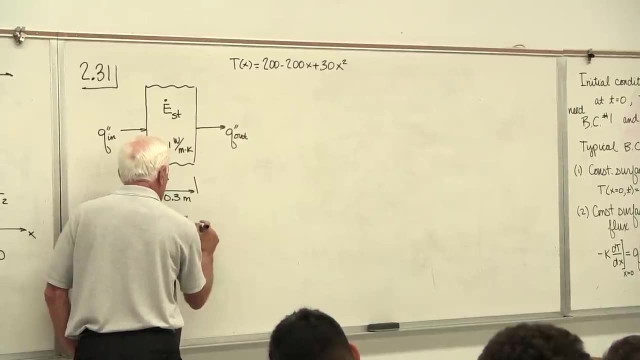 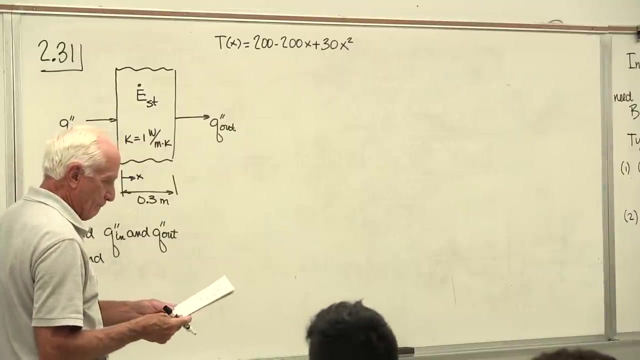 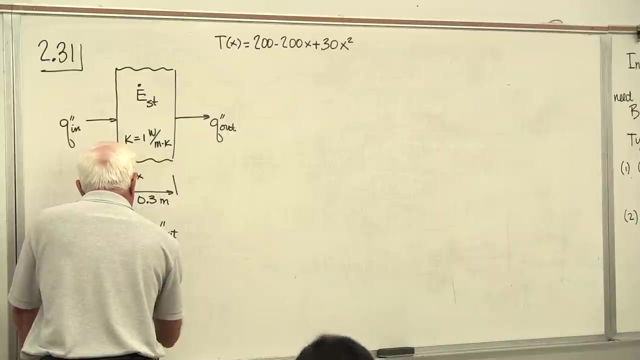 So part A, Find Q double prime in And And Q double prime out And then find the rate of change of energy storage. So E dot storage per unit wall area. Okay, Okay, Okay, Okay, Okay, Okay, Okay. 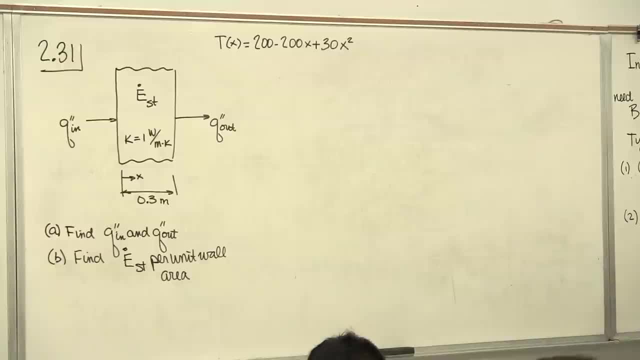 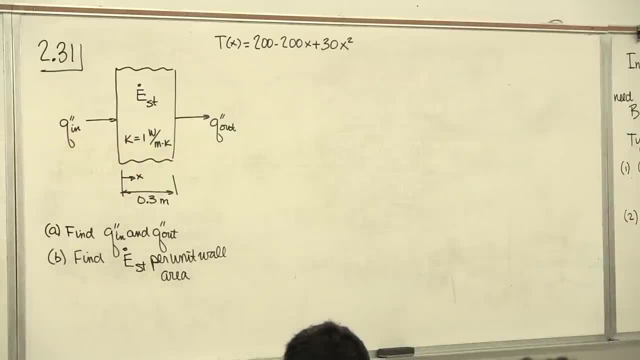 Alright, Okay, Alright, Alright, Okay, Very good. Okay, Very well, I've got my line down here. be body: Okay, Everything is placed right over the board. Here we have Qn minus k. I'm going to do double prime k: dt dx at x equals 0.. 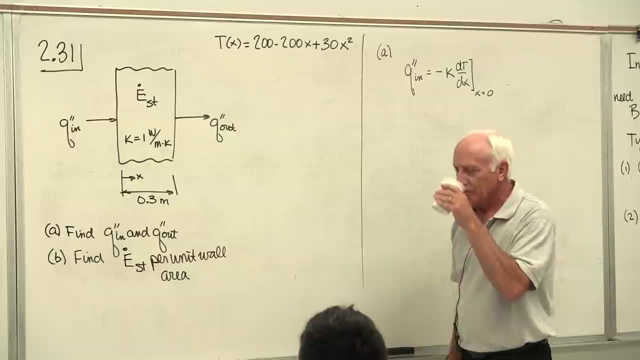 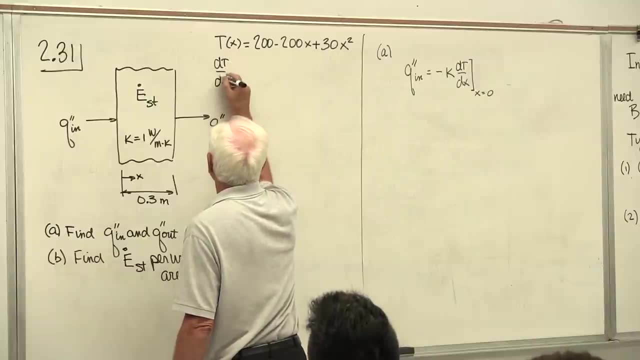 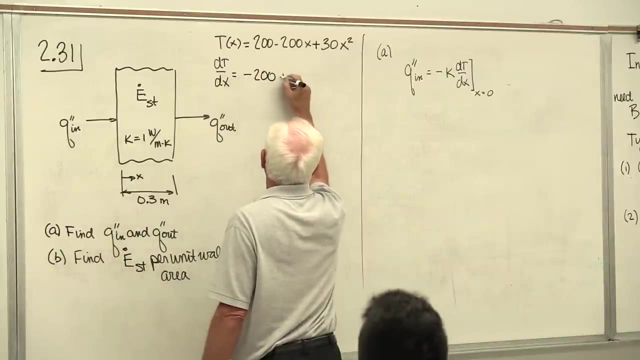 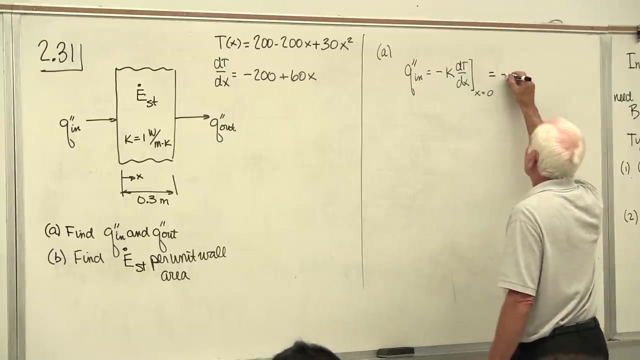 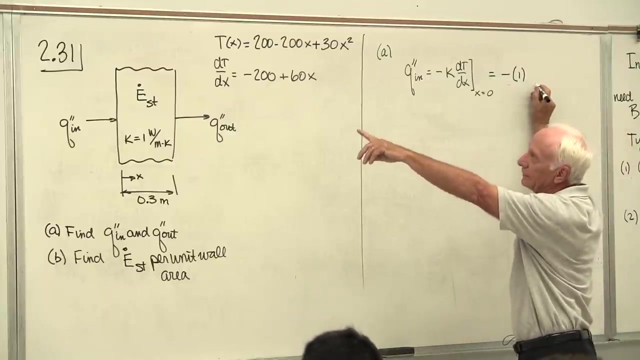 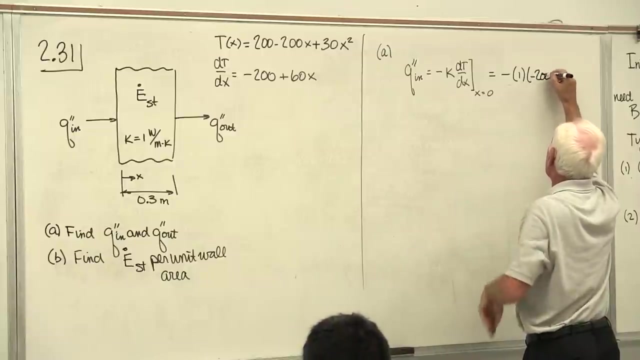 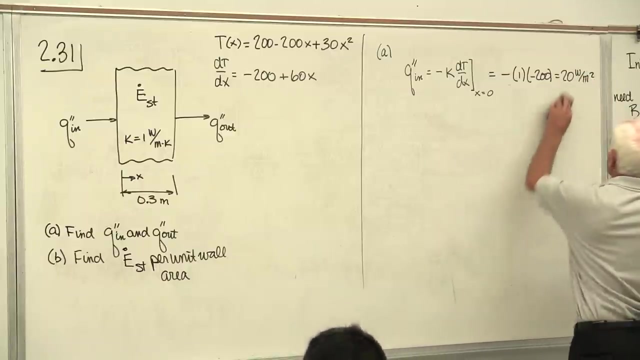 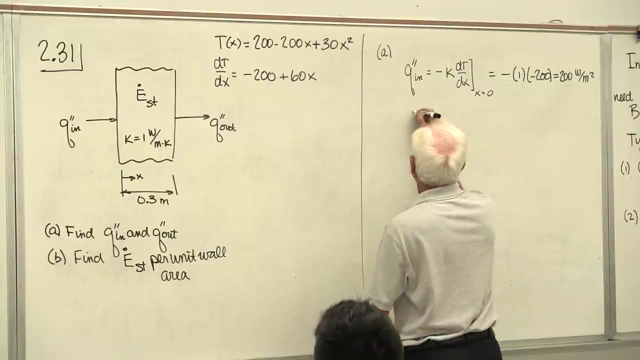 Okay, Okay, dt dx goes out minus 200 plus 60x. okay, Okay, k is 1.. Okay, dt dx at x equals 0 minus 200, 200 watts per square meter: 200.. Okay, Okay, q double prime. 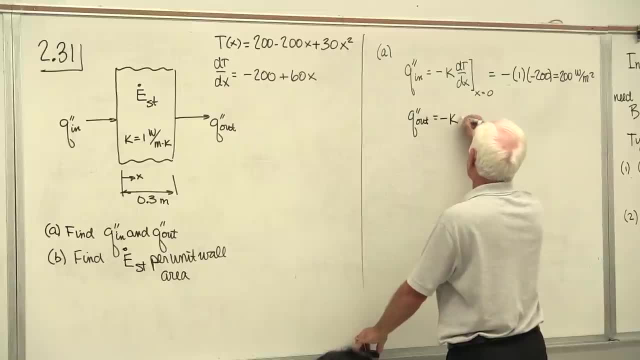 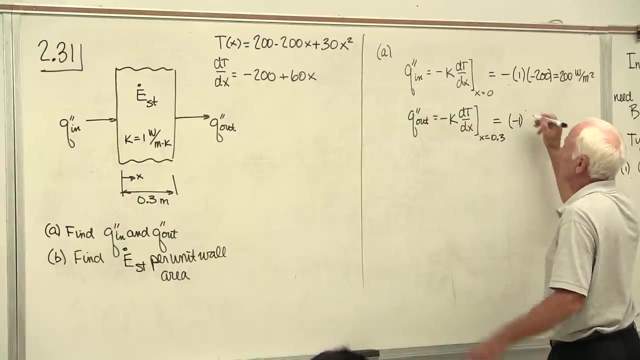 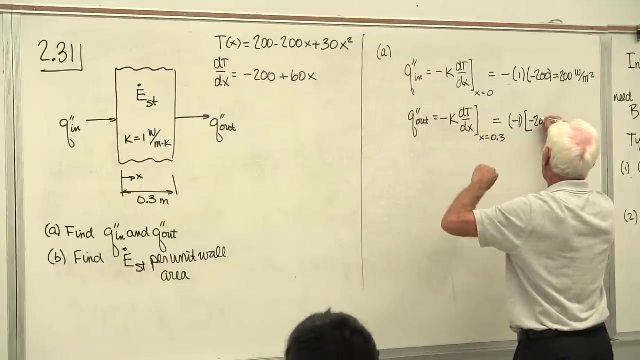 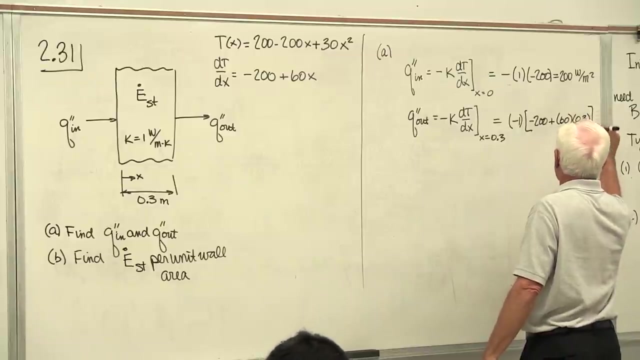 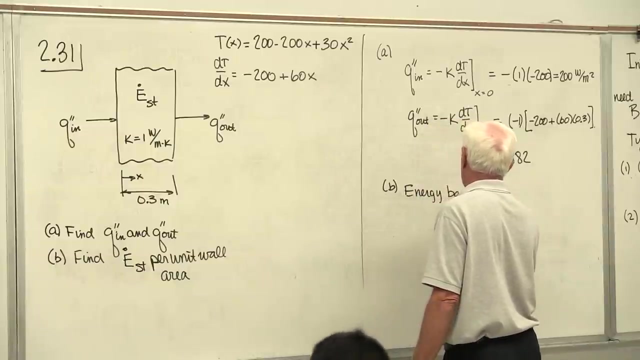 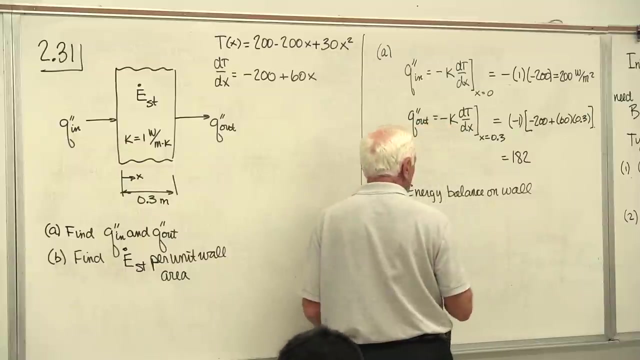 Q. double prime out: All right: k minus 1, dt dx at x equals 0.3, 0.3. Okay, k is 1.. That is 182.. Part b: energy balance On the wall. What comes in the left hand side minus what goes out the right hand side is the stordyapan makes a Hearst equation with k. 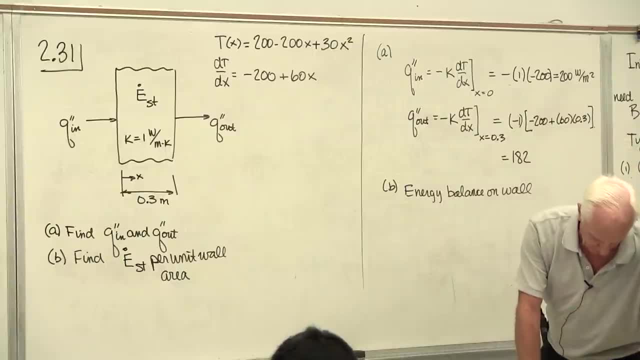 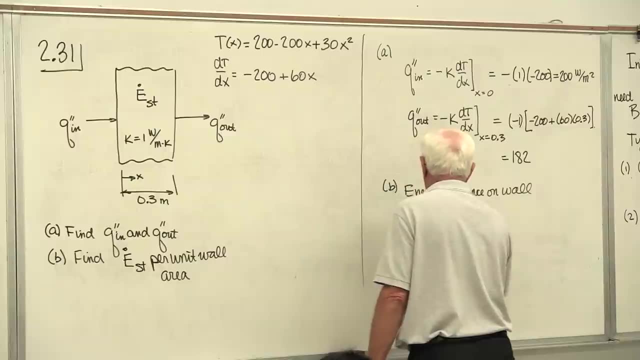 Okay, Okay, Okay, That is a b, So I'll explain how I go through here. Yeah, Yeah, Again, You got all right. that was a quick explanation. All right, storage. So we have Ein double prime minus Eout. double prime equal Estorage double. 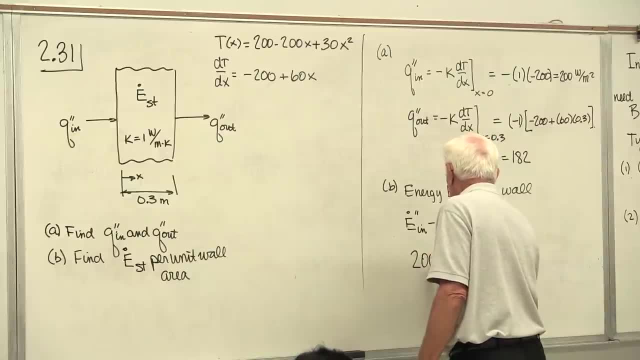 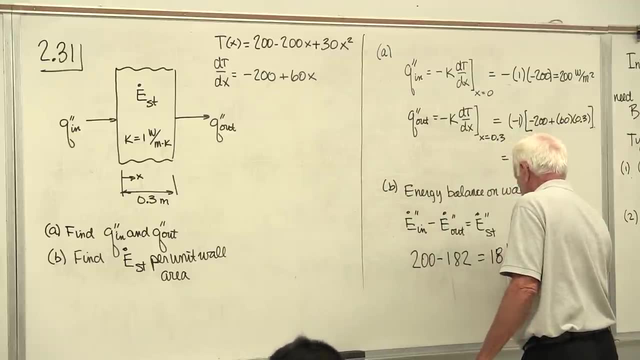 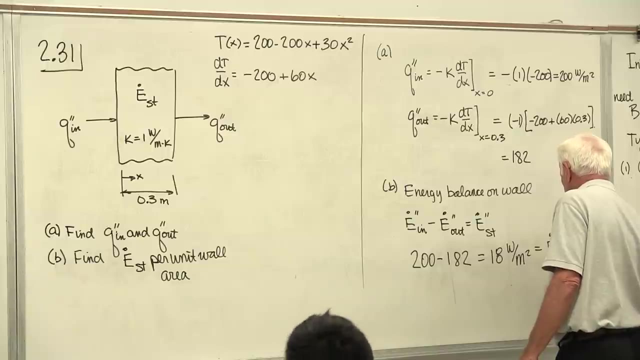 prime 200 minus 182. equal 18 watts per square meter. equal Edouble prime storage. So there are the three ways to do this. These are the three answers of what we are asked to find. Did we use anything from chapter 2 to solve that? No, Where did it come from? It's all chapter 1 stuff. Then why is it in? 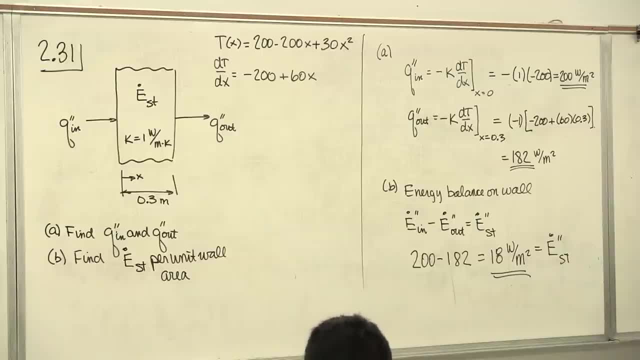 chapter 2?? Well, you can solve it another way. if you want to, Let's solve it the other way. Go to the heat equation. heat diffusion equation: Alright, one dimensional constant properties, no generation. This is what you get, okay. 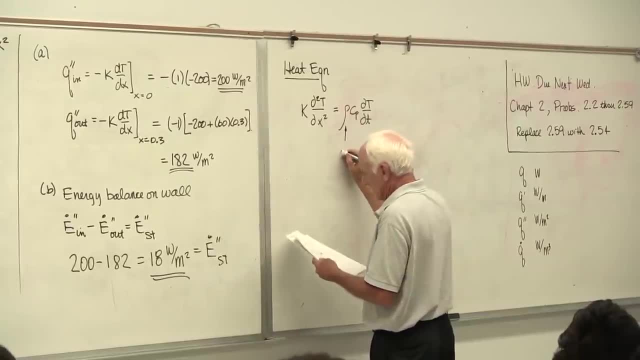 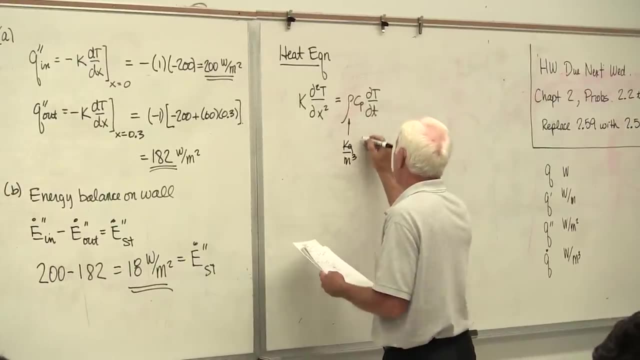 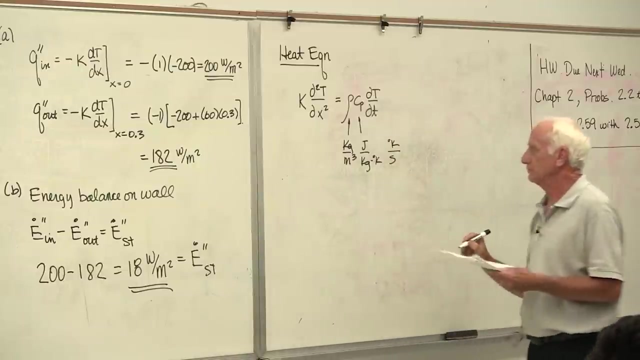 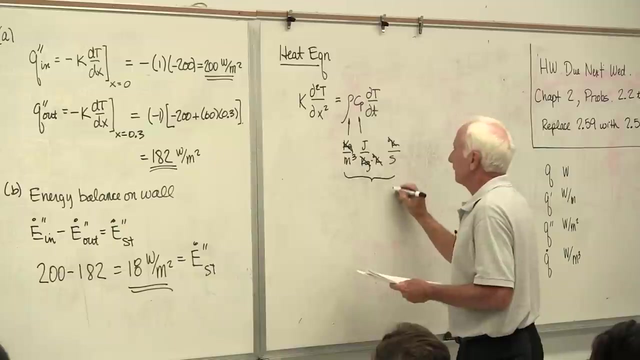 Rho is in our kilograms per cubic meters. Cp is our joules per kilogram k. temperature, Temperature in degrees k. time in seconds: Cancel, cancel, cancel, cancel. This is joule per second. watt. watts per cubic meter. 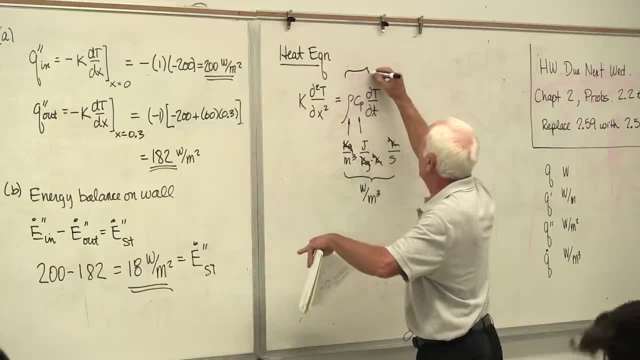 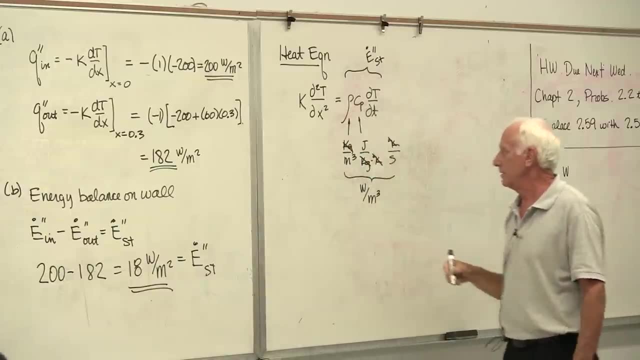 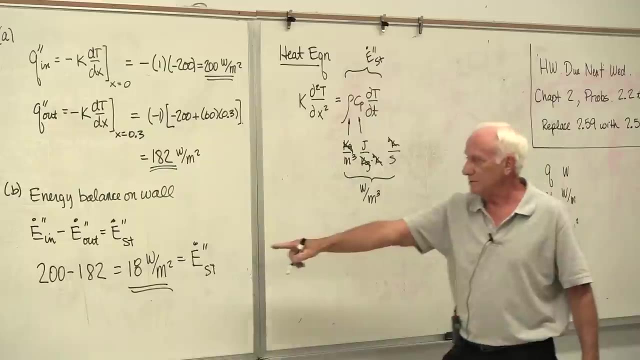 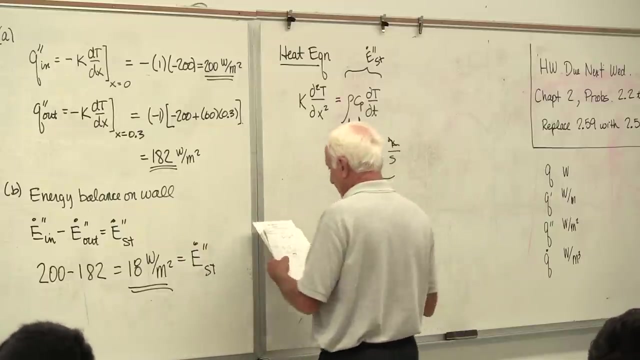 This is E dot double prime storage, because the area is going to fall, We're going to run out of there. But I want the answer in watts per square meter of surface area. So I'm going to multiply both sides by V over A. 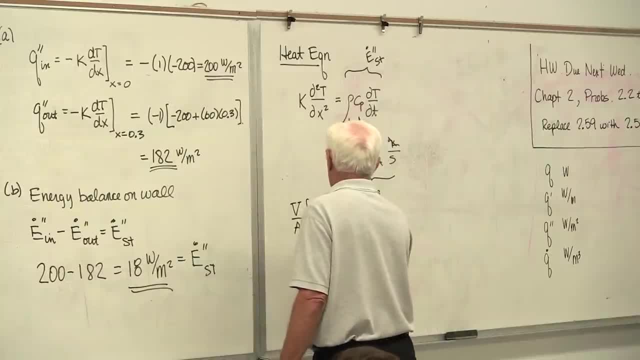 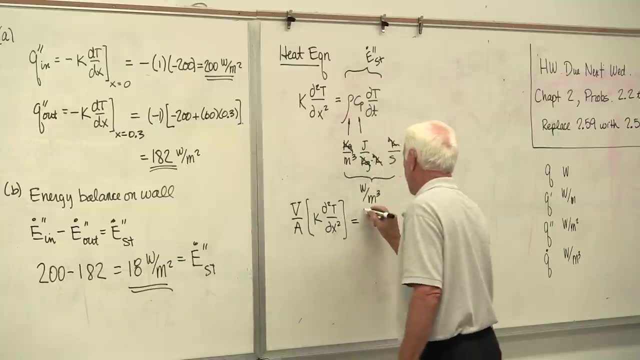 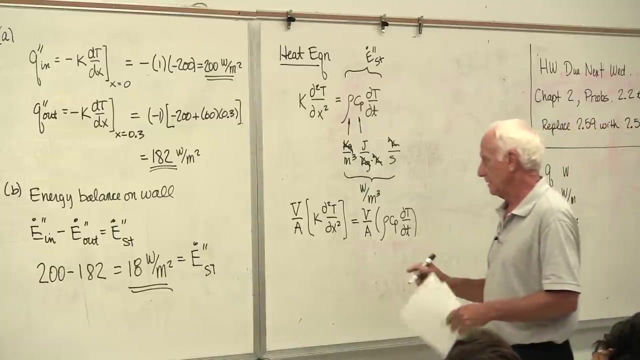 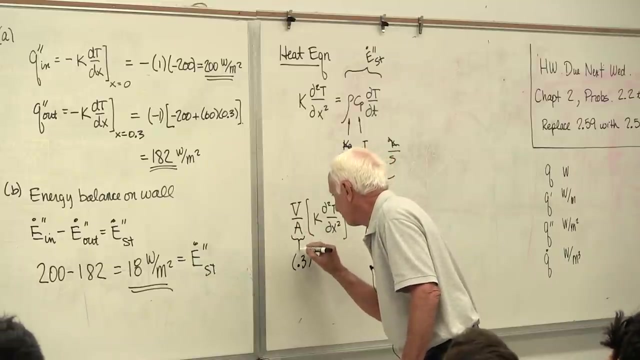 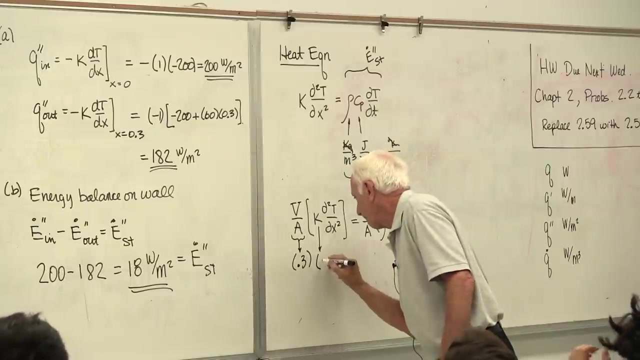 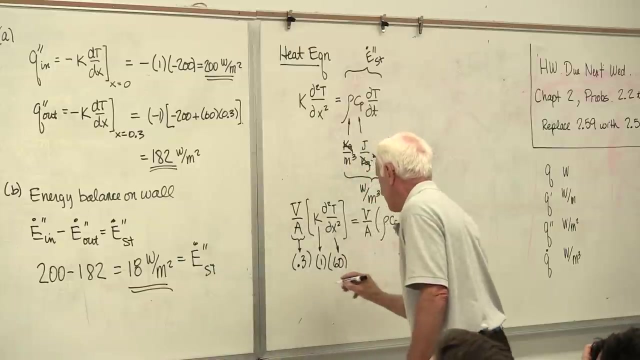 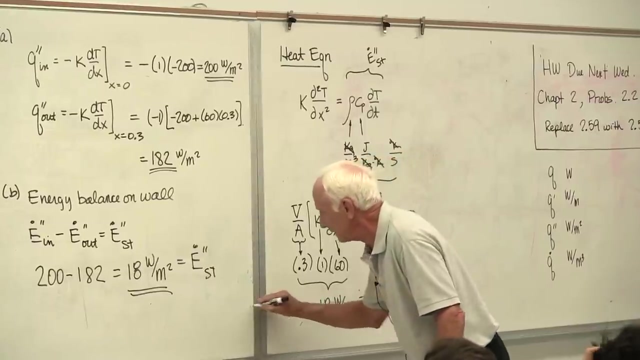 V is the volume. The volume is A times 0.3.. A times 0.3.. So this becomes 0.3.. K. K is 1. Second derivative: First derivative, Second derivative. Okay, You can see what it is.